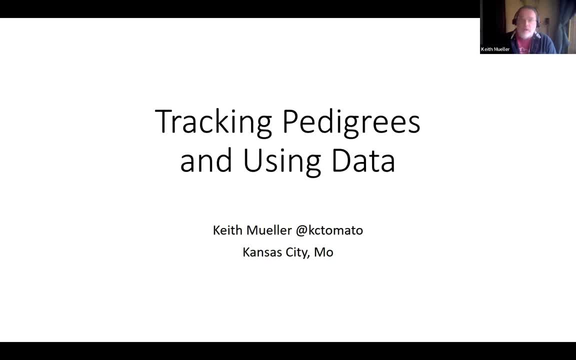 Keith Mueller, R&D. When I first started out I was in the Army started out I was working for a melon and bean breeder and my job was to go out in two acres of melons and write down and take data on every plant in the two acres and I measured size. 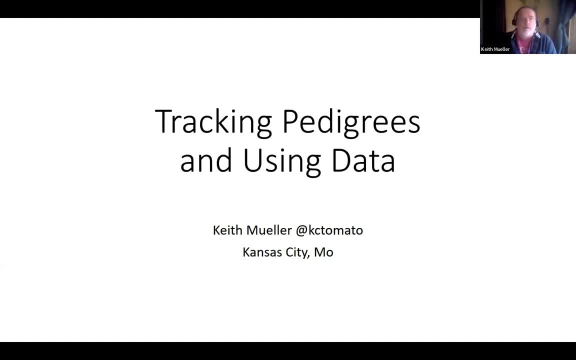 thickness, firmness and you name it- bricks, and it was incredible amount of time and I know all that's valuable, but I'm not really writing papers. I'm trying to develop varieties, and the professor that I worked under at University of North Carolina, Randy Gardner, really influenced a lot. 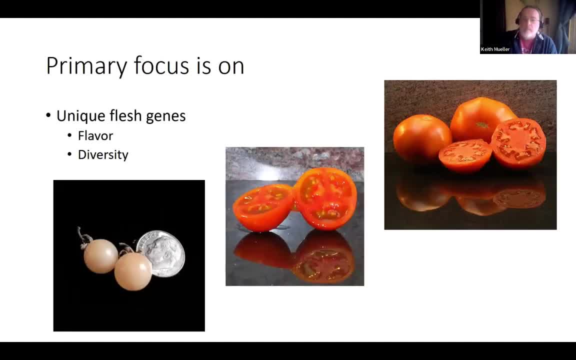 of the way I do things and have changed, and so my primary focus and my project is flavor and diversity, and I work with these unique genes that are found in tomatoes that most people are not using or don't even know about, but they alter the carotenoids and the color in the tomato. they also 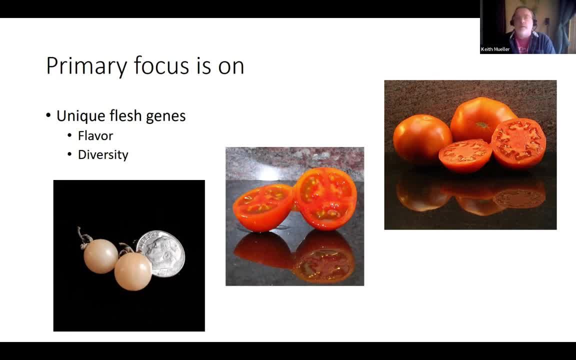 influence the flavor of the tomato. so I work with these unique genes that are found in tomatoes that most people are not using or don't even know about, but they alter the carotenoids and the color influence flavor. Now, some of that you can start picking up on if you go into looking at. 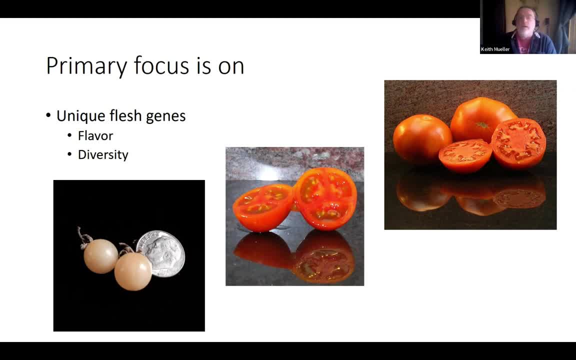 Harry Klee's work and the University of Florida. So in the pathway of developing these carotenoids, these metabolites are created and they create different flavanols, different unique characters to the flavor, beyond things like bricks and stuff like that and that's. 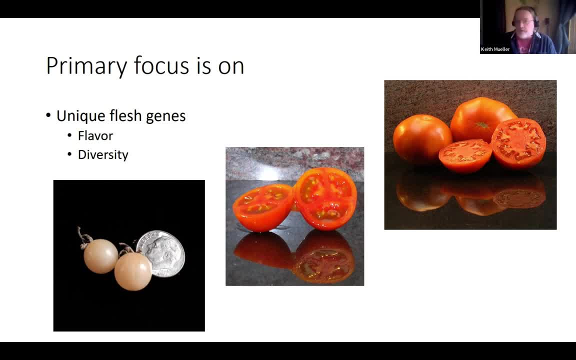 impossible for me to qualify and quantify because I don't have the kind of analysis available to me that they do. but you can, you know, make great observations and pick up on things, provided you take the right kind of data. So the smallest one to the left is the sherry gene. 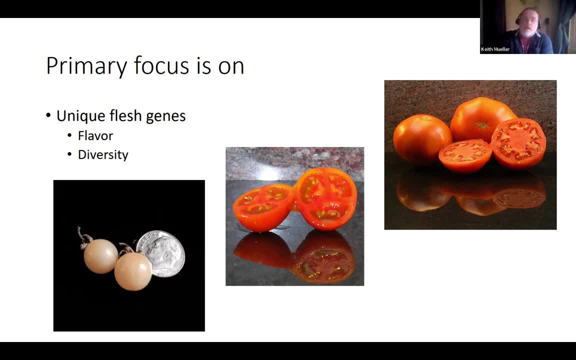 and it was recovered and I'm going to track this one from a very small, almost current-like tomato. but you can see it's kind of ivory and if that one doesn't really show it, but it's got a little bit of a pink tinge to it. 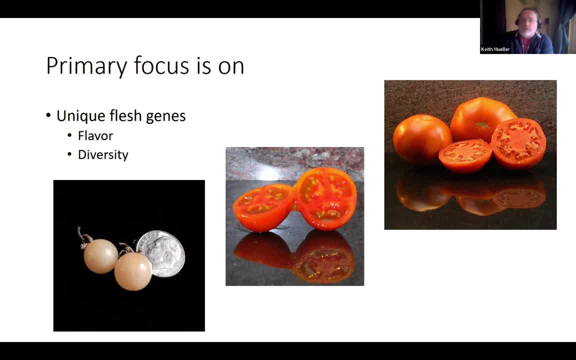 The middle one is called apricot, which was found in a variety in Mexico in the 50s, and the other one up is an advanced form of the delta carotene gene which came from another species, but I've had more luck getting size into that one. but I want to work with these genes to 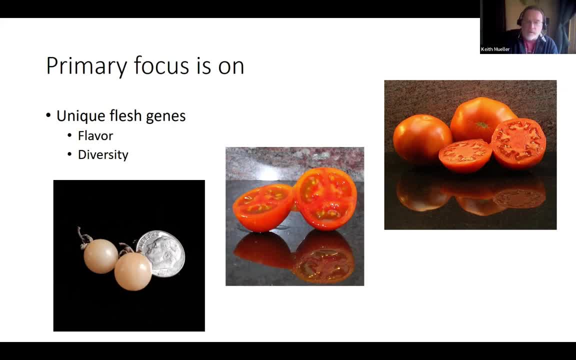 introduce diversity and take them from small things sitting in seed banks into larger fruit that can either be on their own, or somebody younger than me can now take that and run with it and make varieties from it, and that was the idea of doing this is to try to get 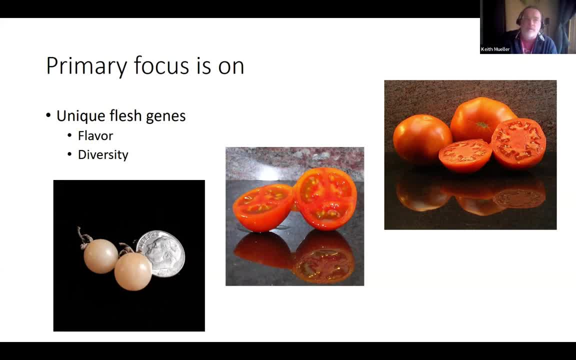 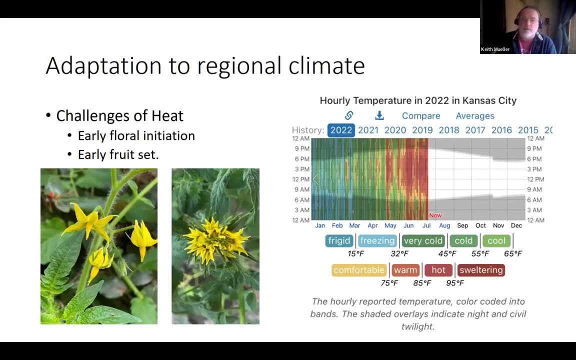 that diversity out there in a usable form, because some of the traits on these are not that great on their own in the plant and they've got a lot of residuals from the wild character. So I also look at adaptation to my environment here in Kansas City and so I should have switched the things. but 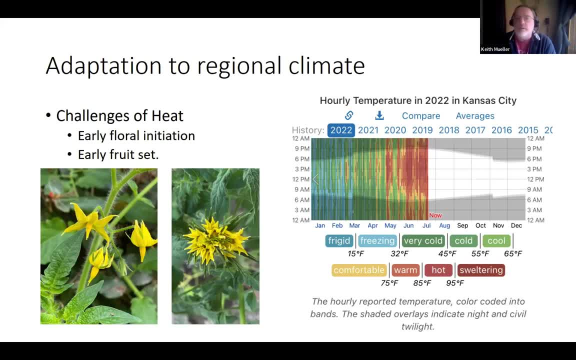 early on when we plant. so we tried to put out things between April 15th- which is kind of pushing it and I'm not talking high tunnels and directly out in the field- to May 15th and then really get everything in by June. The problem is the climate has shifted in the- I've been back 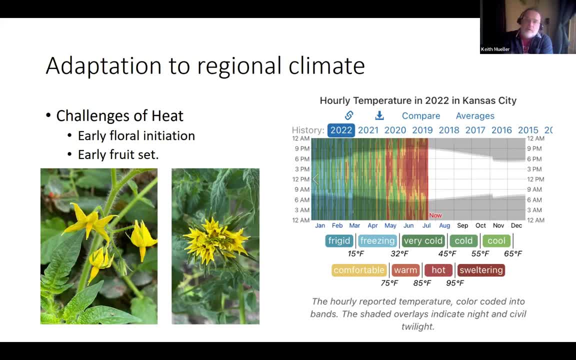 here about 20 years and I've been in the field for about 20 years, and I've been in the field for 20 years and from when I was younger and gardened here. it's shifted and we get this early heat. 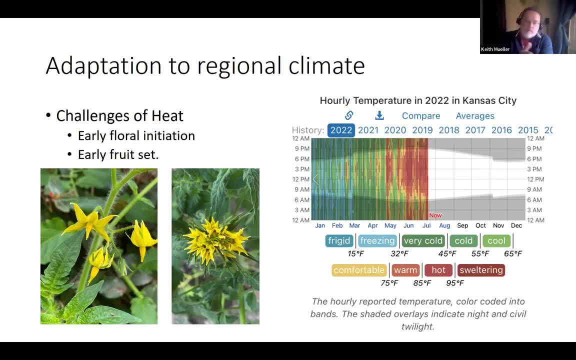 which just it can wipe out flowers, and if you don't get plants in at the right time, it goes from cold to hot real fast. you'll lose your production, and so it's real critical that I find things that not only set flowers but also set fruit, So I spend a lot of time really. 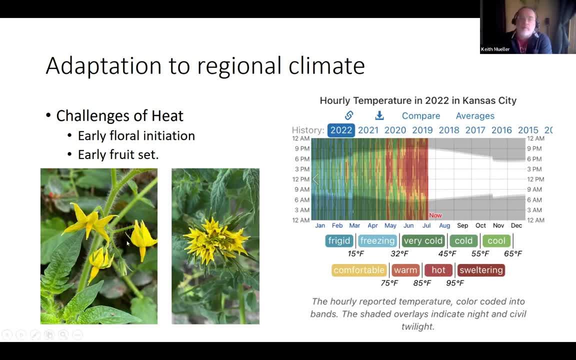 on in the data trying to figure out if I'm getting that initial set. but you know, the heat kicks in in May now and it used to wait until like mid-June and you can kind of see that here. but we get these periods now where it's extremely hot and the flowers just disappear. but you can find. 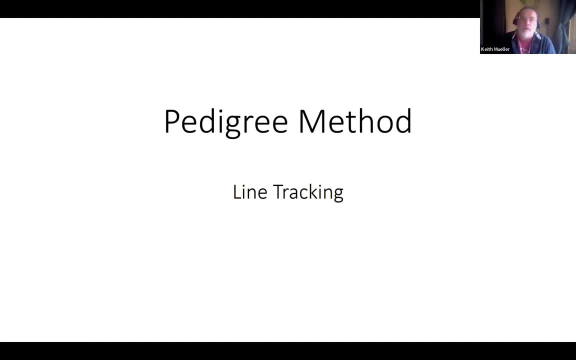 some survival in there, but I use mostly what's called the pedigree method, and I don't know if somebody else is covering this. I didn't have the greatest graphics program here, but it has a lot of different methods and I've been doing a lot of research on that and I've been 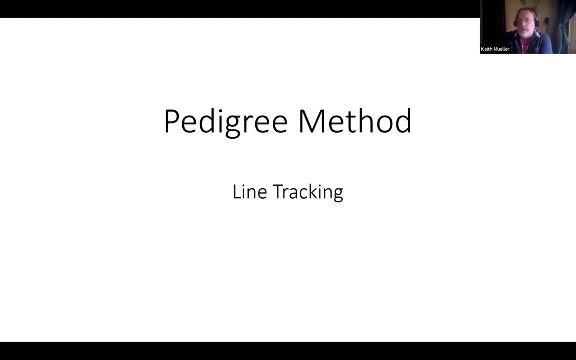 also talking about how I use that to track my lines for my data and development. So what I've got here is: I don't know what's covering your screen or not, but up at the top I've got two parents, so I'm going to look at that sherry line. So I took a large red with. 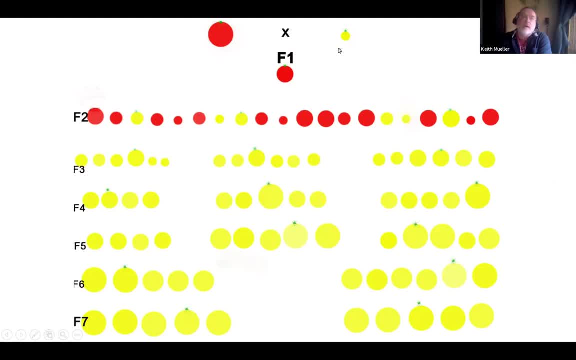 some disease resistance and crossed it to the sherry and what you're looking at is the generations here, year by year, and how I go about it. So I'm going to show you a little bit of how I kind of track it. but you make a hybrid and then you look at the F2, and what I've represented. 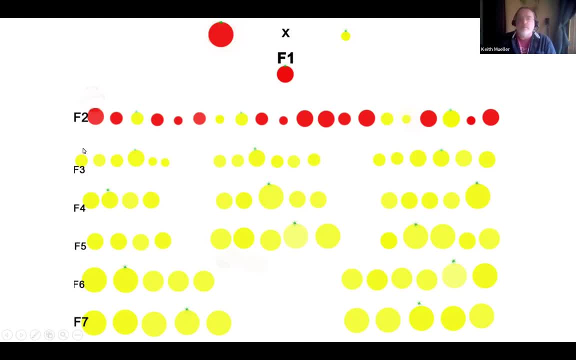 here is there's 20 individuals in this for this example, and then in the F3, you'll see here in a second- I've started tracking three different families based out of that. So this is kind of showing that over here I took plant number three. 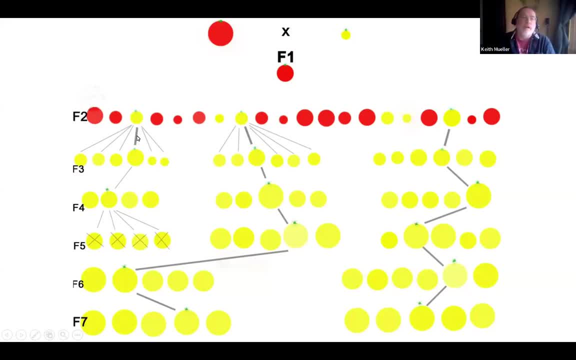 and I grew out- let's say, five, six of them, and one of them was larger. so I used that the next year and that's kind of the path that these dark lines are following. but this is a very basic representation of pedigree method of just tracking a family and just keeping with it and selecting. 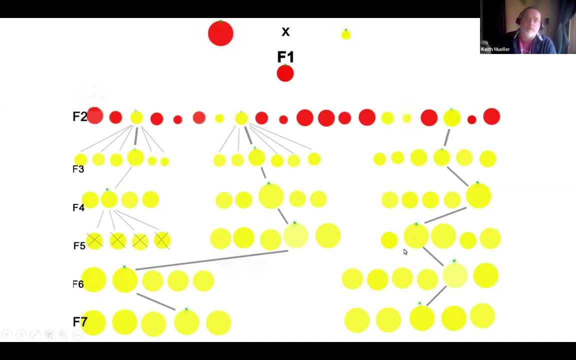 from it and some people call this single seed descent and that's kind of a misnomer sometimes when the soybean project is done and that's kind of a misnomer sometimes when the soybean project we actually did that. but this is more you're saving from that one plant, any fruit and using. 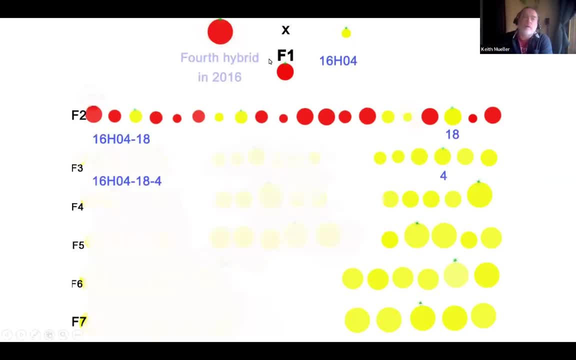 that to go on next year as your selection When I start off in the year 2016,. this is how I label things and track them, rather than names, and it helps with sorting in the data on the Excel spreadsheets and writing things down in the field, rather than if I named it and kept that name. 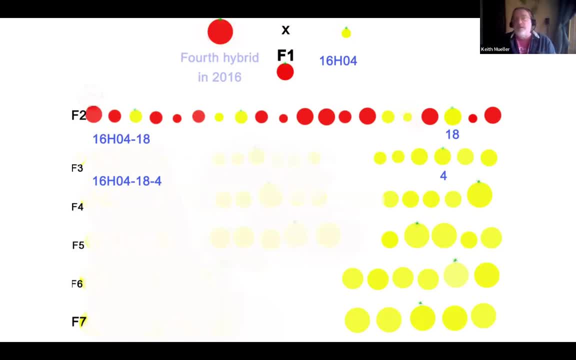 it's more writing, more it sounds funny, but it's more space on the tags and more things you have to do. but, for example, this was the fourth hybrid in 2016,, so I named it 16-H04, so I grew that out. 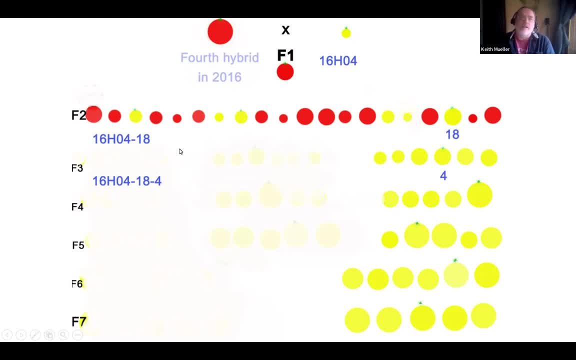 and I've here selected plant 18, so that is represented as 16-H04-18,. so I grow that one out, and next year I select that one out, and next year I select that one out and next year. 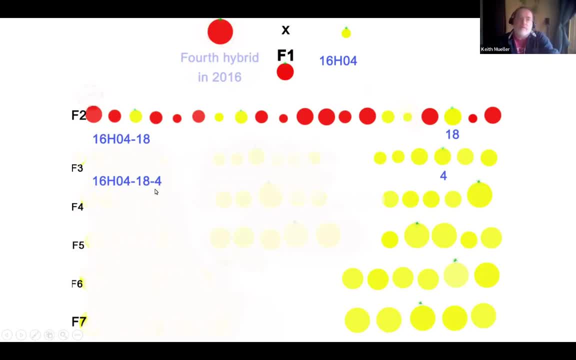 and it's 16-H04-18-4,. so what this allows me to do is track over time where something originated and what path it's going. so if I lose seed or have a problem with a generation, I can go back and go back to that family and look at it and keep it going. but that's basically how I set up. 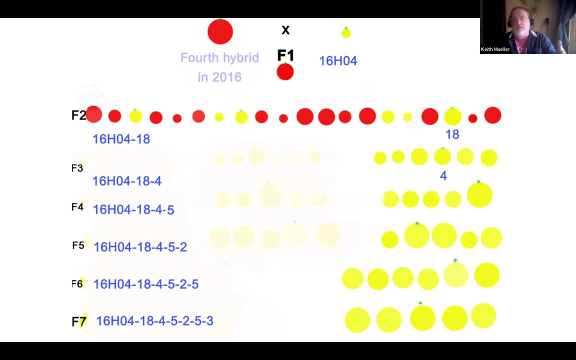 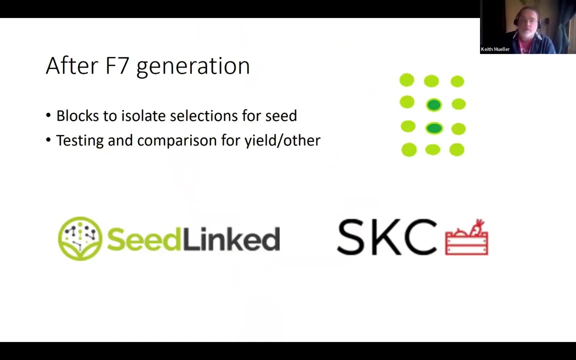 my tracking for a line, since I'm doing all pest control. This is overly simplified, but I was just trying to give you an idea of how I go about using those numbers to do it. After the F7 generation. I will switch things and I will go. 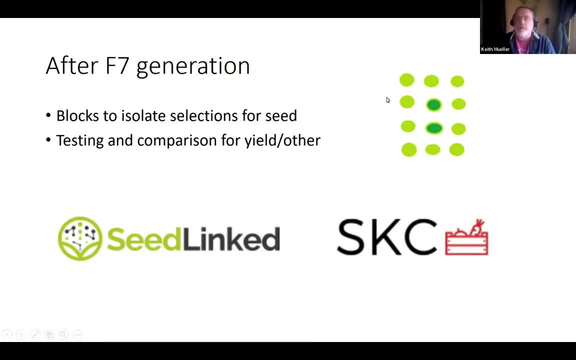 into blocks and that's represented up here. so I'll plant a block and I'll only pull seed from what's in the center. I'd do something larger than this, but that's also when I start looking change the way I look at data. 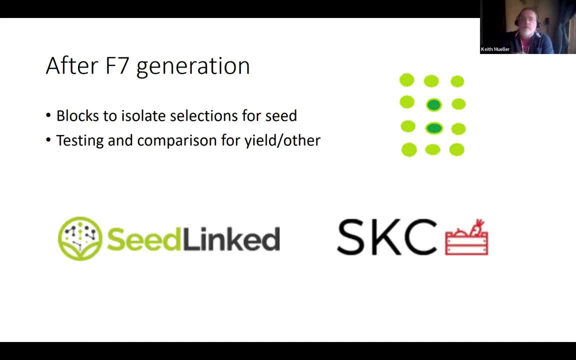 And go into testing for yield and comparing it to other varieties, but I use this block method to ensure that my seed stays pure and kind of do it. It's difficult for me- I work cooperatively with other farmers- for them to understand what I'm doing with this, because I prefer these blocks. 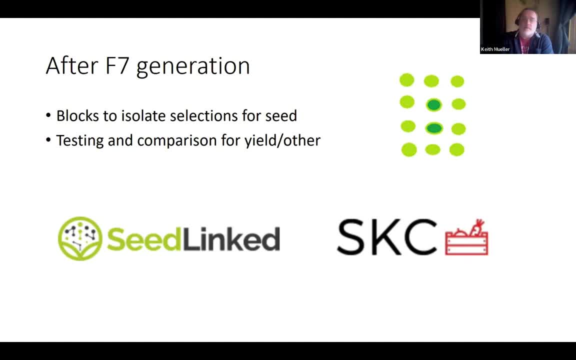 to be 100 feet away from any other tomatoes, so I isolate them and there's no crossing. but I'm going to try to do that. I'm going to try to do that. I'm going to try to do that. That gets a little bit testy. so it's kind of nice to work with other groups like Seed to Kitchen. 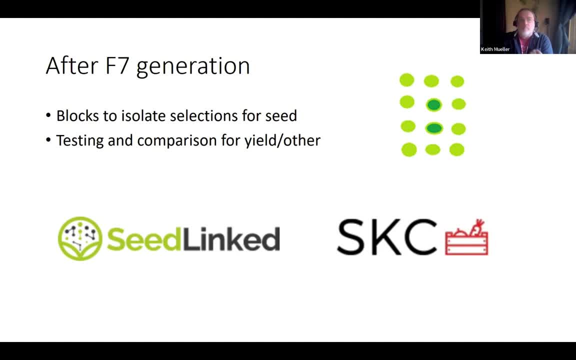 and have some people that are now willing to help me do some of this and also talk to the seed companies about. well, you know I don't have the resources necessarily to do this and you know it's part of the process of me communicating with them about line development and releases. 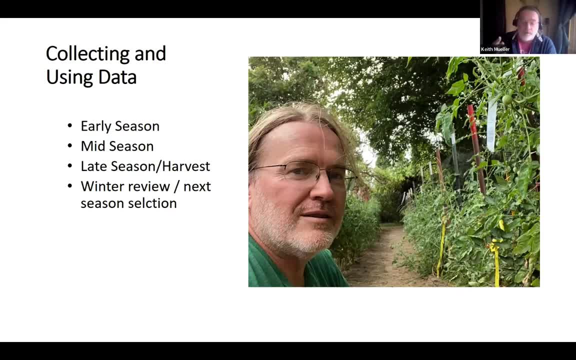 And I also. in that pedigree method I showed you a recessive gene which is pretty easy to track, and the benefit to the pedigree method is that you're going to fix the genes that you want pretty early. It doesn't take as much space and it's more cost effective as far as maintaining it. 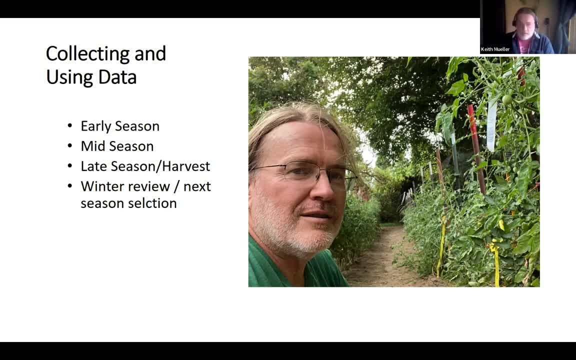 and not having to put as many plants out in the field. Theoretically, then, let's say a bulk method, which I'm not really going to go into. but the benefit to a bulk method would work better for adaptation, because you would just randomly. 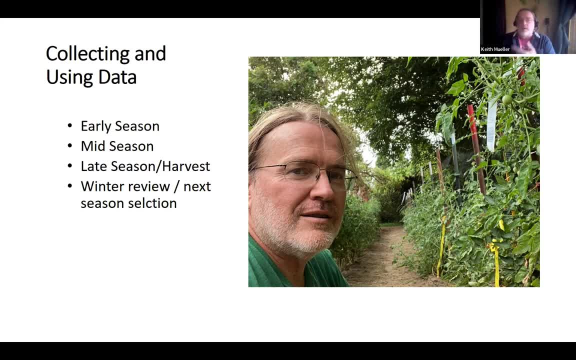 select from that original F2 population and just keep things going for a while. and then, as you get into your later generations, then you start selecting for the trait that you want and the benefit to that is, within that population there's more adaptation. 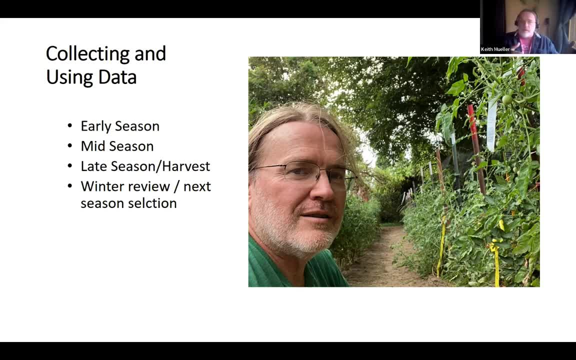 and there's a higher amount of genetic diversity where you've kind of bottlenecked it with the pedigree method. So when I'm collecting and using data I break it up into different parts of the season. It has to do with how much time I have. because I'm independent, I can find people to. 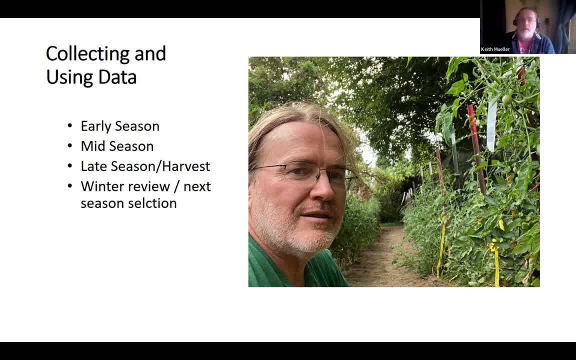 help me do physical work, but usually most of the real, when I need time and help, it's really hot and people don't want to be out there, and I don't want to be in the field early in the morning with the tomatoes because they're wet and I'll spread disease. So I either wait. 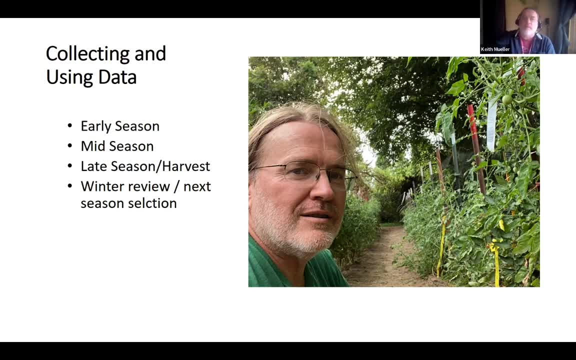 until the afternoon, or in this picture I'm in actually evening and you're looking west and so the light from those trees are blocking in the fields tolerable to be in. I mean, I see some shade there on the row, but you know that affects when I take data and 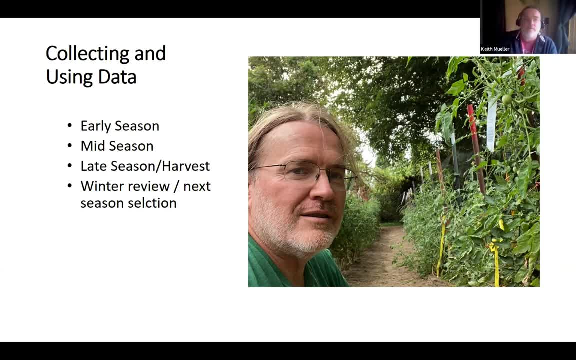 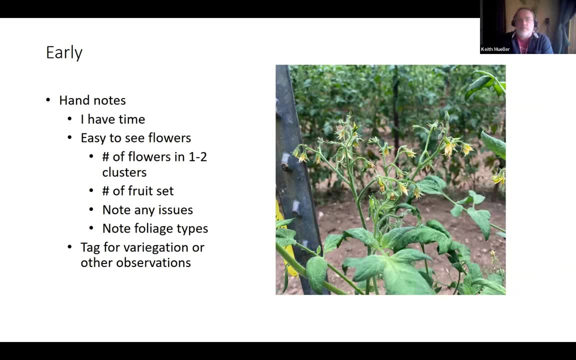 and when people are available, but I don't usually want to work in the evenings, But in the early season- that's when I take all the information on the flowers- I have plenty of time because it's usually I had help putting things in the field and it's just. 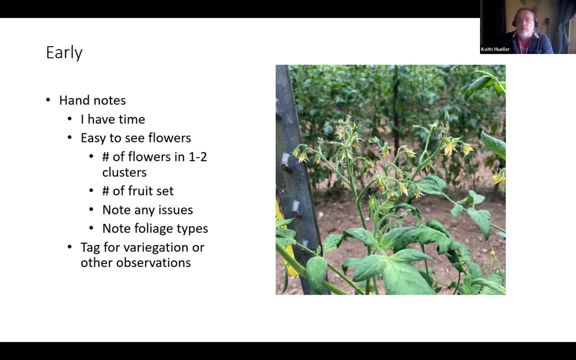 basic maintenance that I'm doing and I could do by myself, which is mostly stringing and pruning and that goes pretty quick. So I have time to go look at the individual plants and see what the flowers look like and what they're doing, And that's kind of an important part of this story. 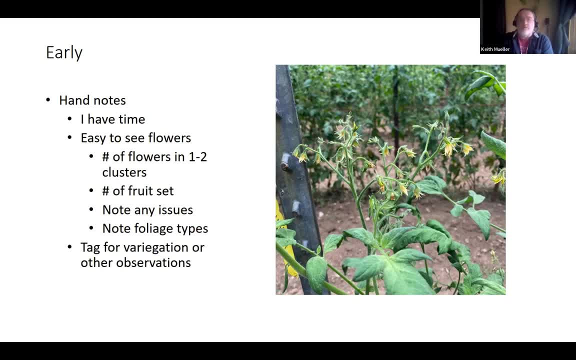 And I have time to go look at the individual plants and see what the flowers look like and are doing in that early critical stage when it gets really hot. so i'll go through and i'll count the number of flowers per plant and per cluster. later on i will count the number of fruit, that's. 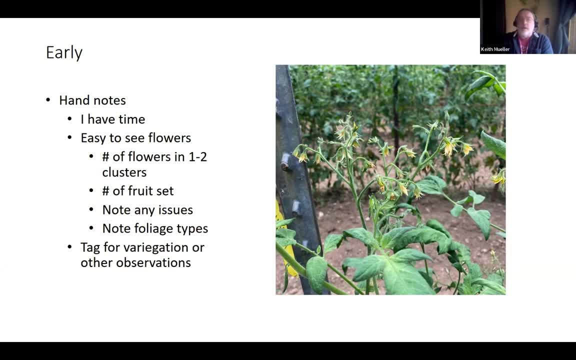 set and i'll note any other issues by hanging a tag. you can kind of see the tag in the background here and i'll write on it what the variety or what line that was and what i saw, and i'll go back and collect those at the end of the year. but it saves me time from sitting down with a notepad and 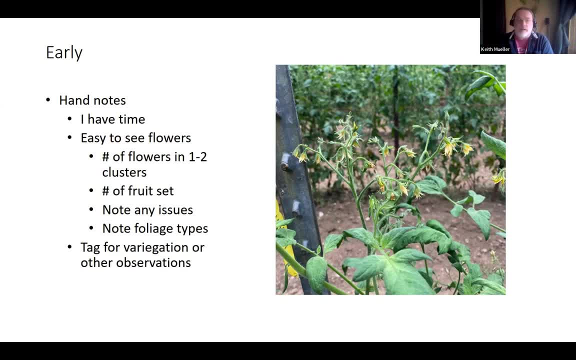 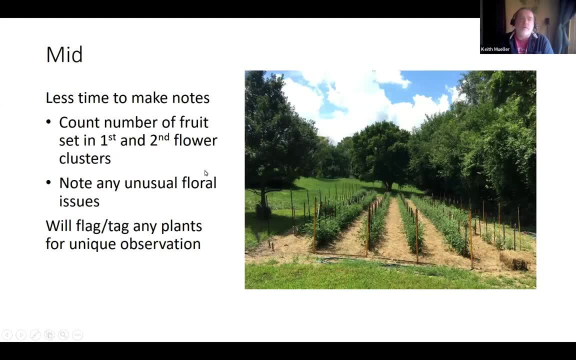 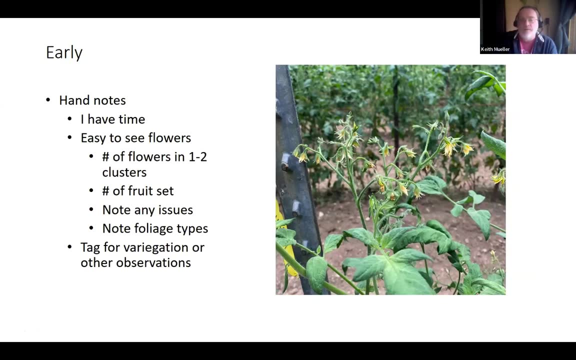 writing notes because it takes quite a bit of time to do that and i can get more things done if i go through and and write just the focus in on the flowers. i will also tag things for, like: if something's variegated, um, and it's, it's a great way, um, working with the plants is a great way to further look at the. 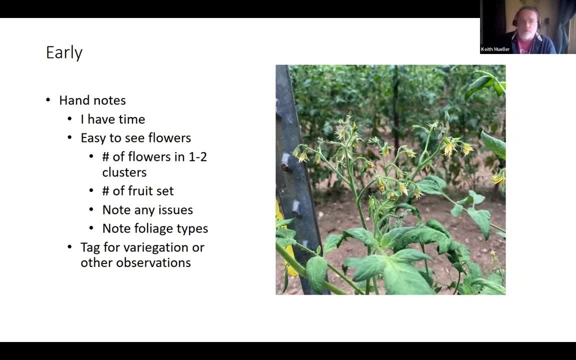 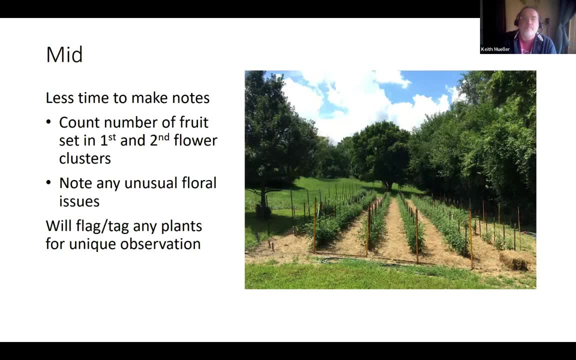 plants more than if somebody else was doing the maintenance and you just came out and went and looked at them. you're you're paying more attention to the individual plants. um, in the mid-season, um, things are starting to come along and um, it's harder to see those uh flowers. but, um, i'll go. 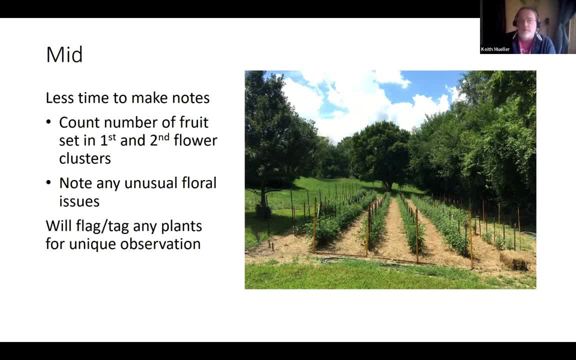 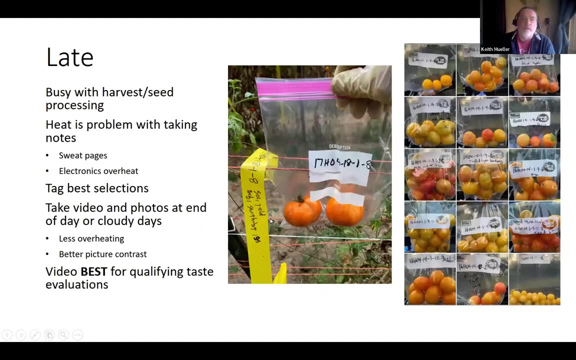 through and i'll count the uh number of fruit, i'll notice any note, anything that's unusual and, like i said, i'll tag the plants. but, um, it goes pretty quick and i use handwritten notes to do most of this. um, but when late season comes in it's really hot and um, it sounds silly, but i've had problems with. 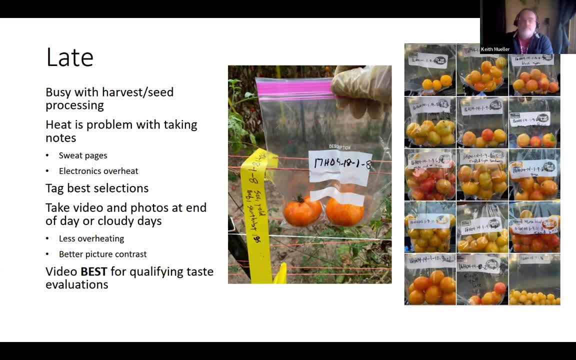 uh sweat getting on the pages and um messing up the data. so you have to worry about what pen you use and i've tried electronics, um phones, computers, even cameras have problems in the field. i have to adjust, you know when i'm taking those pictures and um, okay, i'll move it along, but this is an 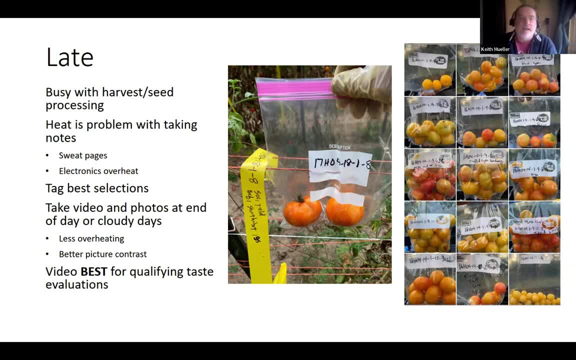 example of how i take that and tag it and write information on um. but at this point i'll switch to videos and i'll do that to um record taste because that's a better way for me to evaluate it, and i'll just stop there and i'll do that to um record taste because that's a better way for me to. 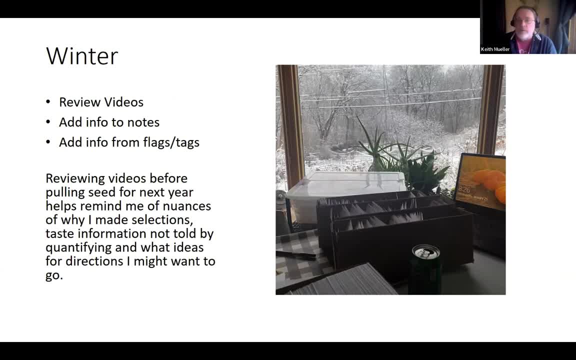 evaluate, and i'll do that to um record taste, because that's a better way for me to evaluate- evaluate what I actually thought in the field- than using numbers. Numbers don't really mean much to me, And so I'm in the point now of where I'm looking at my videos and pulling seed for next. 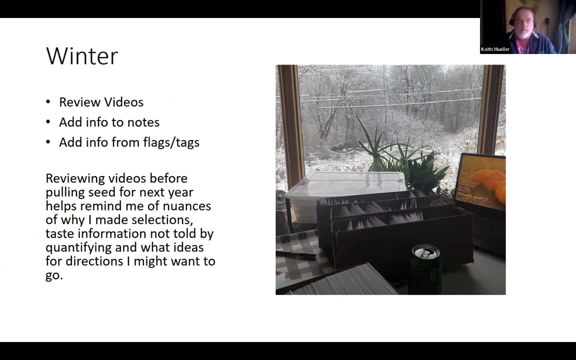 year And I'm actually hearing what I thought about that that I tagged and marked. you know, this is my thought on it. This is what I experienced when I tasted it. It's not just like one from five value, It's actually what I was thinking, what things, and I just don't have the 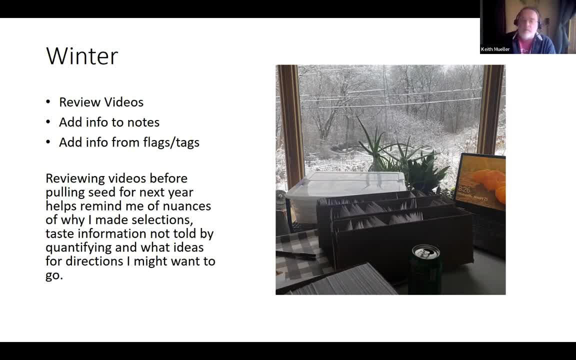 time to write all that. So that's how that process has helped me And I've changed that because I used to take data on size and everything else, bricks and it's. I'm not writing papers, So it doesn't really matter to me that much, And it's those observations I make within the videos. 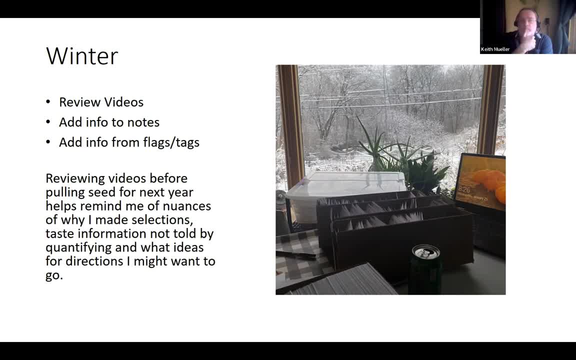 that really helped me make decisions About what I'm going to put out next year and then what I tagged, But that's basically what I had for you. I hope I didn't go over. I came close, I know, But I'd like to thank the following people: 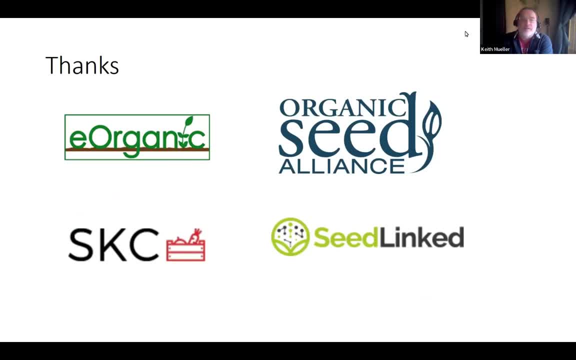 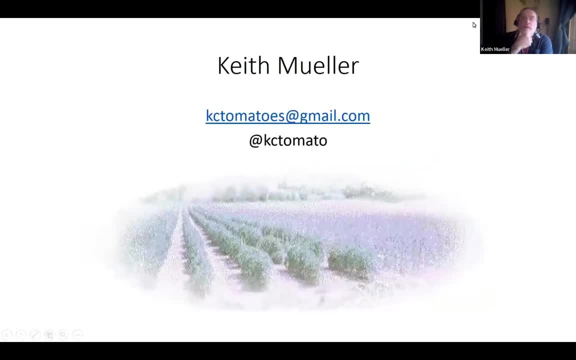 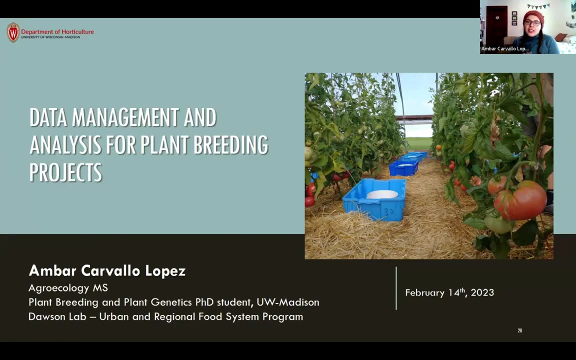 and I missed some logos in here. So, and if you'd like to get ahold of me, I think, oh, there was supposed to be one. That's my contact, But thank you, Hi everyone, I'm Amber Carvalho. I'm a grad student at UW Madison and I've been working with tomato. 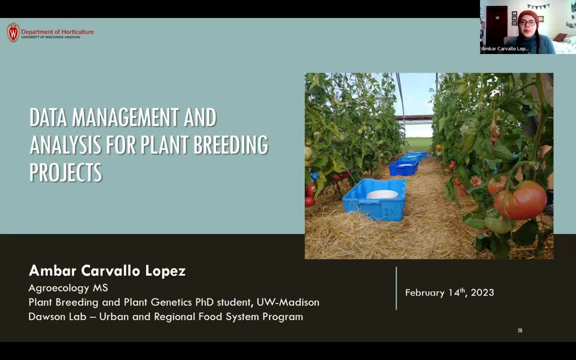 breeding for the last four years. So I think I didn't know that there were going to be other tomato people talking to us. So it might be a little bit heavy on the tomato side. but I'll try to also check in more general ways. So getting in the same page, as I said, most of my experience. 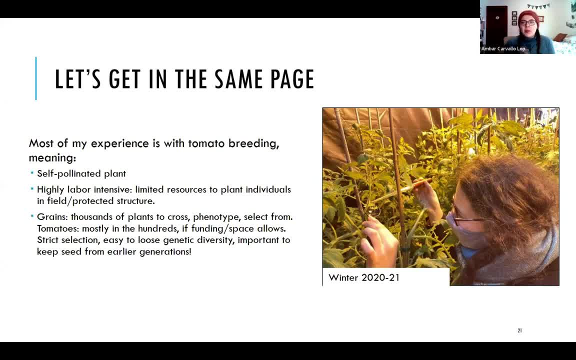 in breeding is tomato, Which means that I've been working with a self-pollinated plant. It's a very highly labor intensive crop, So we have limited resources, either if you're a private breeder or working at university or public. You can only get so many plants in your field, And I put here, for example: 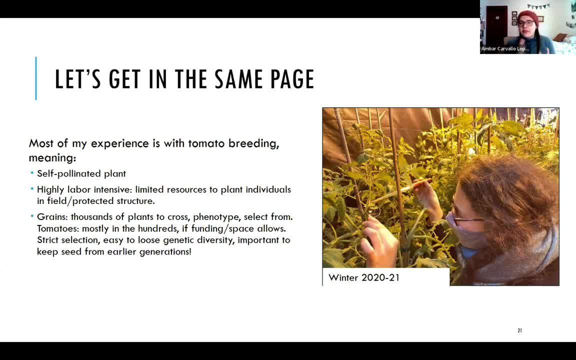 in grains. you can put thousands of plants to grass and phenotype and select from in a field, and in the same size field You can only put maybe 100 plants of tomatoes if funding space allows. So there's strict selection. As Keith said, it's easy to lose genetic diversity because you can create bottlenecks, So it's 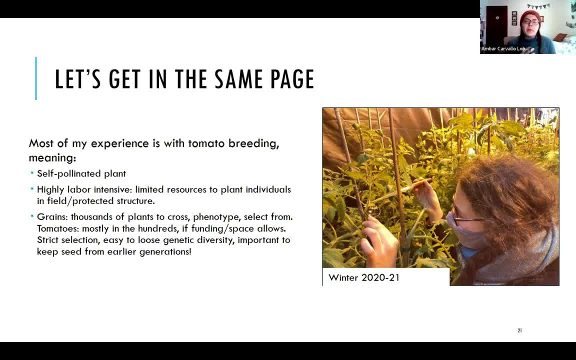 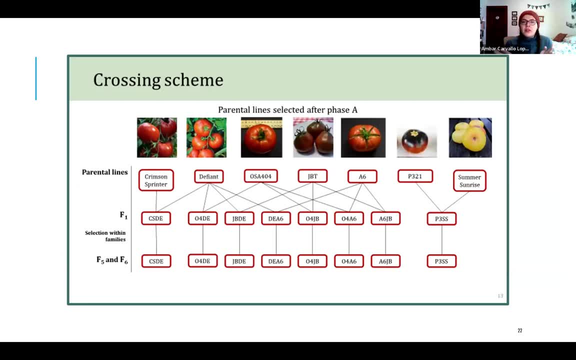 important to keep seed from earlier generations if you want to bring back some diversity into your populations. So I thought I would show you some of our- well, one of our breeding schemes for one of our breeding projects. So we have in the top, multiple varieties that we use as parental lines and we developed hybrids or 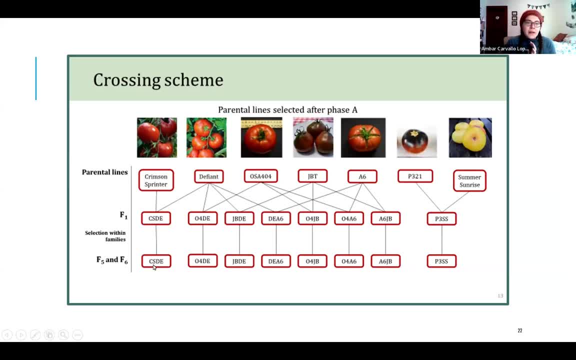 F1s, And then we advanced the lines and selected in the field. So- and this is only a portion of the grasses that we did- So how do we keep track of everything? That's kind of like what, how I'm going. 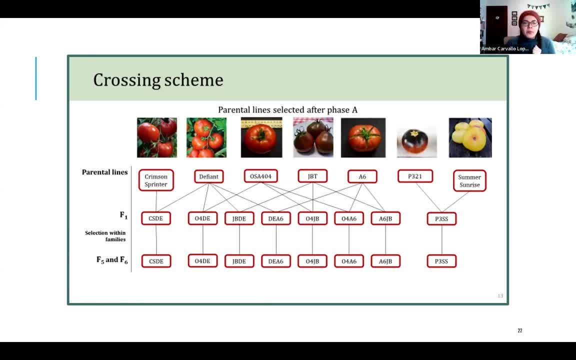 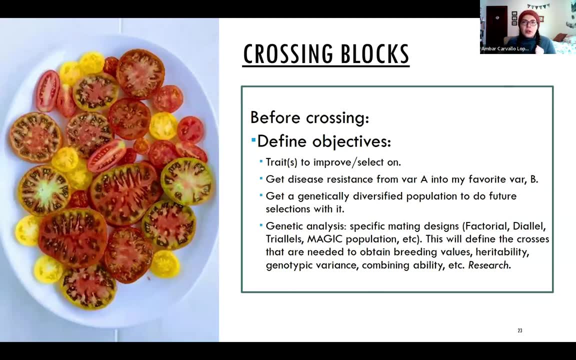 to focus this part of the presentation, Very related. Okay, So the first thing that we need to think about is: what are our objectives? A breeder- private breeder- might be trying to find interesting traits, So might want to keep a diversified population always. But if we're going to do that, we're going to have to keep a very diverse population. So we're going to have to keep a very diverse population, But if we're going to do that, we're going to have to keep a. 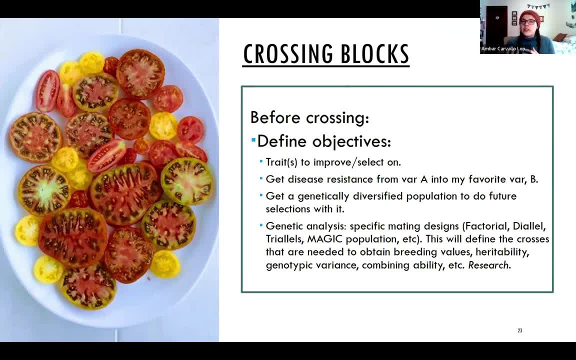 diverse population. But if we're in the field, if you're a farmer or a gardener or a starting breeder, you want to have a clear idea of what traits you're going to be focusing on, And it's usually not single trait, they're going to be working on multiple. 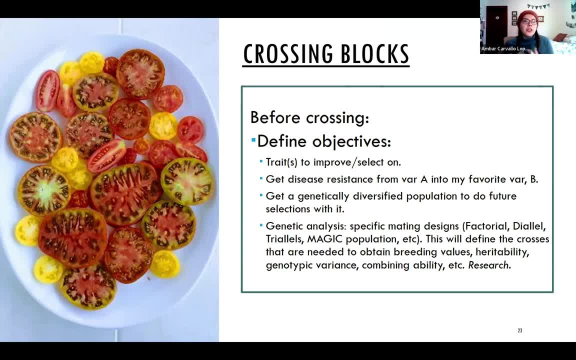 traits at the same time, which is usually a challenge because there can be some negative correlations, especially with flavor, fruit quality and size and production. with flavor, fruit quality and size and production. um want to integrate a disease resistance from variety B, from variety A, for example, into your favorite. 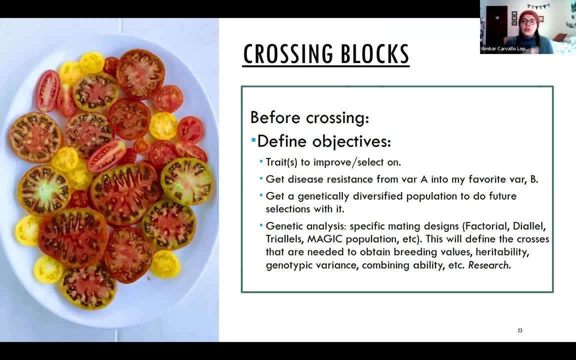 variety, which is variety B. Maybe you just want to maintain a diversified population or maybe more in the research aspect, you want to do some genetic analysis where you are going to use some specific mating designs like factorial dilow, trilow, magic populations etc. And this will really define. 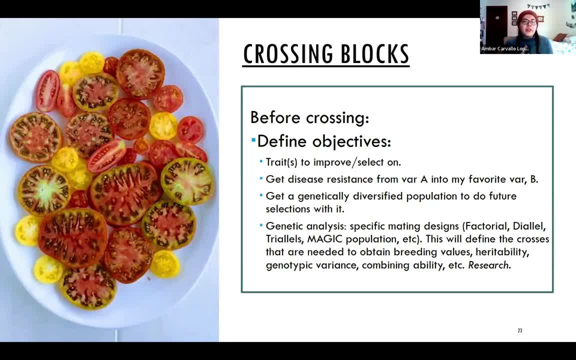 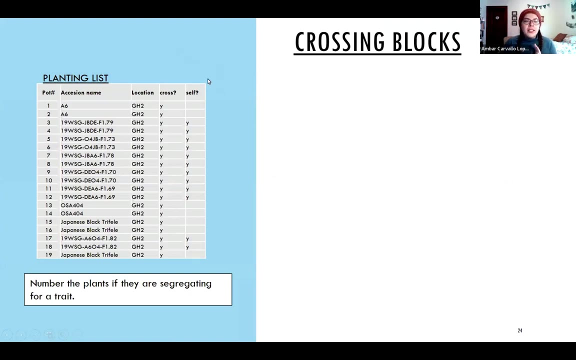 the crosses that you need so you can obtain the breeding values, heritability and other genetic analysis that you might want to obtain. So, before crossing, defining the objectives, of course, is key, And so here I have an example for a planting list through the winter of 2019,. 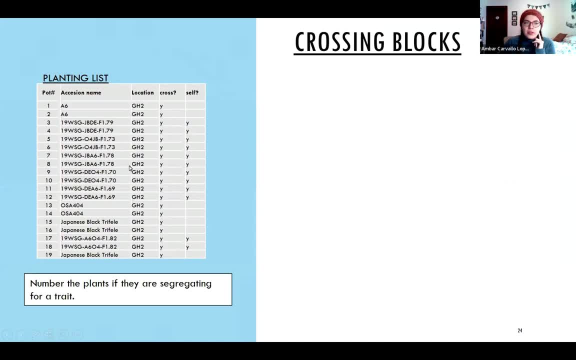 I think no 2020.. And so I have the accession names of all of the plants that I'm going to have to cross, And for some of them, for example, I have A6, which is a variety, OSA 404,, which is an organic seed. 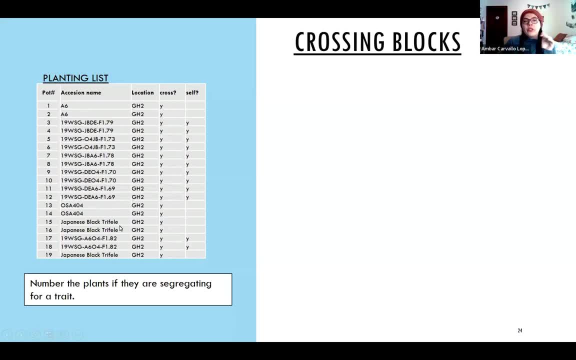 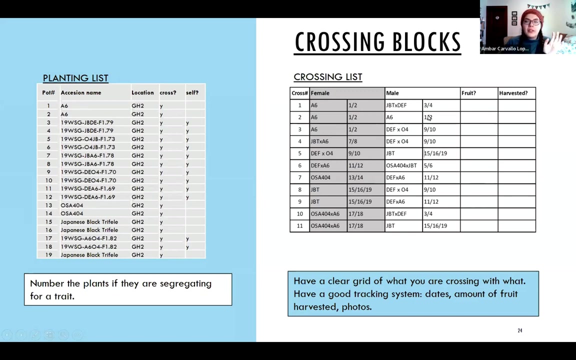 alliance variety. Japanese black truffle. those are all stable varieties, so it's not necessary to number them, But others that might be segregating. we want to keep track of each specific plant, which would be the pedigree tracking. So, with this list on hand, what I do then is make my crossing list. I'm going to have a crossing. 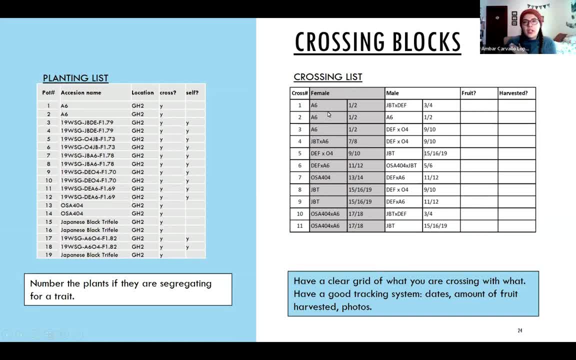 block that's going to define what do I need to cross with what variety. So this is very helpful to know where I'm going to have to go get the pollen, which plants I have to get emasculated. maybe I can do both ways: use one as a female and then use it as a male. Sometimes there are some. 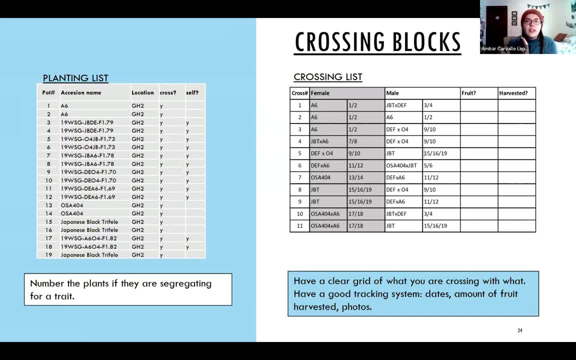 like differences. There can be some like maternal effects in what you obtain in the hybrid, So I always try to make both crosses. I mean the cross in both ways. So it's important to have a clear grid of what you're crossing and that allows you to keep a good tracking system of the date that 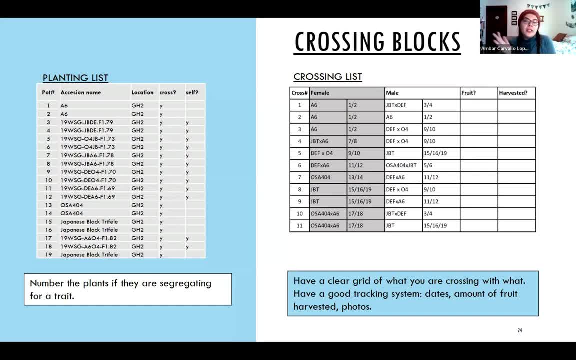 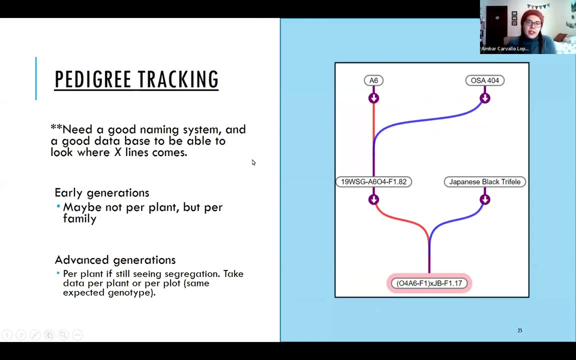 you planted, the date that you made the cross, so you can then confirm that you have the cross available for harvesting In the future, maybe take some photos? and how do we create a pedigree tracking? So you need a good naming system. Keith showed us that he uses the year and the letter that represents if it's a hybrid. 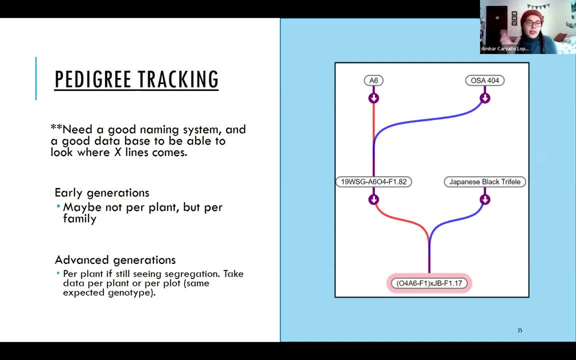 or a selfing, and then the number of that cross. That's, I would say, a very traditional way And we use something very similar. And so in the early generations maybe you don't want to keep up per plant numbering or tracking, but maybe per family, which is what also Keith showed earlier. 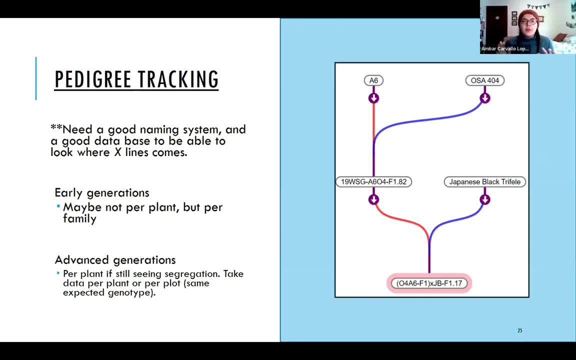 And then in the advanced generations you want to keep- or that's what I like to do- at least keep up more per plant separations. So if you still have segregation, you can make sure that you have all the traits that you want, that you're going to be able to make sure to choose and then be able to track that specific line with those specific traits that you like. 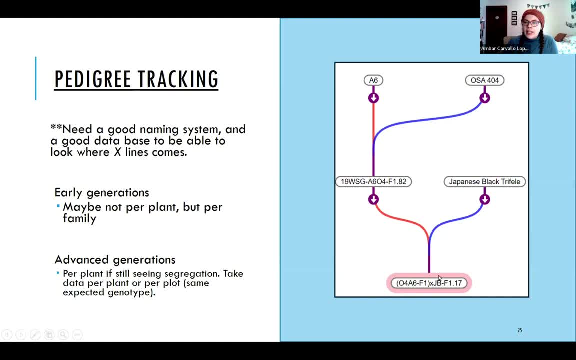 So, for example, in this figure we have this hybrid here, at the bottom We have an 04a6,, which is an F1, that we crossed with a Japanese blacktree feld, and that's an F1. And what I'm showing you here is that we have both of the parents. 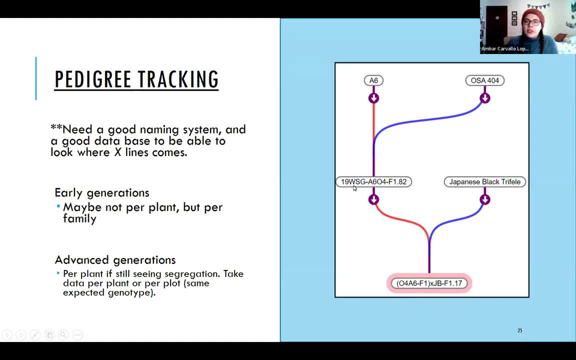 This is ignore the first, the first one, this one, the second one, the third one, the fourth one, the fifth one, the sixth one. first, numbers and letters are year and location. so these are the parents, and then I can go back. 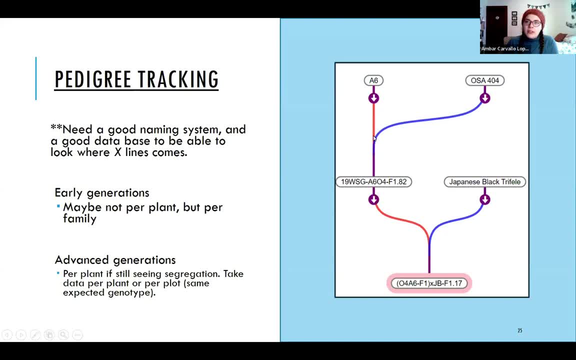 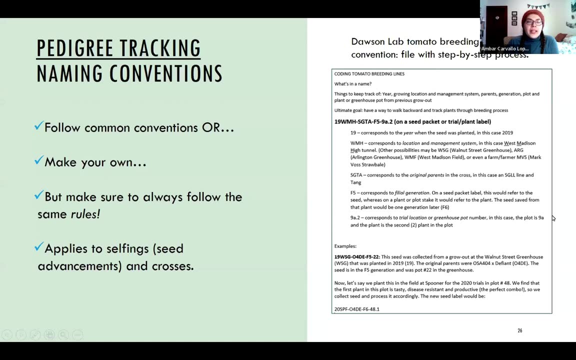 again and look at the parents of this, which is also an F1, and see that it was A6 and OSA 404. so this would be like a triple, a triple cross. it has three different lines in it and, as I was saying, having a naming convention is very important for you to be able to. 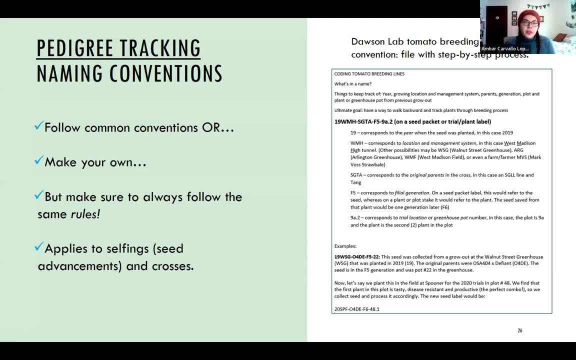 be able to track what you've been doing. there's the common conventions that you can follow, or you can make your own, but you have to make sure to always follow the same rules. we at the Tasson Lab have a reading protocol on how to label everything. so, because we have students coming, 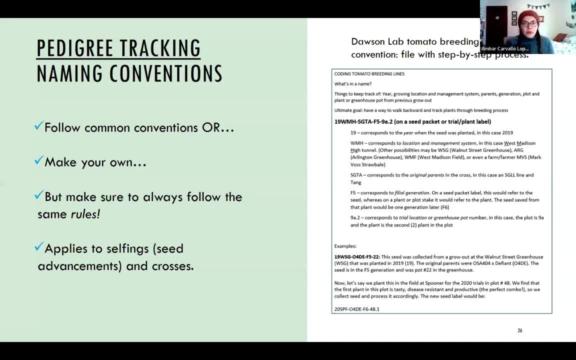 in and then graduating, and then other students taking over. it's important that we have a very clear process of what everything is, what happened in the past, what was crossed with what, which lines were selected, etc. and also have good notes on whatever it is that you're selecting. so, for example, very briefly, we have this name: that 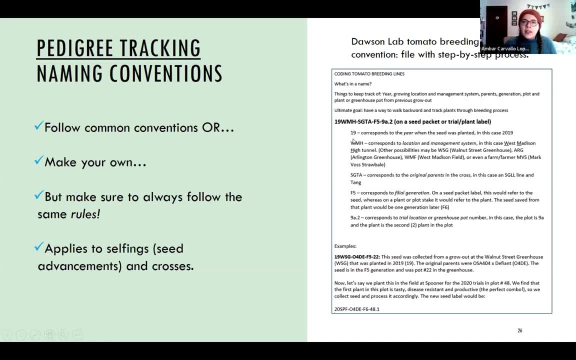 indicates the year 2019. this three-letter code is West Madison High Tunnel, that was um in the summer of 2019, then SGTA corresponds to the hybrid, but the original crosses, which were those two, and then F5 would be the generation and then, depending if you have blocks or 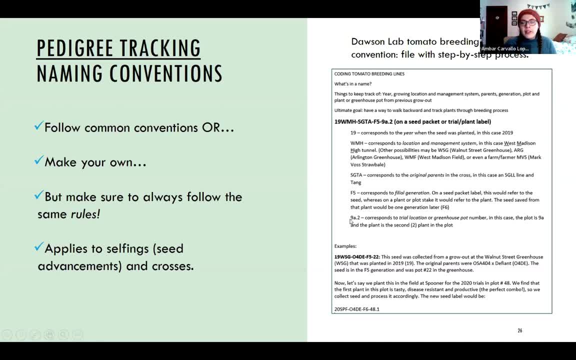 um plots with a certain amount of reps. this one was the plot 9, um A and then plan 2. but then that it's gonna depend on your, how you plan your system. um, and this also applies to cell fins- not only so you make the cross, you want to keep track of the track of the cross, but then you're gonna make cell fins. 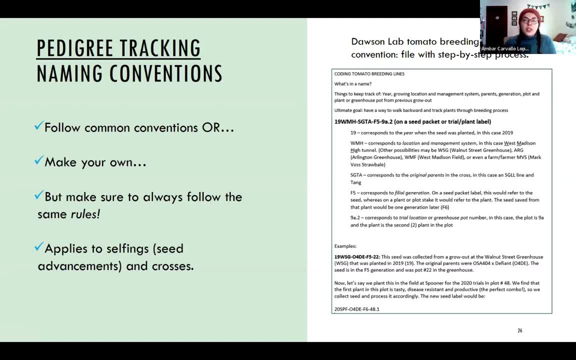 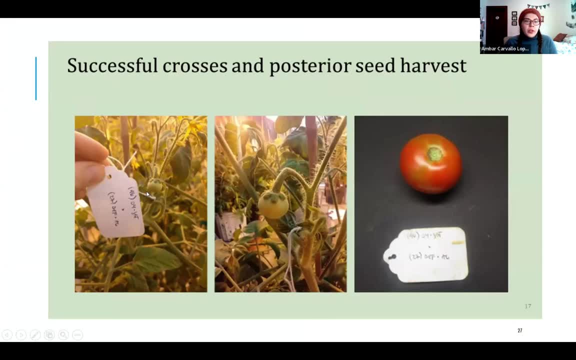 and you want to make sure to also keep a good record of those. so, for example, this is a cross that I made in the winter. we usually make, uh, most of our crosses during the winter- and I have here the number of the plot that I use, the name of the female, the male, again the number, the name of the accession, then 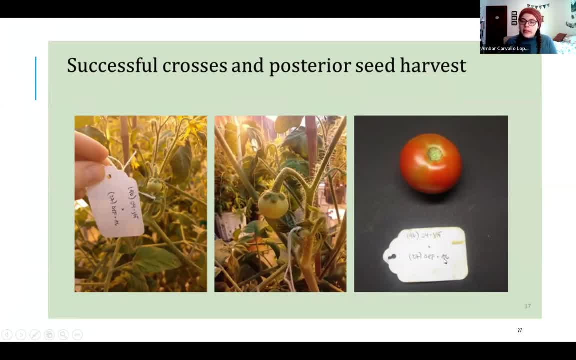 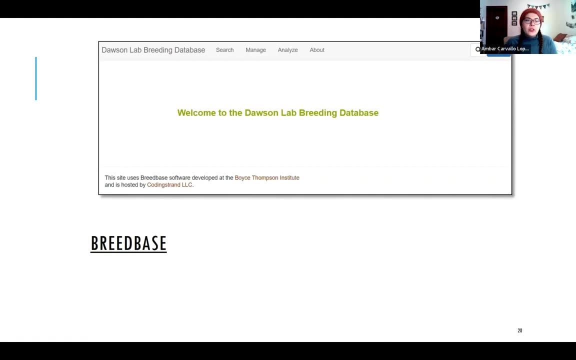 this has been confirmed, and then, when we harvest, we have that information that allows us to go back um in in previous, to previous generations, um, and I briefly wanted to show you something that that we use, that it's called brief base, uh, that, as a dozen lab we have access to, which has been 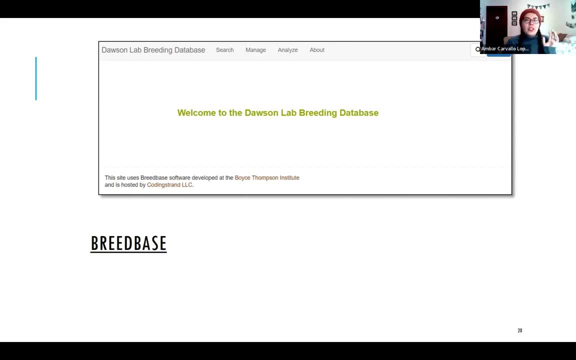 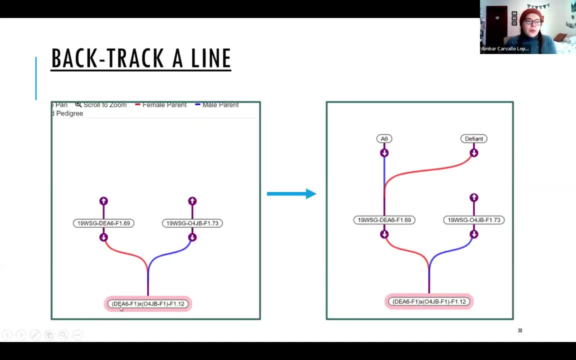 great to uh be able to visually track our crosses in our lines. um, we can put the name of an accession here and um, as I show you before, we have here, for example, it's a four-way cross. we have a hybrid, a hybrid that we are crossing to make another F1, and I can see the parents which were each one a hybrid. 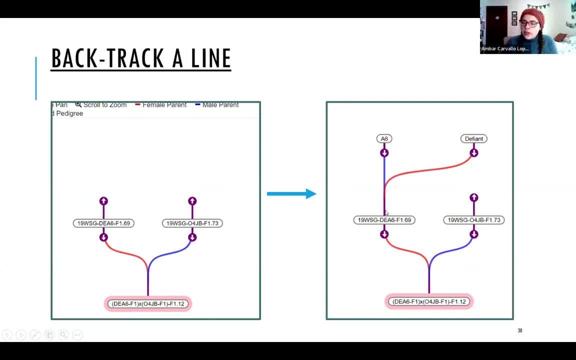 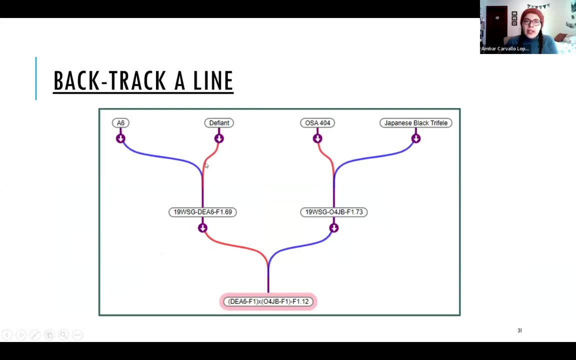 and then, if I click on them, I can know where those favorites came from, um. and so now here I can see that we have, uh, four different lines in this cross, so a very diverse cross. uh, that in an F2 is probably going to be segregating a lot. 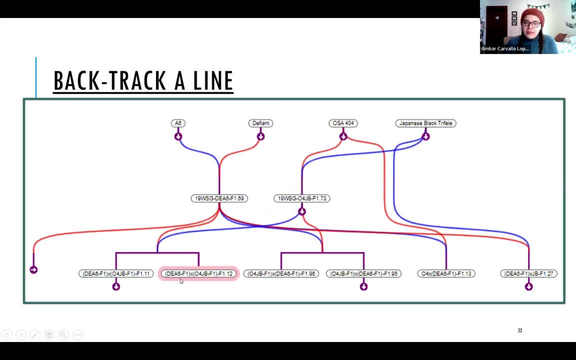 and then we can also see all their related um crops- I'm not, not crops, I'm sorry- lines. this is the one that we were looking at and this is part of um, uh, kind of like a magic population, so we wanted to be able to cross everything with everything. 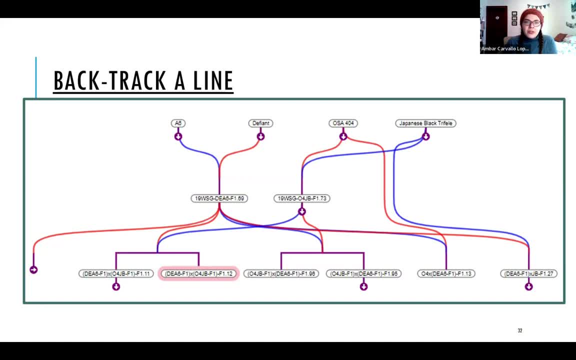 so there are many related lines that use the same parents but cross them with other the parental lines. so this is a very good um program or tool to visualize what we've done, but then the only way to have this is have a very organized tracking system in your computer. 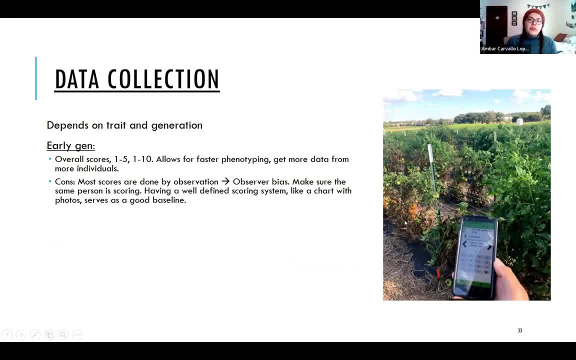 in an Excel file, for example, where you have the information of um what you cross, um when you crossed it, Etc. and in terms of data collection, I think it also depends on how detailed the data is, depending on how, on what generation you are- um early generations, I usually 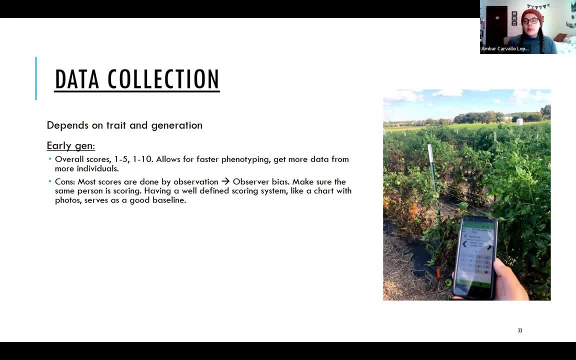 what we've done mostly is give scores- maybe productive productions score 1 to 5, 1 to 10,, of course, having a very well-defined way to assign those scores, those numbers. This allows for faster phenotyping, so you can get more data from most of your individuals. 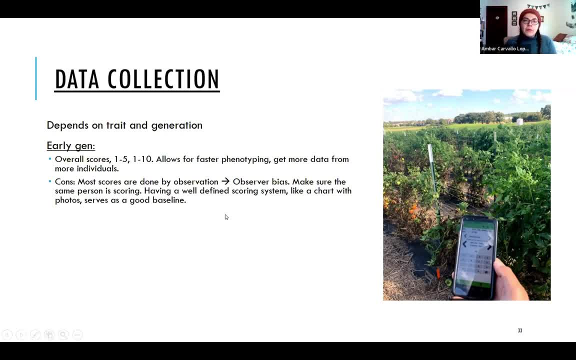 or hopefully all of them. Something to keep in mind with that way of taking data is most of the scores that are done or are taken by observation, so there's going to be an observer bias. You either have to make sure that always the same person. 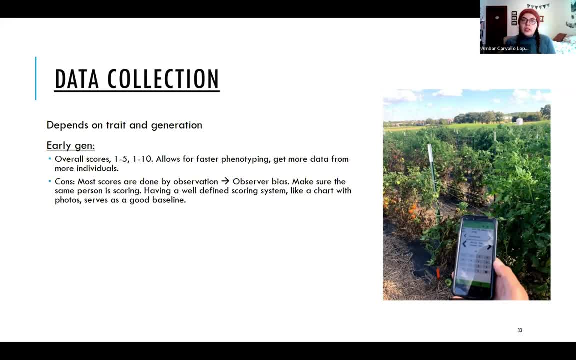 or people are walking the field and giving those scores, or also, at the same time, have a chart with photos that can help people define which score to give. This also works with the season. So you want to do a lot of analysis and make sure. 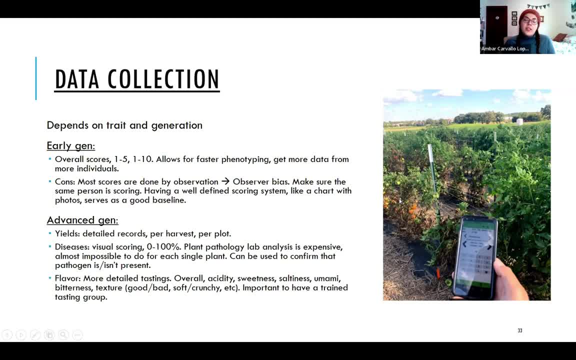 that you're calculating what the data are, So you want to do a lot of analysis and then you can give all of the scores for each season. This is something that is very important. It's important to have a really good comparison between lines. 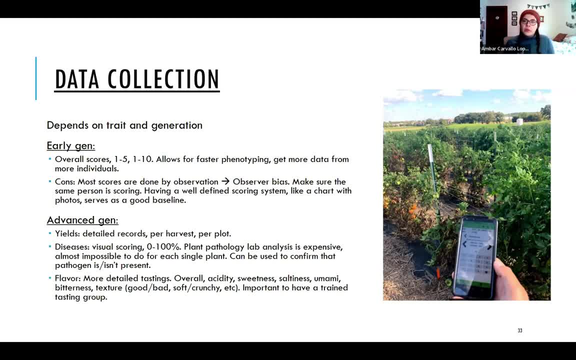 So for diseases again, usually we continue with visual scoring 0 to 100% of the plant affected with certain pathogen. A plant pathology lab analysis is expensive, Almost impossible to do it for each single plant, but it can be used to confirm that. 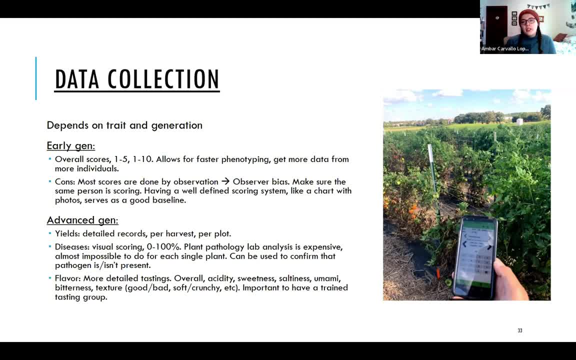 the pathogen is or isn't present. So you want to make sure that what you're seeing it's the fungi or bacteria that you are working on or selecting for resistance, for, For flavor. there can be more detailed tastings in the advanced generations. 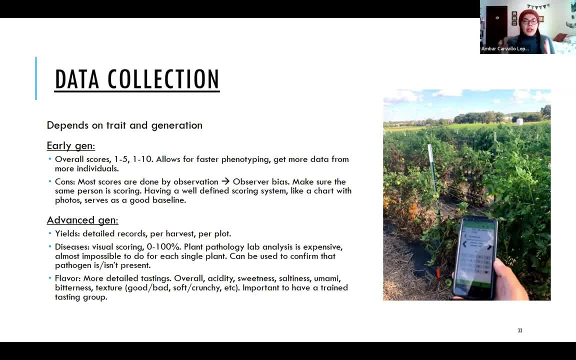 We usually have a trained tasting group and we rate overall lightness, acidity, sweetness, umami, bitterness. If it's other crops, you can also evaluate saltiness, the texture, et cetera. So we also make sure to have good, more substantial comments from the taster and that we don't 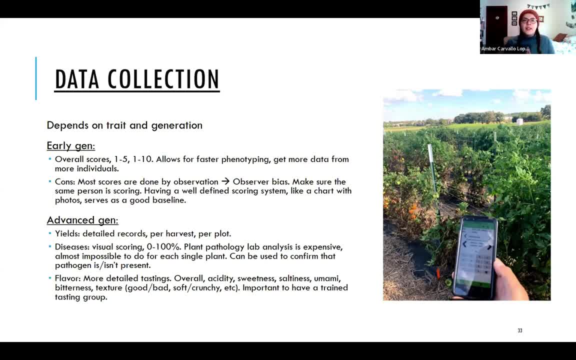 have only a number because, as Keith said, sometimes The numbers are are hard to understand. One person may give a one, another person might give a two, but maybe they experienced something similar. So having those comments are very important to us. 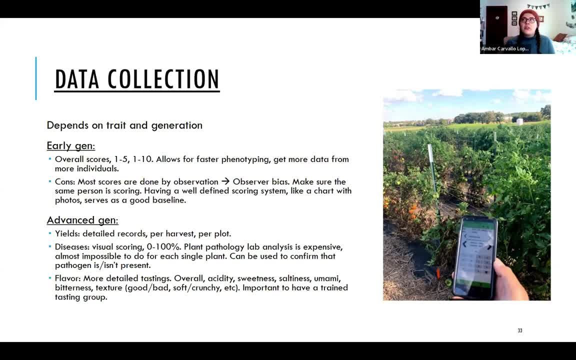 And also discussing after a tasting gives us a better idea of in the moment of what worked and what didn't work. And here in this photo I'm showing I'm taking disease data collection, But We love to try to get more information out. 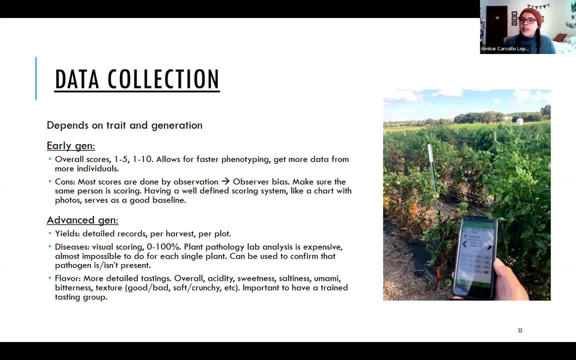 And I'm not saying that it's all in our head, because you can see there's a lot of septoria, very common here in the upper Midwest, And so I score that On. And there's this app called Field Book that allows you to upload all your your plot to. 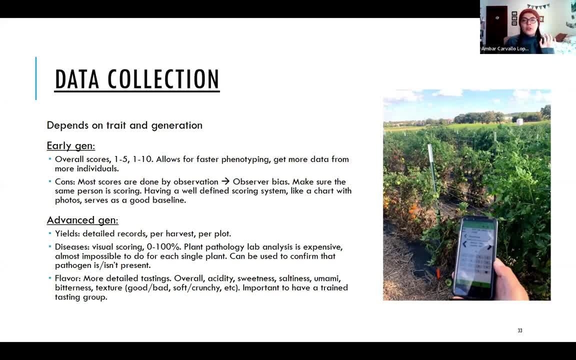 mention not dimensions but the plot numbers, all your plot information, your field information, And then you can take The data very easily by just typing a little bit of what you like. And that's that's where we what we that. 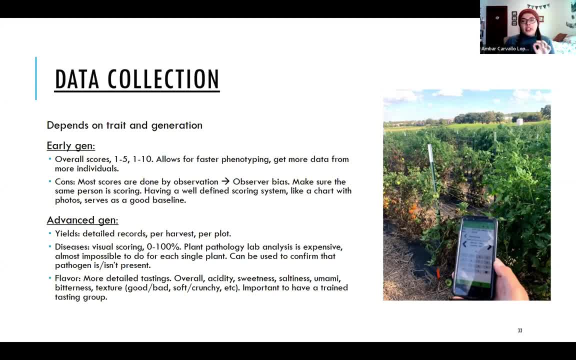 And then, lastly, is a very popular tool, And this is- this is a good example If you're interested in, let's say, you were in the natural history. you know what, what. what are you looking for? just you know, pressing the number that you are assigning to that specific blood, As Keith. 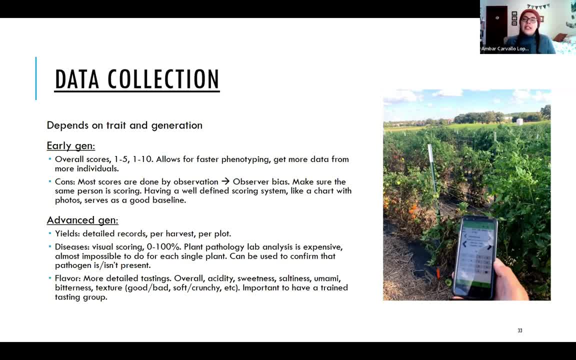 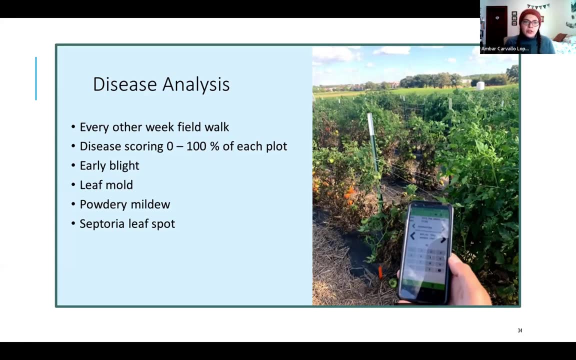 mentioned also, electronics tend to heat up, but it has worked fairly well for me. I've taken all of my disease data with that and other observational traits For disease analysis. this is a slide that I used for previous presentations to just wanted to give you. 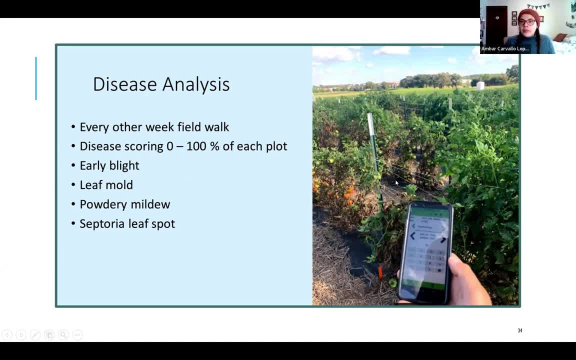 an example of what diseases you could evaluate in the field. For example, early blight and centella leaf spot are easy to see in the field And then, if you're in the high tunnel, leaf mold and powdery mildew- all of them. I can take that data in a single moment while I'm walking the. 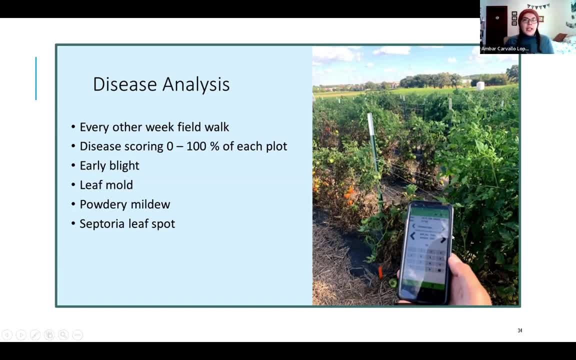 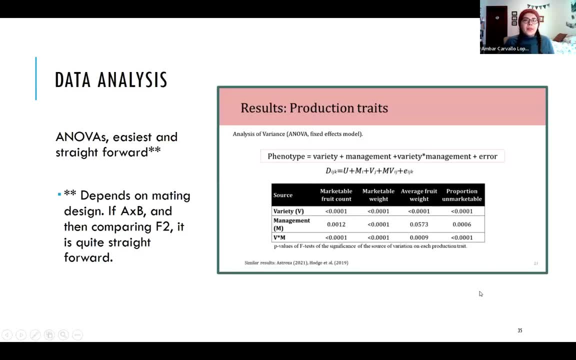 field. So that's very useful And then I can download an Excel file and I don't have to do any transcribing of field notes or stuff like that. And for data analysis, ANOVAs- a variance analysis is, I think, the easiest and the most. 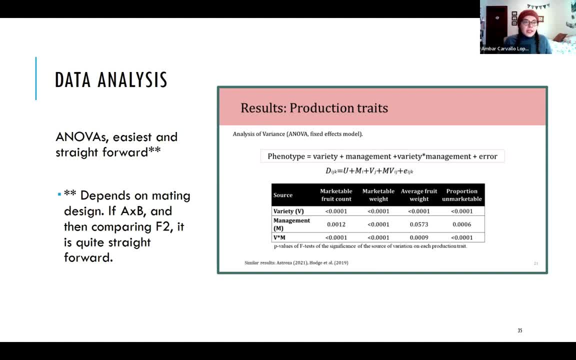 straightforward. Of course, it doesn't apply for every system or every trait. It really depends on the mating design. If we're talking about an A by B and then comparing F2s- F2 lines, that's really quite straightforward Here, for example, this is also a slide that I 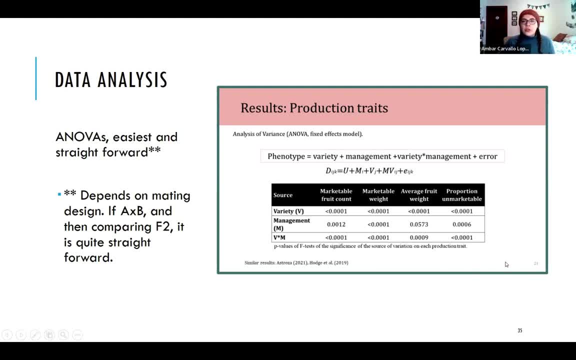 brought up in the previous presentation. So this is a slide that I brought up in the previous presentation. So this is a slide that I brought up in the previous presentation. So this is a slide from another of my presentations. I was given the results from a trial that we had. 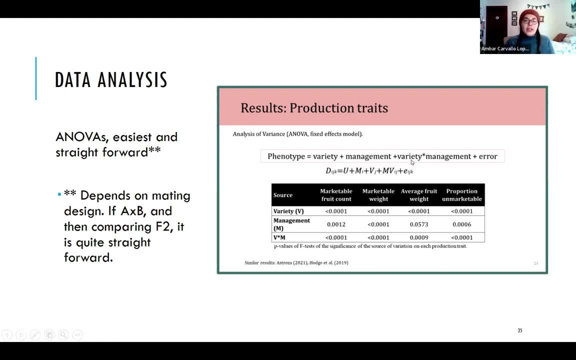 two management systems: field and high tunnel. We had the varieties, And so this is the model that we built. And then we have the results of the ANOVA. which components were significant to the phenotype that? in this case, we took the marketable fruit, count the yields, et cetera. 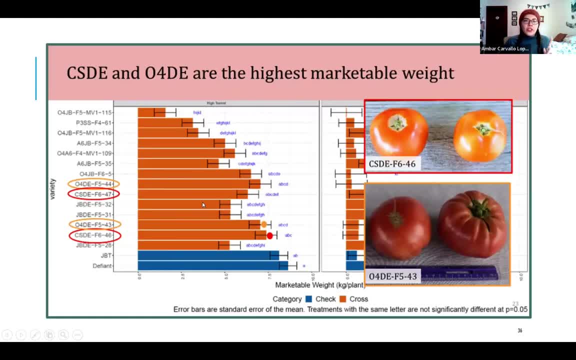 So this is a slide that shows the results of the ANOVA, And then we have the results of the, the yields of the different lines that we evaluated that year in our field. So we had multiple F5s, F6s, And so I can easily see what had a higher production and what didn't, And also 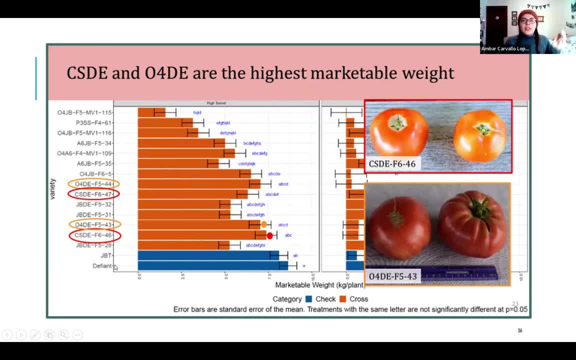 we had our checks. It's always very important to have your check varieties to know if you're making any progress or not. And here are the photos. But this was just a part of a whole other presentation, So mainly the take out here. the takeaway here is: with an ANOVA you can get a lot of. 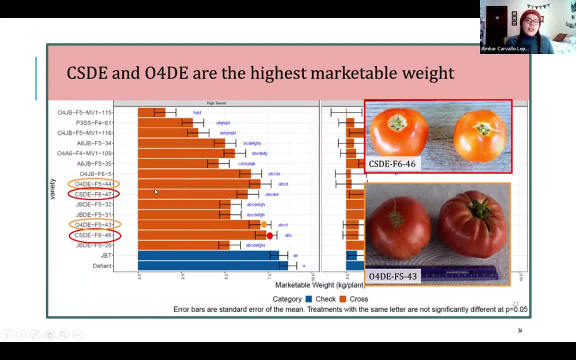 information. You can also do a variety trial and compare different varieties, advanced lines, like we're doing here, And you can do it with most traits. Sometimes you need to tweak. You do need to do some like data transformations If you're working with decimals, for example in the 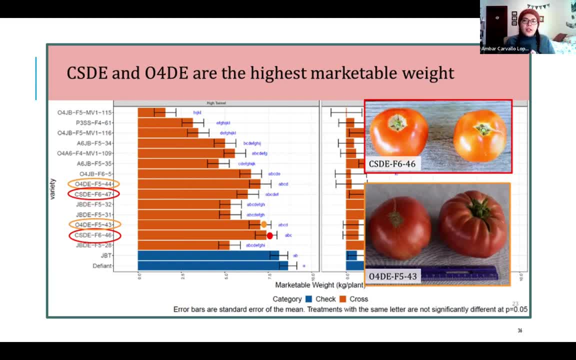 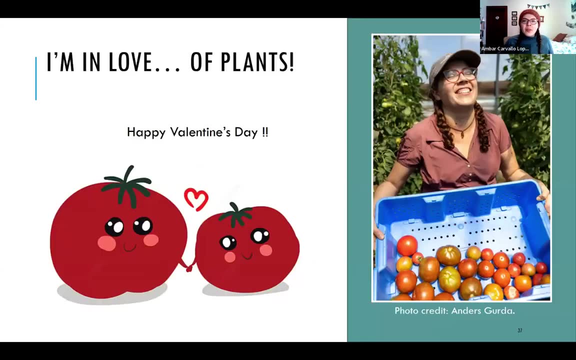 lab. you might want to do some content of a specific biochemical And it goes from 0.1 to 0.9.. You might want to transform that because otherwise you're not going to see significant differences because the numbers are too small. But that's another, And I think I'm over the time, So happy. 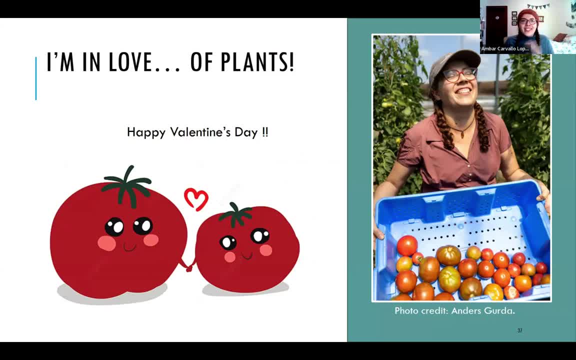 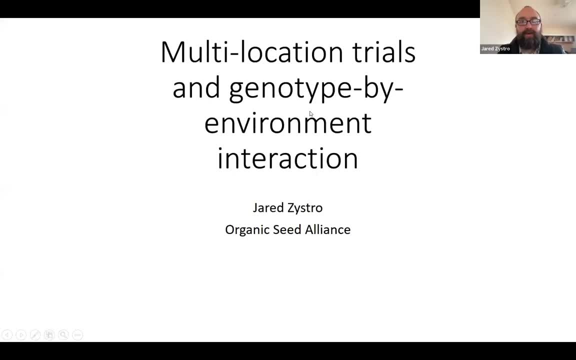 Valentine's Day And if you have any questions, I'm happy to answer at the end of the session. So I my name is Jared Zeistro, I am with Organic Seed Alliance, I am our Assistant Director of Research and Education and have a background and interest in plant breeding And I'm happy to share. 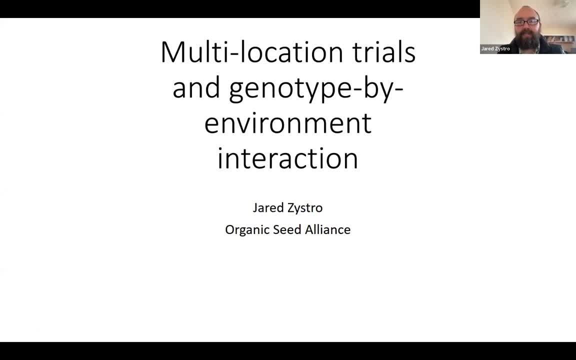 this presentation, with all these other wonderful presenters and with all of you who are watching. My piece is going to be talking a little bit about managing multi-location trials and thinking about them and understanding a little bit of what we talk about when we talk about genotype. 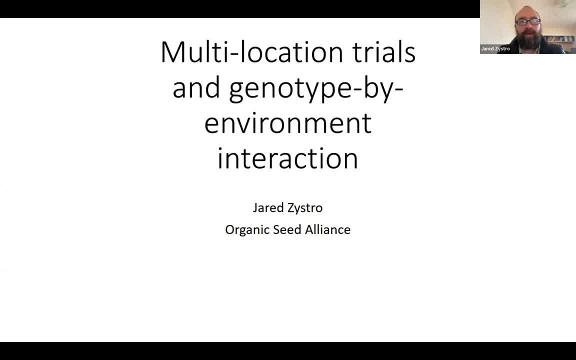 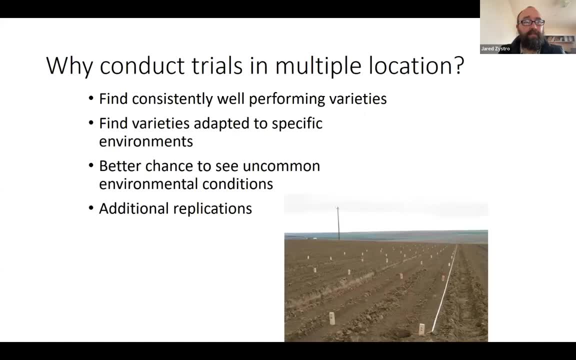 by environment interaction. So let me walk you through both. a little bit of the logistics and the theory of multi-location trials. First, a little bit of thinking about why conducting trials in multiple locations. This is something that's worth considering because it's expensive to do so. 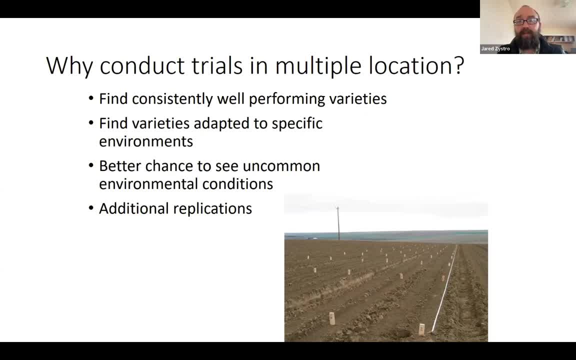 in the sense that this requires new sites, It requires potential travel, It requires extra seed, It requires new plants. It requires new plants. It requires new plants. It requires managing, you know, maybe partnering with other people, if the other sites are being managed by. 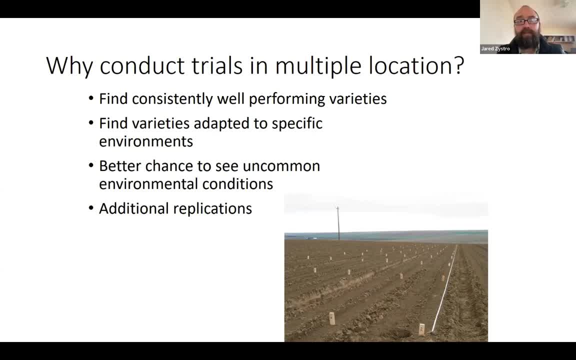 someone else. So all of these things are kind of costs that are associated with multi-location, with trials in multiple locations. So what are the benefits? Some of them might be to be able to find consistently well-performing varieties, varieties that across all of the ultimate locations, that you might want to see this variety grown in. So what are the benefits? So one of the benefits is that you might want to see this variety grown in. You might want to see this variety grown in. You might want to see this variety grown in. 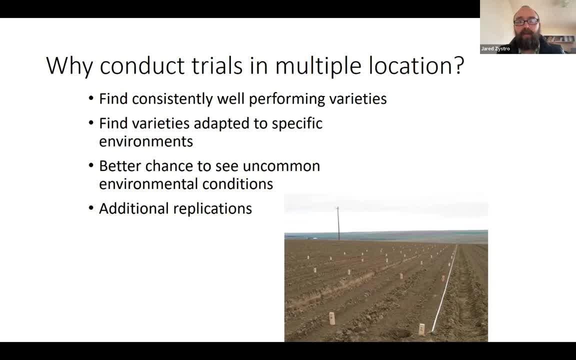 You also may be able to identify varieties that are specifically adapted to certain environments. Having more sites is also a real opportunity to see less common environmental conditions, or ones that you might not see every year in a single site or at all, unless you choose a location where 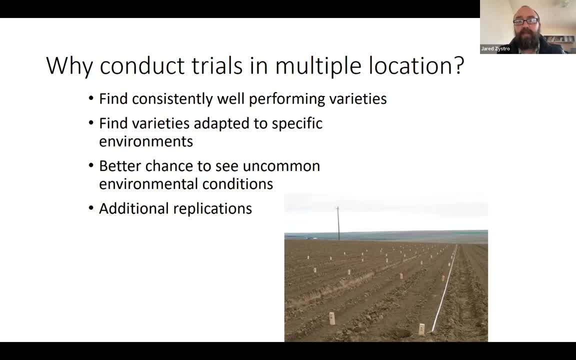 these might show up. So good example of a variety that you might want to see. examples of this might be disease pressure that happens inconsistently but generally will appear somewhere within the larger region of where all your sites are. or specific stress like a drought stress or an extreme wind storm that might affect your lodging. and last, is just that additional. 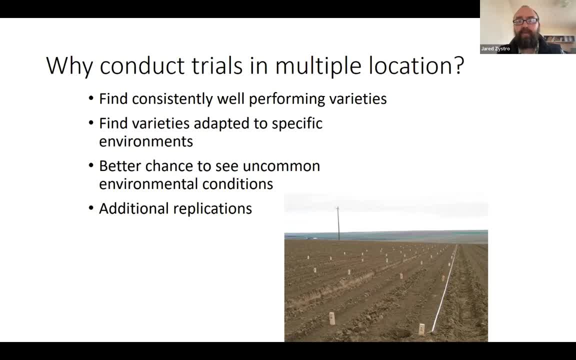 sites provide additional replications, both in the sense of it providing more data for you to incorporate into your overall average, but also as just a backup. it's not uncommon for things to go wrong in any kind of agricultural work, and if one of your fields gets completely flooded, it's 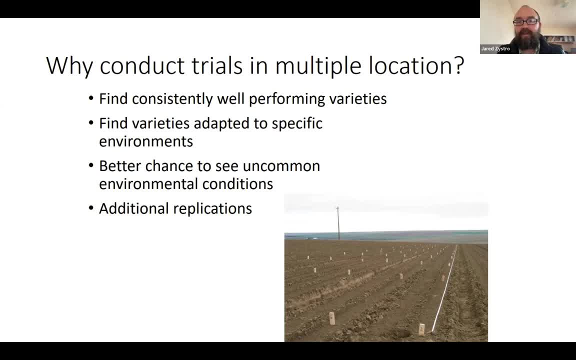 really nice that you have a second location or a third location and so having that redone dency and having that redundancy be spread out a little bit so that you know if you, versus just having, you know, replicating that trial side by side. well, if there was, you know, that wind storm, 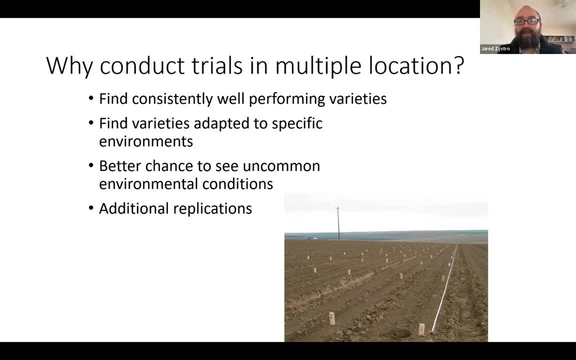 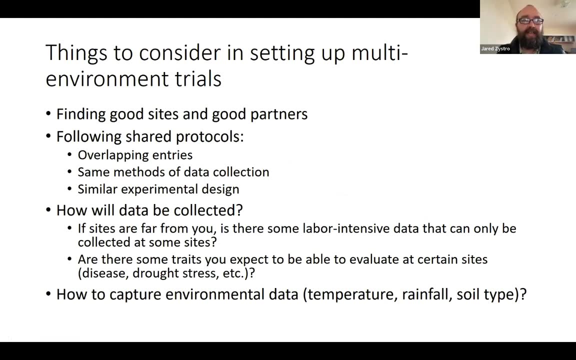 that block of crows, that flood, that still could wipe out your whole trial, but if you split it up it will reduce the likelihood that you've lost that season. so a little bit of a text heavy slide here, but just some things to consider in setting up multi-environment trials. first off is where are you going to be citing those trials and who? 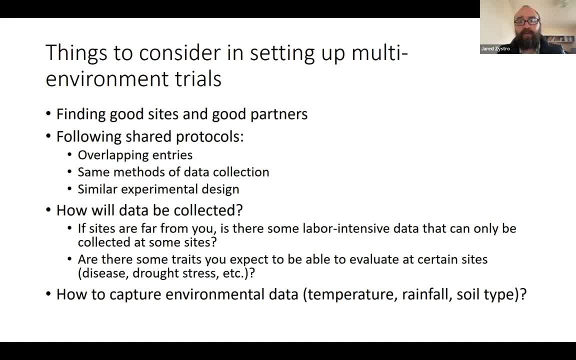 are you going to be working with? are these going to be trials you're going to be managing yourself, or are you going to have partners managing these trials do? are you and your partners on the same page with kind of the expectations around how this trial is going to be conducted, what kind of information you're collecting, how you're managing? 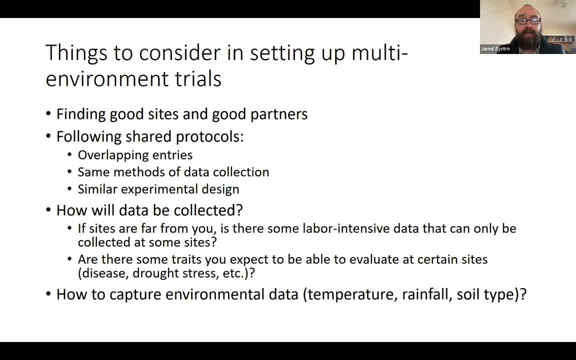 it, the amount of data you're collecting, how you're managing it, the amount of data you're using, the amount of work that it might take to manage that, and is the site a site that's that's useful to you? so, in other words, is it a place that is reflective, of sort, of your ultimate? 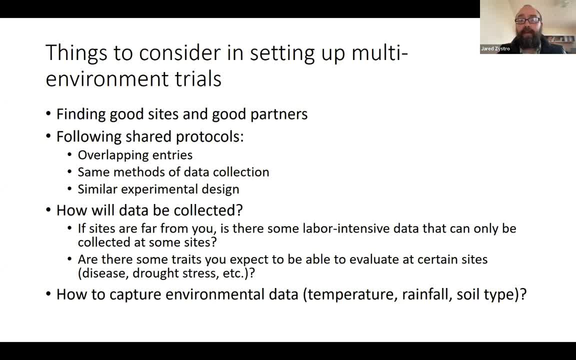 environments that you would be wanting your varieties to end up in like. is it a representative of a production environment if you're trying to have these ultimately end up in commercial production? is it representative of the right kind of climate and disease pressures and management strategies that you would kind of would like these varieties that you're developing? 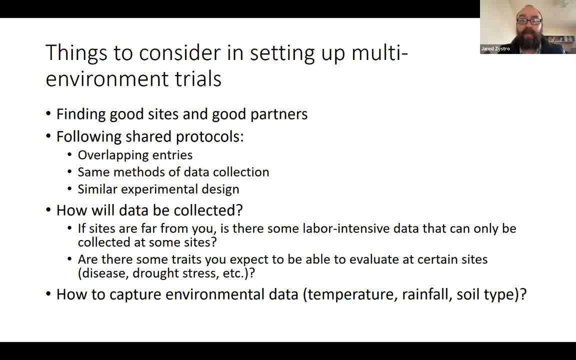 to be adapted to? in other words, is it, if you're developing things for organic, is it being grown in organic conditions? if you're developing something that's supposed to be resistant to certain diseases, are you expecting to see those diseases show up, and so on? next tip here is if you're going to be doing this in your trials in multiple locations. 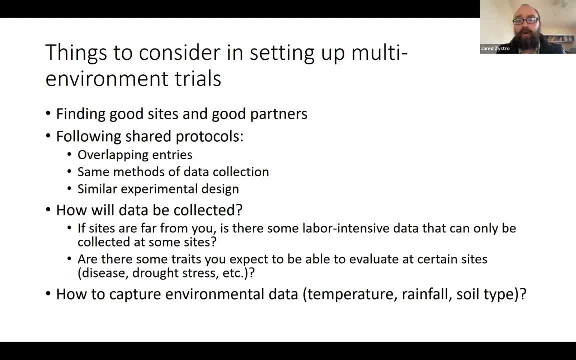 thinking about how to make sure that you are, at the end of the season, feeling like you can look at that data from those different locations as kind of a whole, something in whole cloth. in other words, are you looking at the same or similar entries in those different locations? 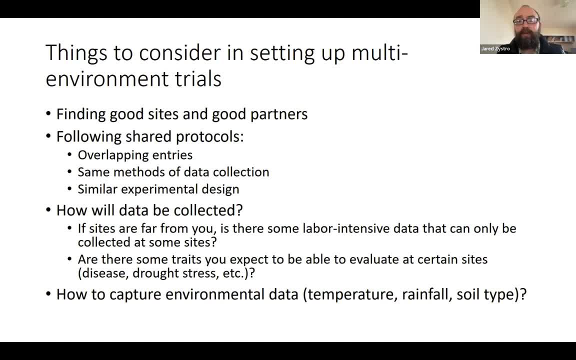 they don't necessarily have to be an identical set of entries, but you need to have enough overlap, including kind of like amber was talking about having some good check varieties in there, so that way when you're looking at the trials side by side, you can say: well, how did these? 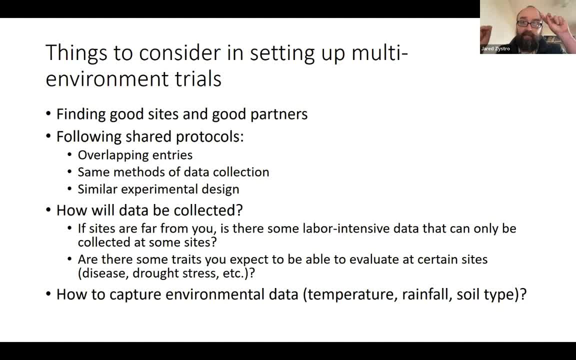 varieties compare to here versus there. you don't have the same varieties in both locations. it gets really hard to be able to combine your data. same thing goes for how did you collect the data? making sure that you have the same data collection protocols? if you're measuring, if one person's 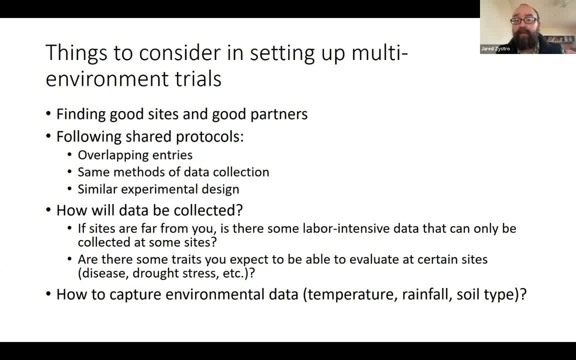 measuring flavor on a one to five rating scale and someone else only does it in bricks. how do you combine those that data later? and it's not very easy to combine. so making sure that everyone's on the same page with clear data collection protocols, if someone else is helping. 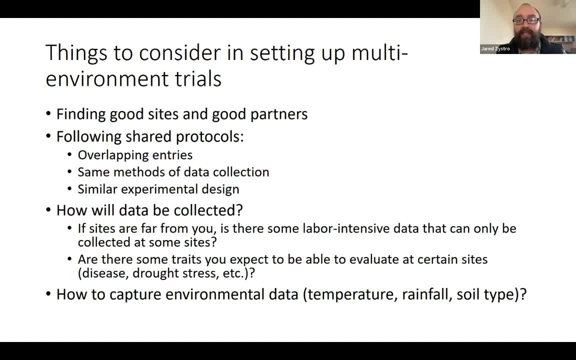 you manage one of those other trial locations. similarly, having a somewhat similar experimental design will help you be able to combine those that trial information later. so next is: how exactly is the data going to be collected? are you going to be collecting it yourself or is someone else going? 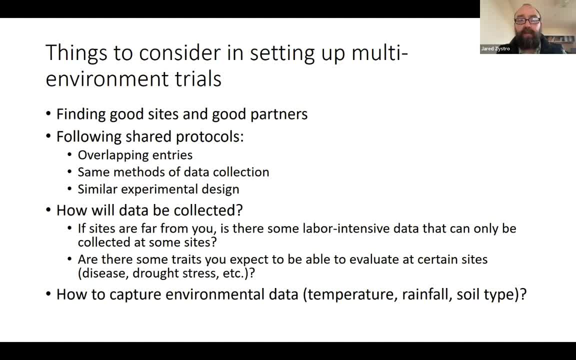 to be collecting it for you. if you're collecting it yourself and the sites are far away, there might be some data that you normally you know, if kind of you have a home trial that you can go out and be collecting data on it every day. or you know if you're collecting, you know, marketable fruits. you. 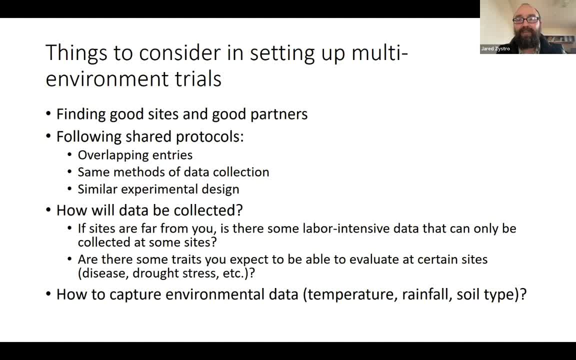 might be out there. let's say something fast growing, like summer squash. right, you can be harvesting those you know a few times a week, but if it's somewhere far away that gets harder. likewise, something like i work with sweet corn a lot and it's really sensitive to harvesting. 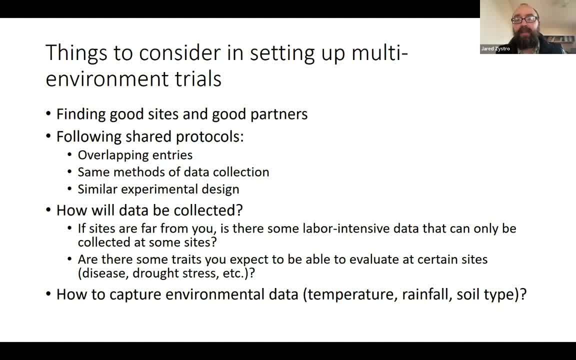 if you're doing taste testing, harvesting at exactly the right maturity date, that can be hard to get that kind of data if it's far away and so thinking about: okay, if this trial is far away, are there certain pieces of data that aren't going to really be able to be collected at that? 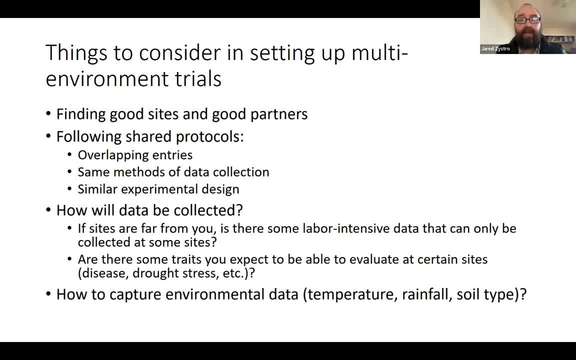 remote site and what are the pieces of data that you can collect at the remote sites, and are those pieces of data going to be useful and additive to your understanding of how these varieties perform? likewise, if you have certain traits that like going back again to finding good sites, if there, 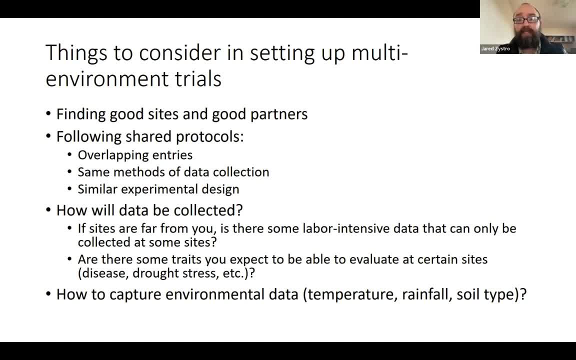 are certain traits that you're really hoping to be able to collect that you're going to be able to see at certain sites like: oh, this is going to be my drought stress site, or this is going to be my- you know- early blight site, then making sure that you've got a plan for how to collect. 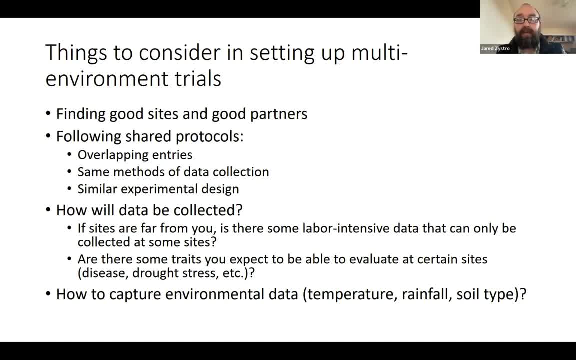 those site-specific pieces of data and can and collect them and incorporate them in there. and then, finally, how do you capture environmental data? so, at the end of the year, if you see big differences in performance between varieties in different locations, the question you might ask yourself is why? and so being able to say okay, 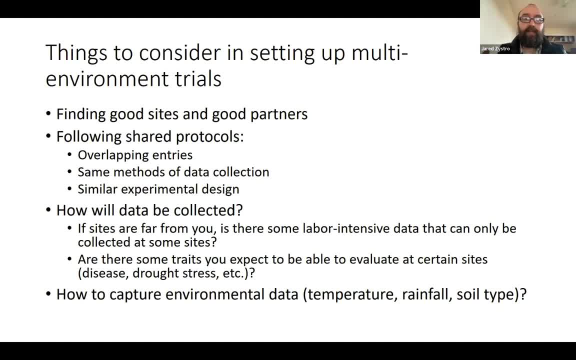 what were the environmental conditions that were different at those sites. so being able to- if you can have a weather station set up or something like that to be able to capture things like day and night time temperatures, rainfall, so on, that all can help you later on in untangling. 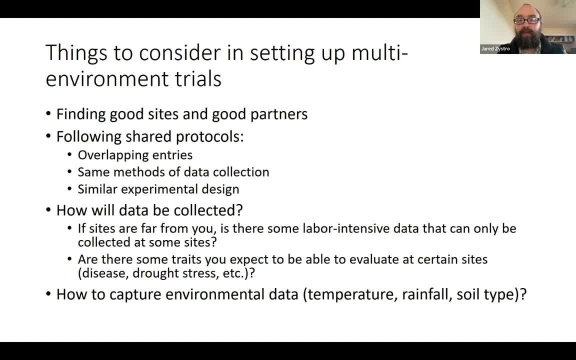 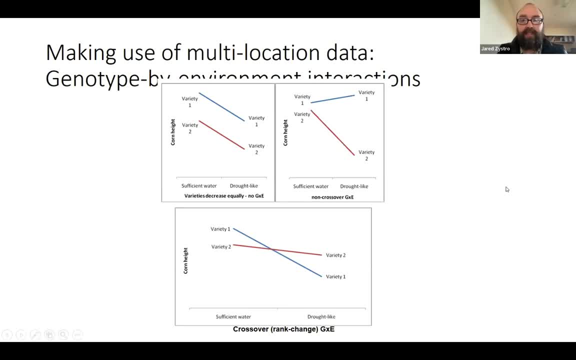 and teasing out what exactly happened in your trial across these multiple locations when we're talking about multi-location data. unfortunately, i think this slide got a little jangled up here, but the underneath that picture there it says genotype by environment interactions and so this term that you often will hear when people talk about multi-location trials or talk. 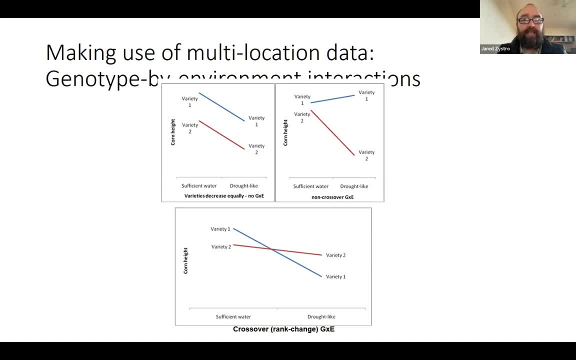 about breeding and selection is basically saying that it's asking the question of how do different genotypes, different varieties of species get their genetic representation and how do they get their genetic representation, and how do they get their genetic representation and how do they get their varieties or entries perform in different environments? And is there, are they performing? 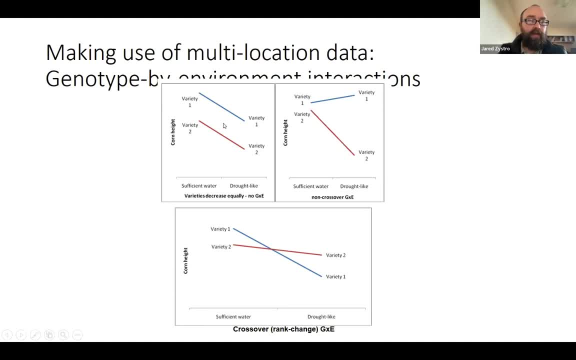 consistently. So this picture up in the upper left-hand corner of the slide here that says no G by E, you can see that there in fact are differences between the varieties and differences between how those varieties perform in the environments, but they consistently in this case. 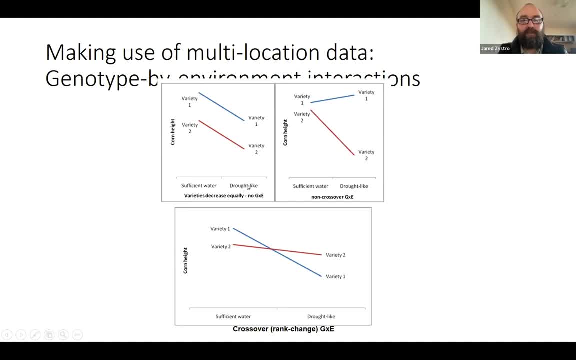 you know we're saying: oh, one of these was a high water and one was a more drought-like conditions. You can see consistently both of the varieties drop about the same amount in terms of height as they move from the well-watered to poorly watered environment. This is not. 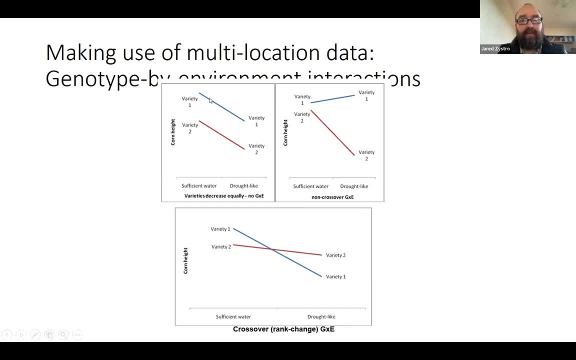 genotype by environment interaction. This is an effective environment, but the effect is applied equally to all the varieties, in this case, two varieties. The second thing is, you may see that there are differences in how the varieties perform in different environments. So this is a 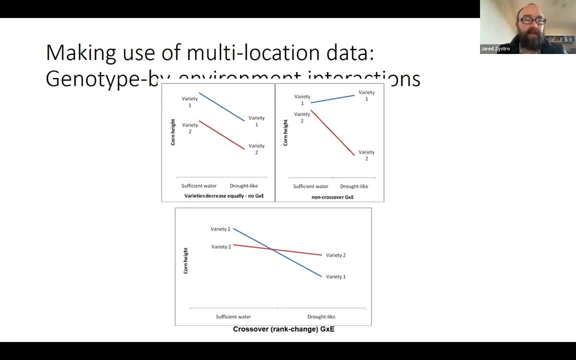 picture of how the varieties respond to the environment, in the case of sort of the upper right-hand corner. here You can see that variety one actually did about the same or even slightly better in the drought conditions where variety two really fell down. But if we were making 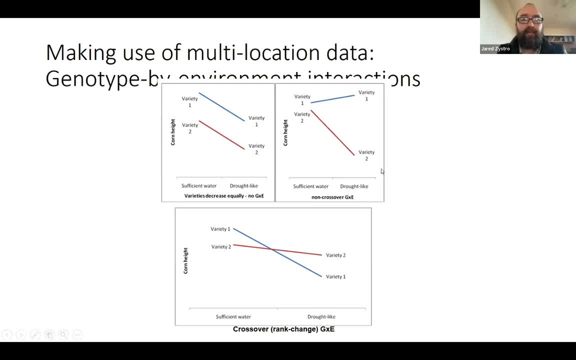 recommendations or decisions. as a plant breeder, the ranking of these varieties didn't change. Variety one was still better than variety two in all conditions. The last, that is the trickiest one to handle, is called crossover or ranking. So this is the case where the environment is affecting the varieties, It's affecting the 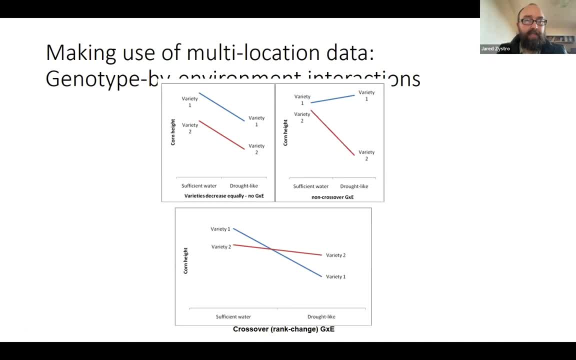 varieties in such a way that some of the varieties actually respond. they change ranks so that variety one is better when there's sufficient water, whereas variety two was better in the drought-like conditions there. So understanding what kind of environmental effects you're having is going to be the next question. 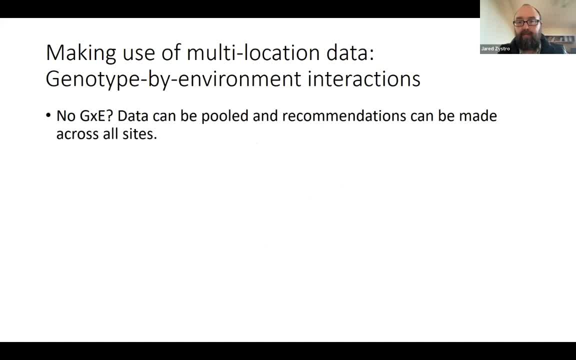 So if you don't have any genotype by environment interaction or is not showing those changes in ranks, then you can basically have an opportunity potentially to pool your data together, kind of combine across all your environments and make overall recommendations across all your sites. How do you do that? You can just take simple means, though you need to be able to do that. 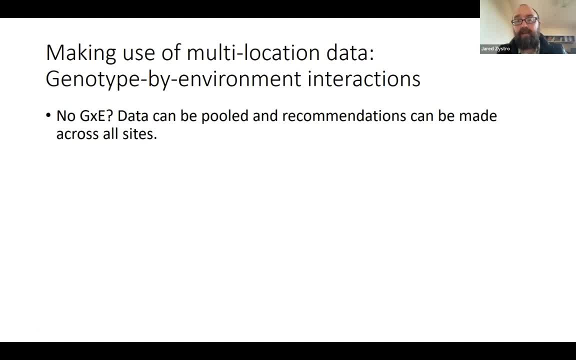 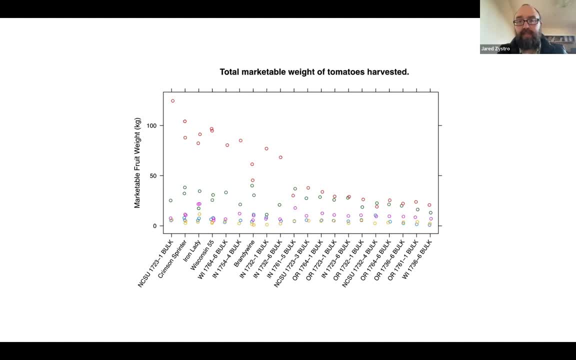 immediately. Yes, But you need to be aware of the differences in kind of the, the, the magnitude of the ratings in the different environments. So here's an example. This is just doing it visually. So this is from our one of our tomato breeding projects. 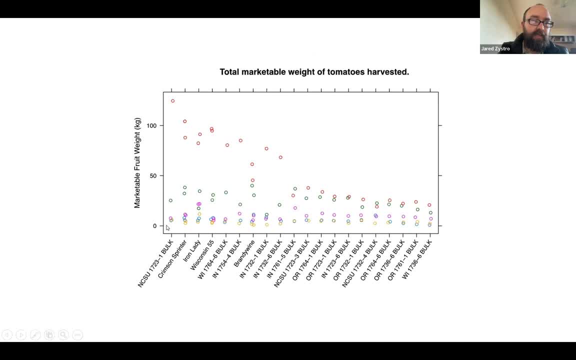 And this is looking at. looks like the tomato yield across five different environments here And you can see if we took averages it looks like the key got cut off, But there were The red there I think is grown at Purdue University. 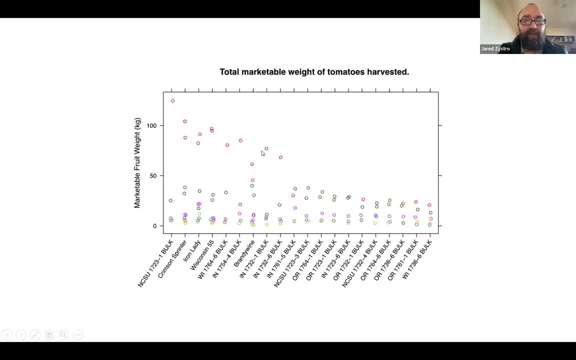 And if we took simple averages, Purdue's high yield across all of the varieties. really, if we just took an average it would be most influenced by those yields at Purdue versus some of the really poor yielding sites. But if we want to kind of look at it more in terms of ranking- a simple way to be able- 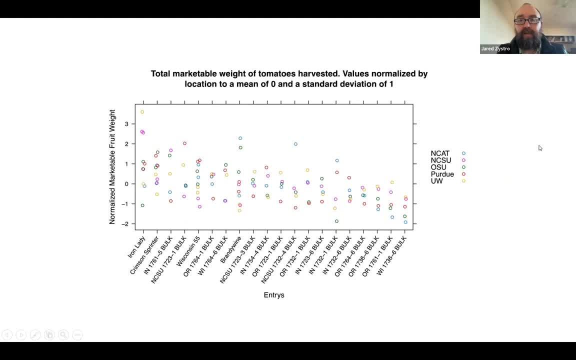 to compare things is just to normalize or standardize those values. So, in this case, same data, but what I did was I just normalized it to say that each the average of all of the varieties at each location. we're going to call a zero and the 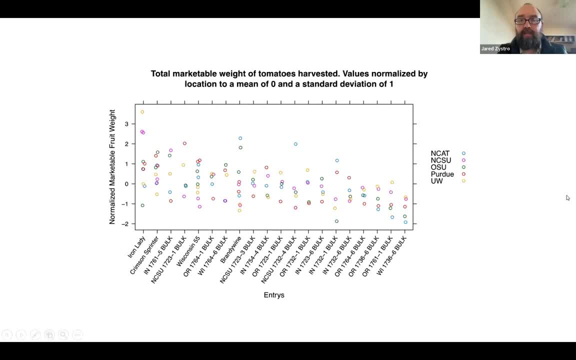 standard deviation around that we're going to set to be one and basically just transform all the numbers to make it so that the average at a given location is zero. the average and the standard deviation is one, And this basically lets us kind of see. OK, we can see here. Iron Lady. 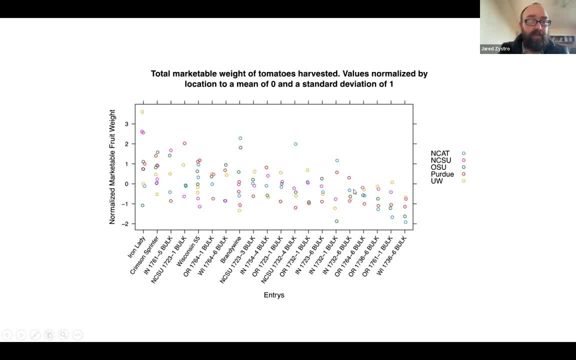 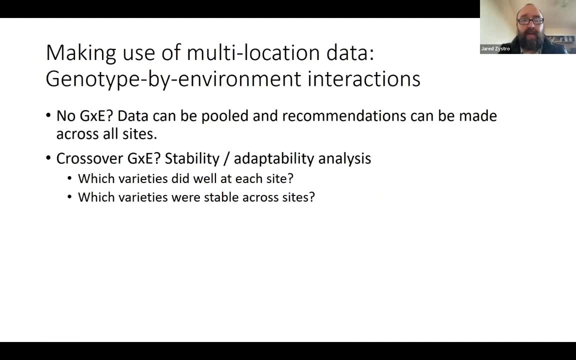 It was the best basically on average across the locations and but you can still see there's variation there. So if we have some genotype by environment interaction, then what do we? there's two things we can kind of look at. We can look at what we call stability or adaptability analysis. 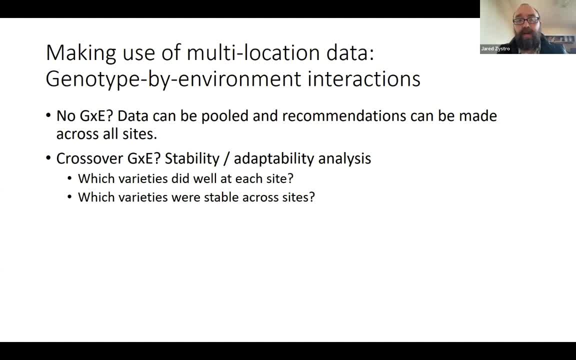 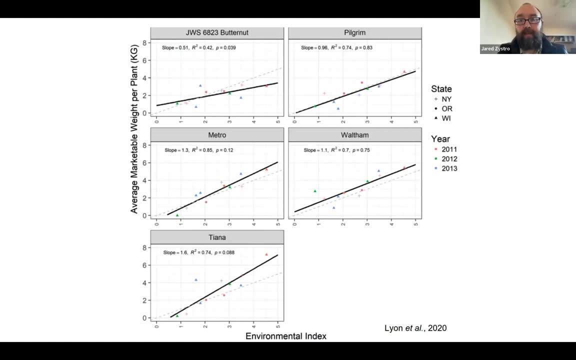 In other words, we can ask ourselves what varieties are doing especially well at each site And which varieties were pretty stable across all of the sites. This is from a paper by Alex Lyon. this is looking at adaptability analysis, very similar to stability analysis that you might see. 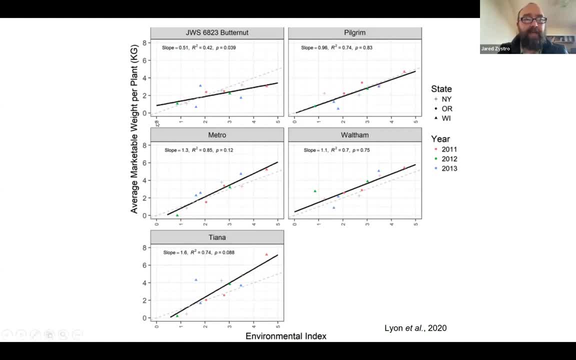 And basically what you do here is you arrange your environments from kind of what we might call lowest to highest performing. That's just based on the overall mean of the of whatever trait you're looking at. So, like going back to that tomato data we looked at earlier, 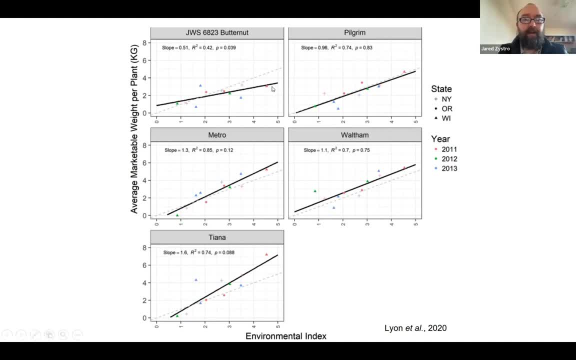 Purdue would have been kind of the highest performing environment. We put that on the far right-hand side here and the lowest ones on the left-hand side And then we basically draw a regression line to say as the varieties for given varieties. this is butternut squash. if you move to higher performing varieties, I mean higher performing environments. 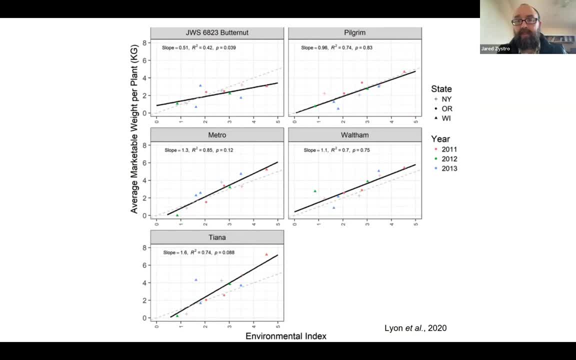 environments where the average performance of all the varieties that were grown in that environment was higher. as you move to these higher performing environments, how does that variety respond? And if this dotted line here, this dashed line, represents sort of the overall performance of all the varieties that were grown in all the environments? 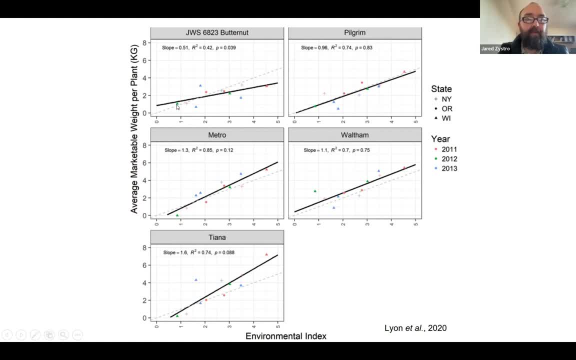 So as we move across the environments, the lowest performing environments, you have varieties down here, And as it moves up in terms of the performance of the environment, the varieties also go up. Now what the straight line here is looking at: how well did that individual variety respond? 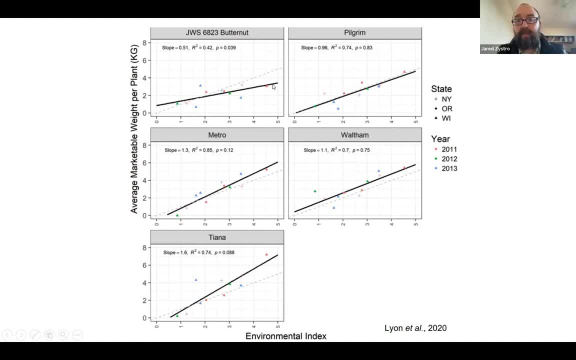 So a flatter line here means it's more stable. It means regardless of the on average that variety was, or that environment was kind of a poorer environment or if it was considered a better environment, the variety performs pretty stably. 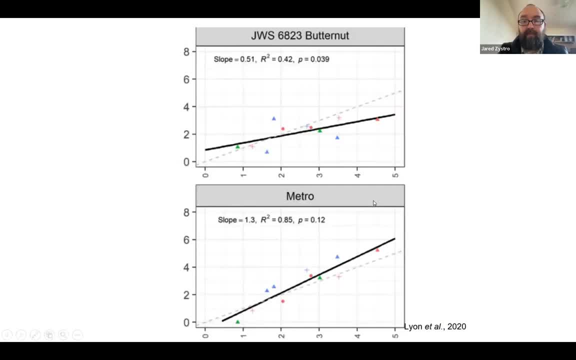 across all those environments versus. let me zoom in to just a couple of them here. If we compare these two metro here it really responds strongly to the environments, so that if you go up to the highest performing environments metro does really well but it really falls down at the kind of lower performing environments. 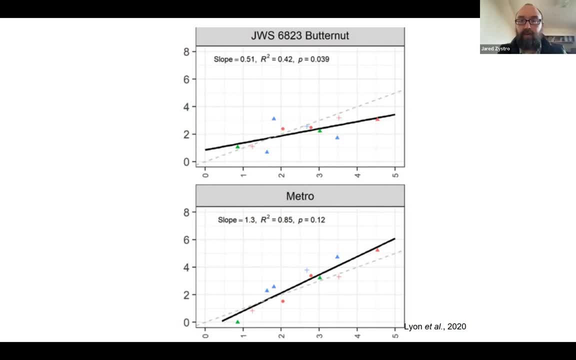 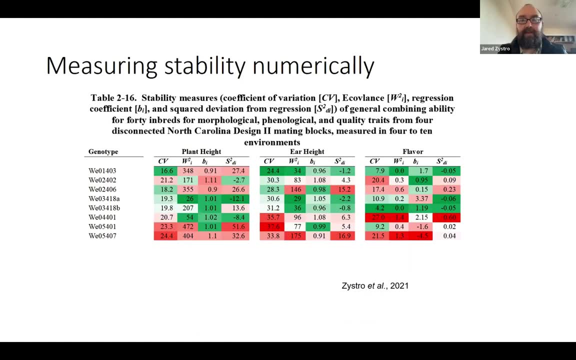 And so this is one that's really adaptable to those high performing environments, but not as stable. You can look at this stability. There's a lot of different ways to figure this out, and what you will learn is that those ways don't always produce the same results. 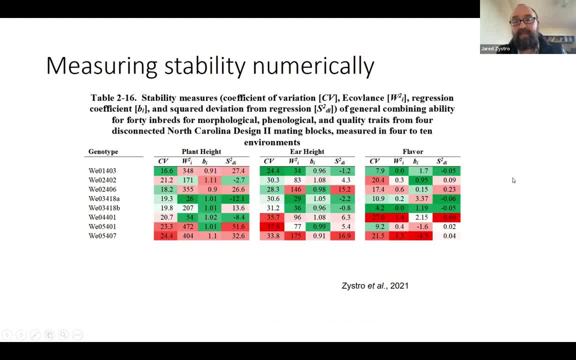 So this is just. there's like four different examples of different ways of measuring this idea of how stable the variety is across the different environments, And you can see that sometimes that you can see a consistent pattern of things that are stable or not, and sometimes not. 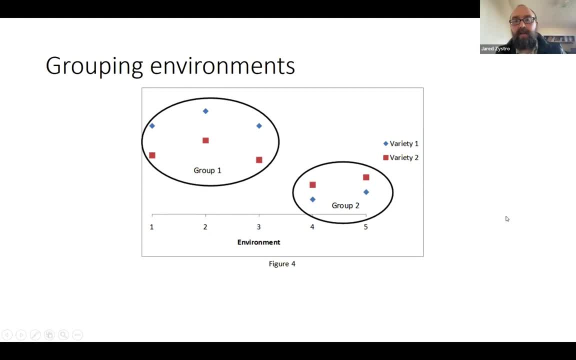 But another final piece here: Is that not, not, it's. sometimes you can actually look at environments and say, oh, we see a similar ranking of varieties in a group of environments Like in here. I mean, this is simplified down, but in this case, all of these environments in group one, here variety one performed better than variety two. 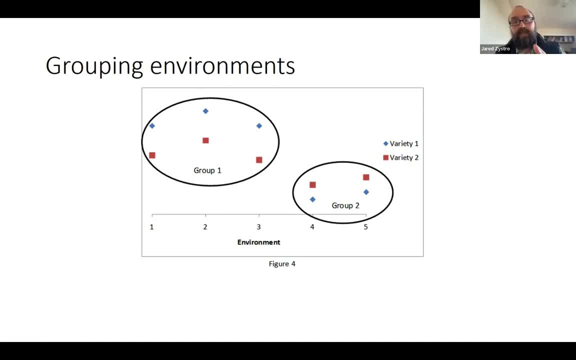 And if you expanded this out, it might be like similar ranking across many varieties in this group versus here, this group of environments over here on the right hand side. variety two did not perform or perform better than variety one. they flipped. 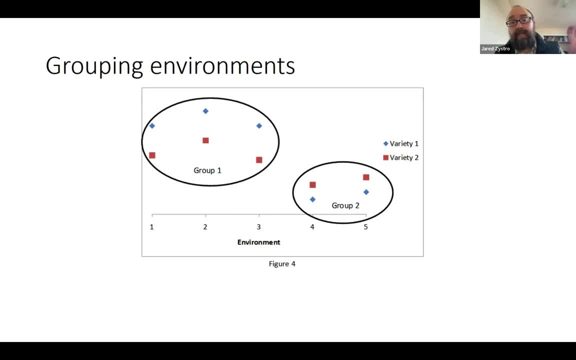 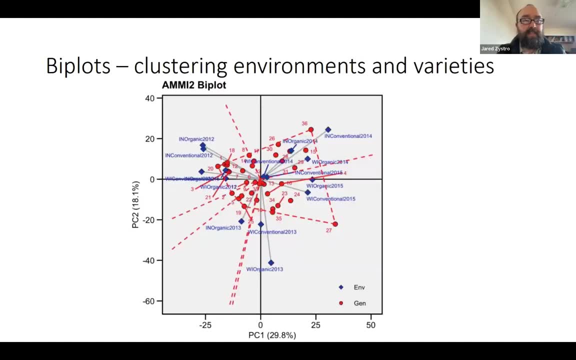 So when we talk about this, we talk about kind of populations of environments or mega environments, groups of environments where you're seeing the same performance. This is a way that's a bit cluttered with the amount of varieties and environments that we're looking at, but this is something called a biplot. 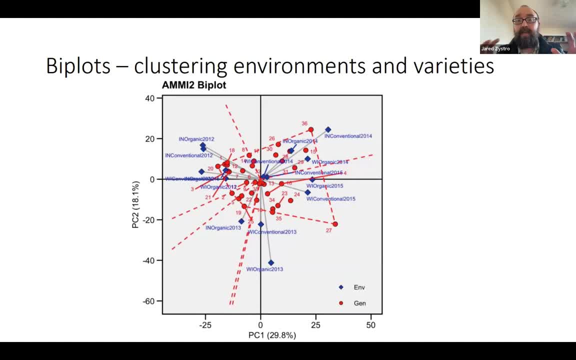 which is a way to sort of look at both environments and varieties together to see which varieties are doing well in which environments. And basically in this case the red dots are the varieties and the blue diamonds are the environments. and the closer that the varieties are to each other, the more alike those varieties are performing. and the closer those varieties are to a given environment, the better they perform in that environment. 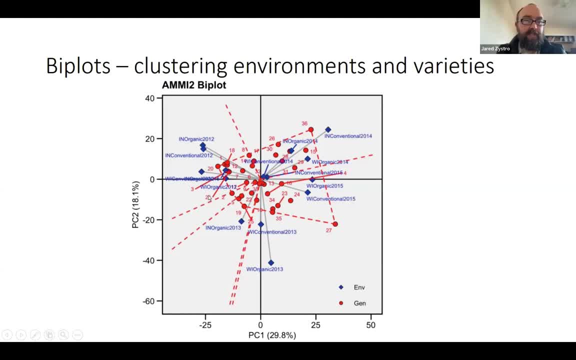 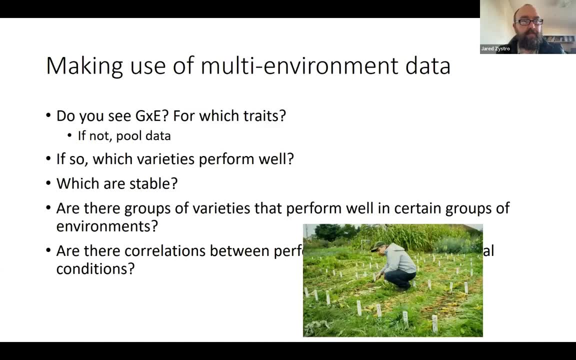 And so you can kind of start to see where certain environments cluster together, where certain varieties cluster together and which varieties cluster with what environments. So, just to wrap up, if you're making use of this multi-environment data questions, ask yourself again: are you seeing genotype by environment interactions? Which traits? Keep in mind that this is going to be different for different traits that you're looking at Some you may not see. 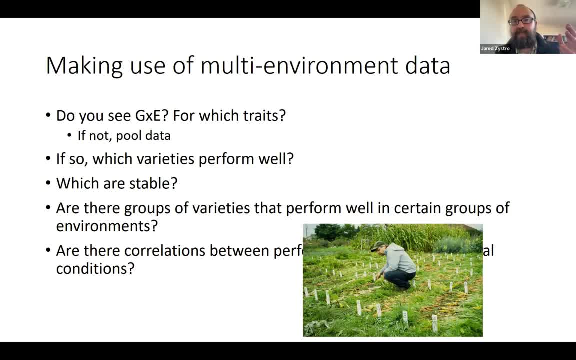 these kind of interactions between the environment and genotypes and some traits. you might see that, If you're seeing these genotype by environment interactions does which varieties are performing well across all environments, which ones are stable and which ones are not. 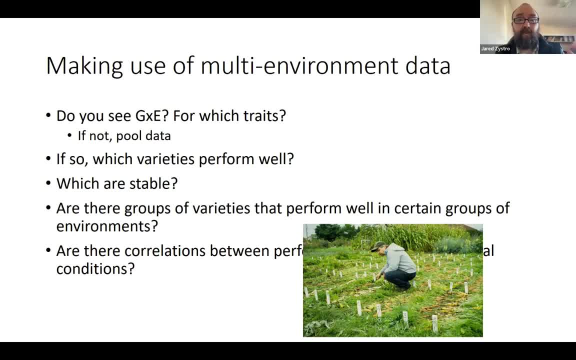 So again you're looking at: are there groups of varieties that are stable? are there groups of varieties that perform well in certain groups of environments? and then, circling all the way back to this question of why, are there correlations between performance in certain environmental conditions? 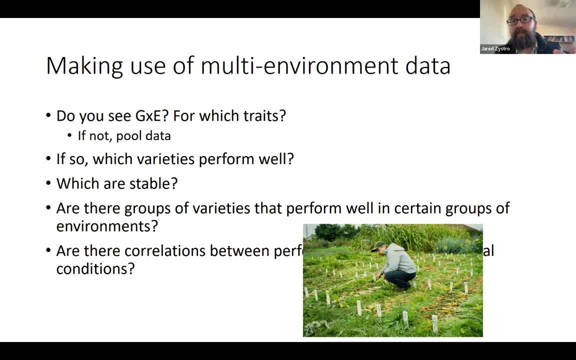 So if you did have those weather stations out there, did you collect some data that gives you some indication of, oh, all those environments that where we kind of in that group one of the cluster of environments, we're all wetter environments. all the ones in group two were drier environments. 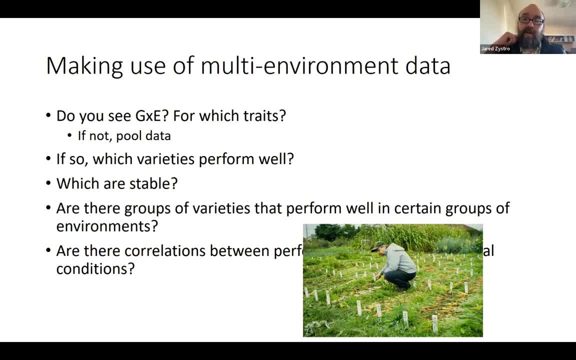 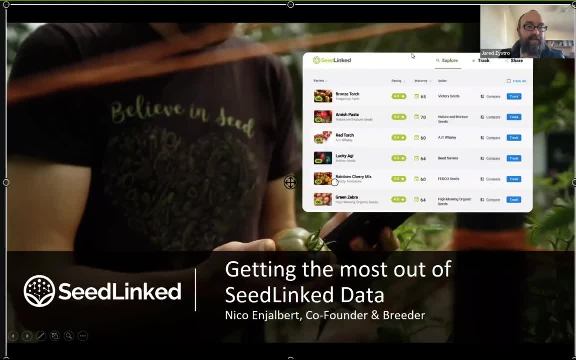 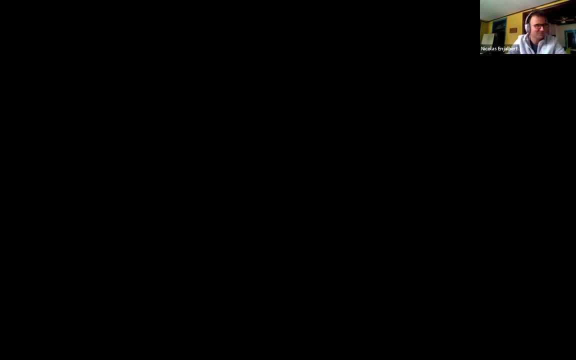 Things like that that you can start to answer when you have multi-location trials. All right, I'm going to pass it on to our last speaker. Hi everyone, Here is Nico Angel B at SeedLinked. I'm going to share my screen. 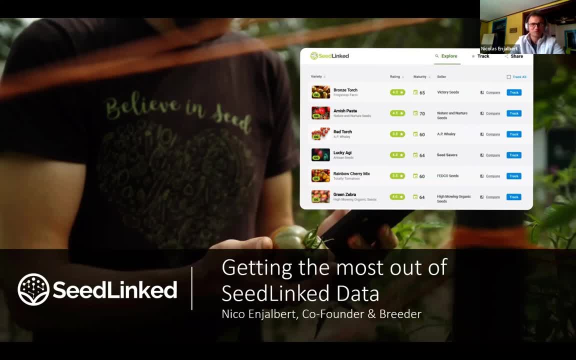 Thanks so much for having me Today. I'm going to go over how to get the most out of SeedLinked data, and thanks so much for all the presenters, especially Jared. at the end, too, I'm going to lay out the ground on a multi-location trial, as I'm going to cover the use of SeedLinked. 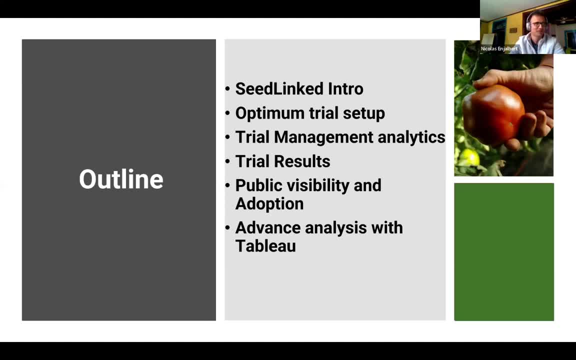 I'm going to give a quick intro for the ones who don't know, and how to build a trial to get the most out of the data with SeedLinked, and how to create engagement and then go over the results. and then I'm going to give a little tutorial on how to use another visualization software: Public Tableau. 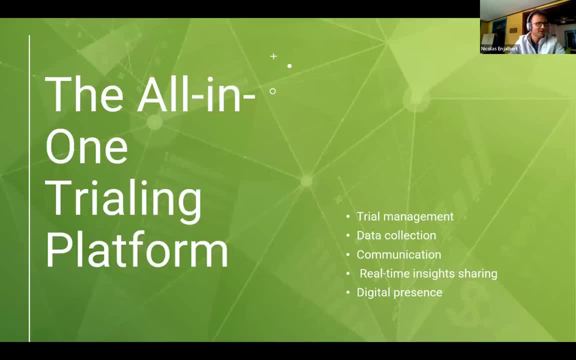 I use a lot. So, yeah, quickly SeedLinked is an all-in-one collaborative trialing platform that really allows to create collaborative trial engaging many growers- from trial setting all the way to data collection, communication, data sharing and so forth- at a really minimum cost. 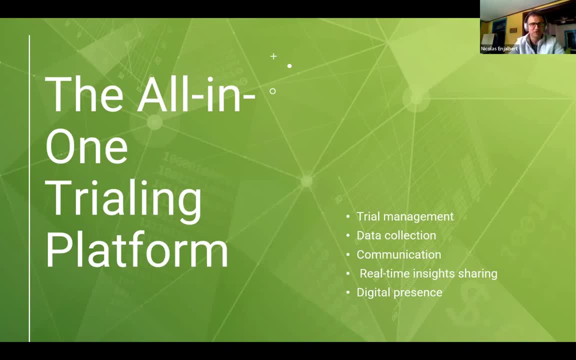 It's used to give capacity to people. Like Jared said, it can be very costly to do a multi-location trial And also Amber also mentioned on how to to give a structure to all, collect similar data and make meaningful insight, and how can. everyone has biased. 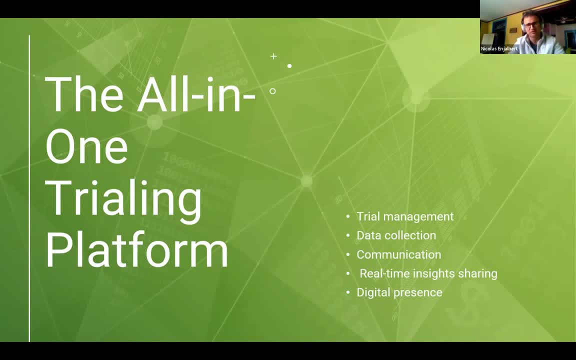 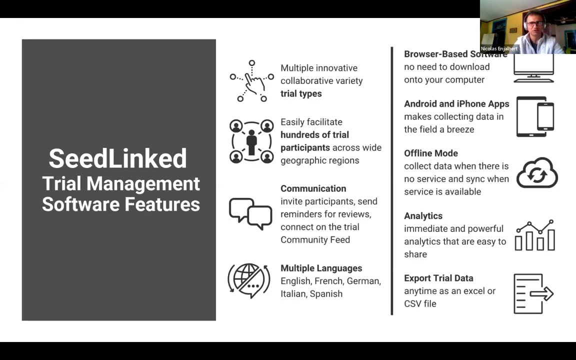 and so why collaborative trialing is really useful in this case to give information for multiple people, multiple place, And so C-Linked has multiple feature, multiple trial type for different statistical design, many feature to really remove all the barrier of collaborative trialing. 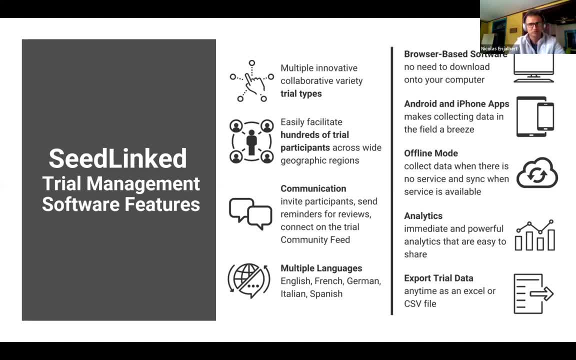 embedded communication multi-language. Also, it's rather in cloud base and app in iPhone, So you don't need to have your own database and system. You can be all store in the cloud and C-Linked and it has its own simple analytics embedded. 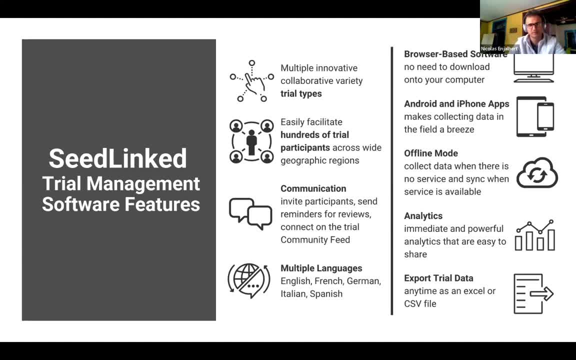 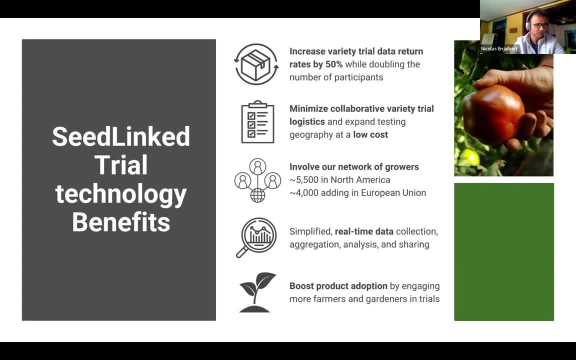 but also you can expose the data and do further analysis, And you have offline mode as well. if you don't have capacity- and, yes, benefit- using the platform is really true- You remove. you have all the, I think, trying to have all the advantage of collaborative. 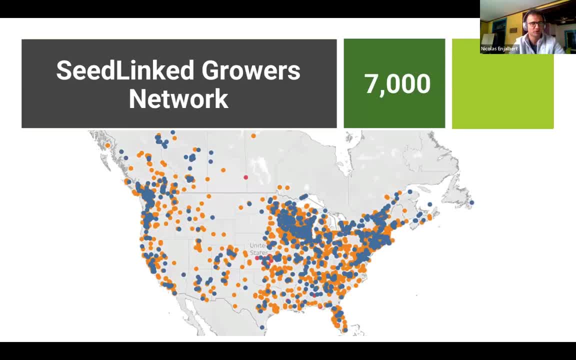 trialing and trying to remove is a barrier of it. And also we can leverage as C-Linked has been used by many organization and we have a large network of growth that can be tabbed to if you don't have the network yet to trial. 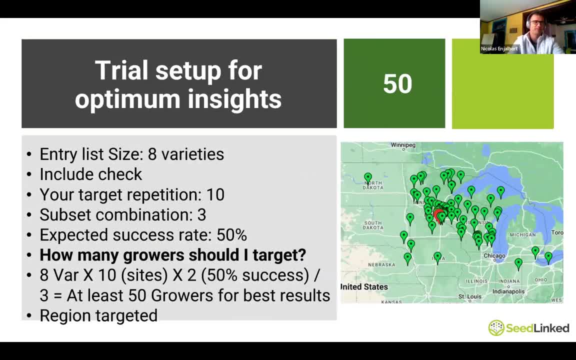 especially in the US, And so now I just want to lay the ground on on how to make to get the most data and to get the most the best decision out of the data, using collaborative trialing, collaborative breeding, And first is depending on your entry. 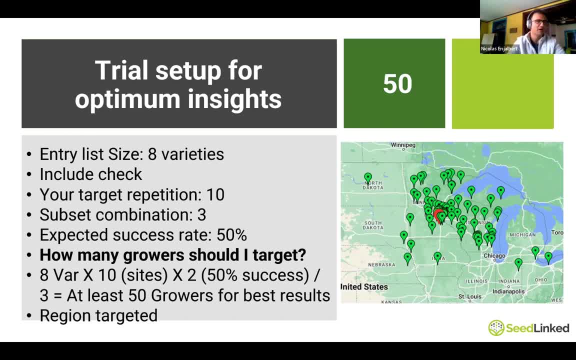 and you check what. how much farmer do you need to get enough repetition and enough reliable data and to calculate quickly as this? you really need to know what's potential success rate as what you do- collaborative breeding or citizen science. 40, 50% perception rate is very high and it's good. 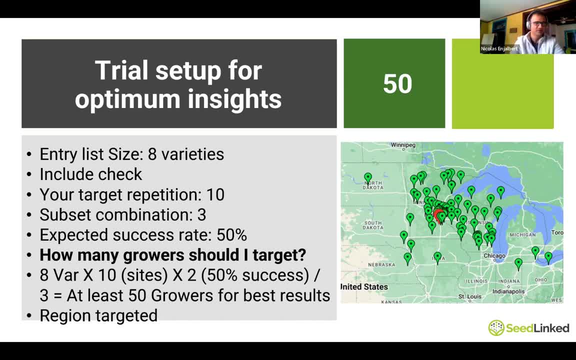 but you have to take this into account. take into account also how many variety each borer is going to take. in this case, Let's say three out of eight, and then give you kind of a target of number of grower to get really, really deep data. 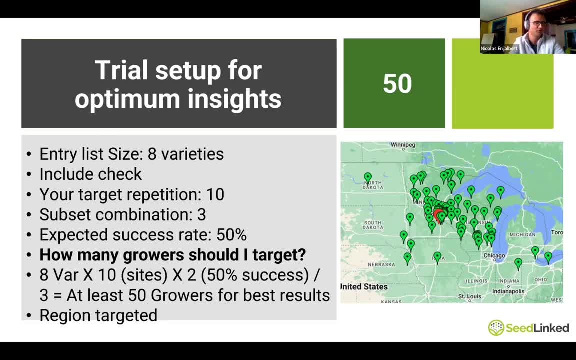 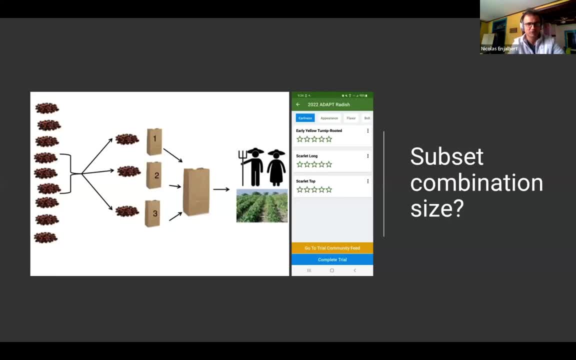 And then defining what region do you want to focus, to find the grower or to invite grower. Here's a quick an example of one of statistical modeling in C-Linked triadic where you can kind of a combination. let's say, here I have nine variety. 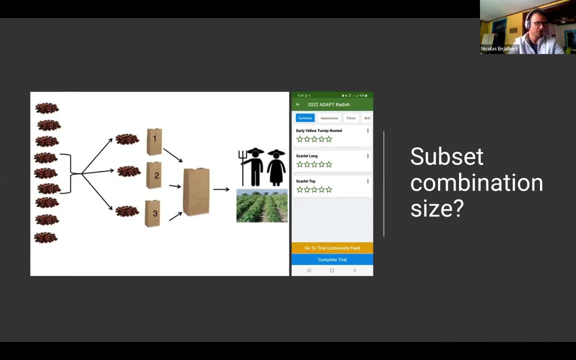 and you can decide to send three to each grower and C-Linked. do that automatically, Create automatically those random combination. But if you increase, we can do three out of nine, you can do four out of nine, obviously as the combination increase. 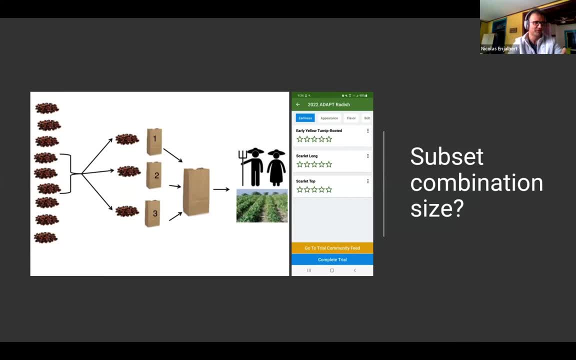 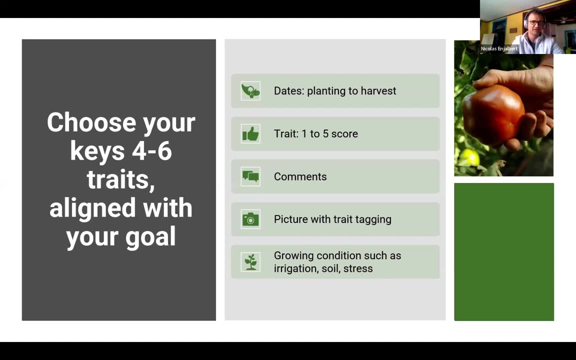 you get more repetition, but also grower might give you less data because if you overwhelm with too many varieties, it might not be as engaged. Also, it's very important, like the past presenter mentioned, to frame your trait and what you ask, along with your breeding goal. 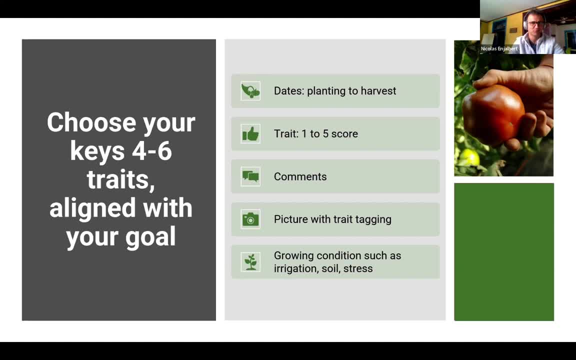 and not ask too much to your grower again, to get more engagement, Better data and then make a better decision. And so you can pick your trait in C-Linked. so it's also a default information that are asked like: dates, comments, picture, growing condition. 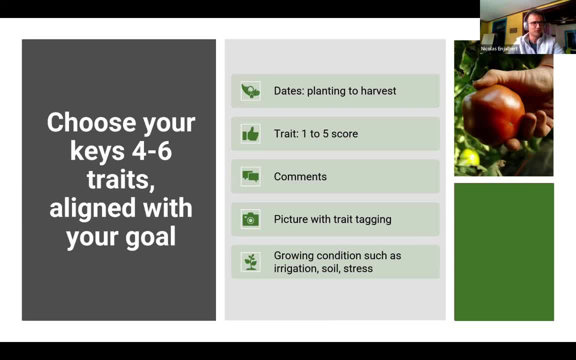 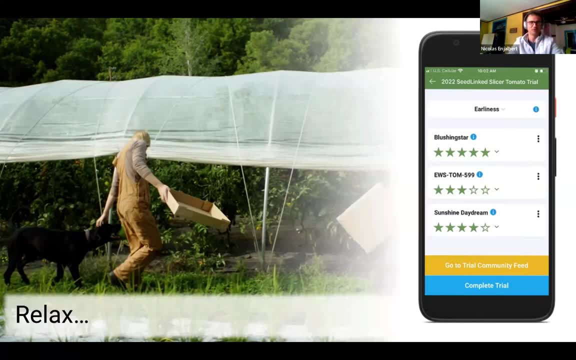 as meant past presenter mentioned. those are really important to really put into context of score and C-Linked. do that all in the app when you invite your grower And so when you set up all this and you send the seed, it's time to relax a little bit. 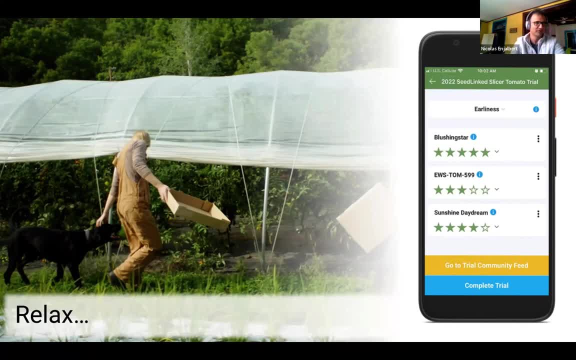 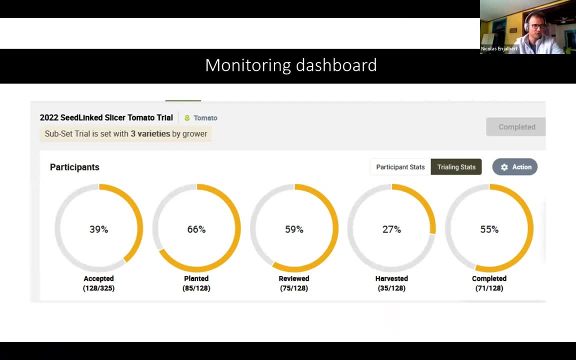 and really lets the grower grow and send amazing information. but also we have dashboard in C-Linked that allow you to track progress, how many planted, how many review, and you can send automatic reminders that you have push notification coming on their phone. 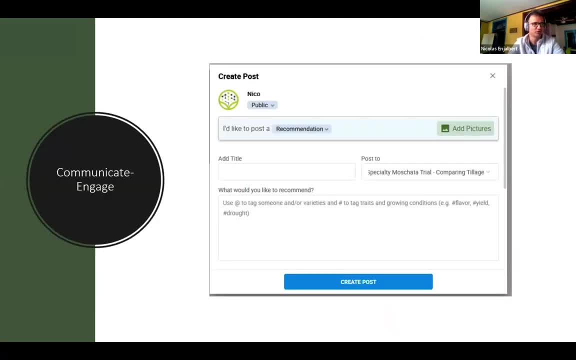 And also there's an embedded feed or communication where you can send, within each trial, as almost as your Facebook group. you can send information like: oh, it's time to review. You can send a picture and you automatically land on their phone. 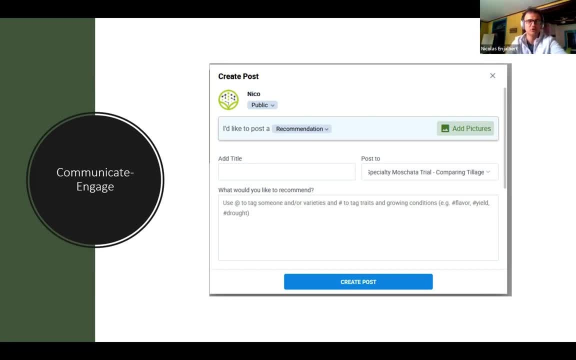 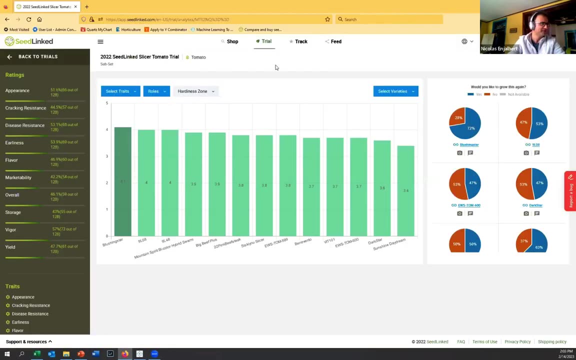 And also grower, can engage in between to create a community and ask, question and share, which create engagement Again. the more engagement you create within your group, the more data, the better decision you can take. And now I just want to dive. 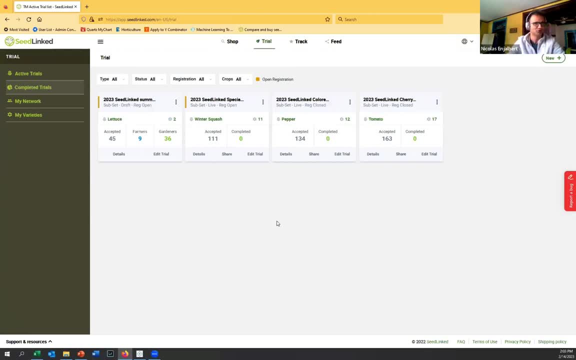 and using directly C-Linked here. This is a trial manager account. I can see here is a trial. I can create new trial. Here's my new trial for this year. You can see I have a lot of grower from 160, 130 invited. 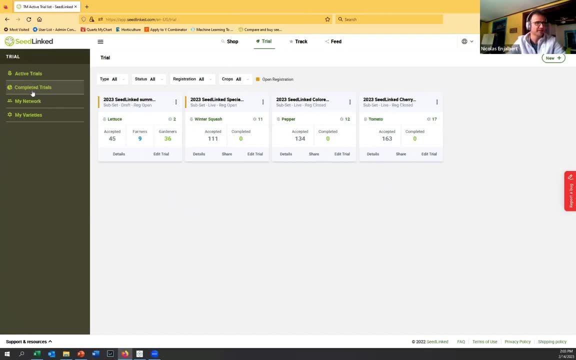 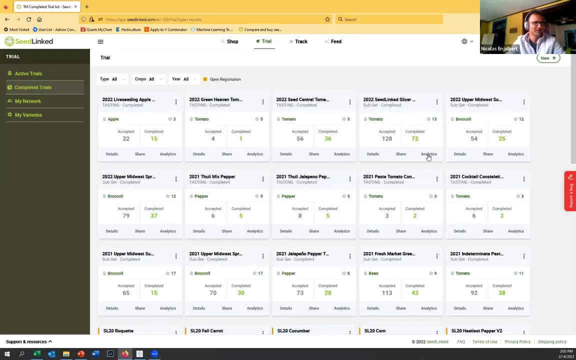 For today's webinar. I'm just going to focus on looking at the data, So I'm going to take a completed trial here Again. I'm going to stay in as a tomato, as I guess we all talk about tomato today, but 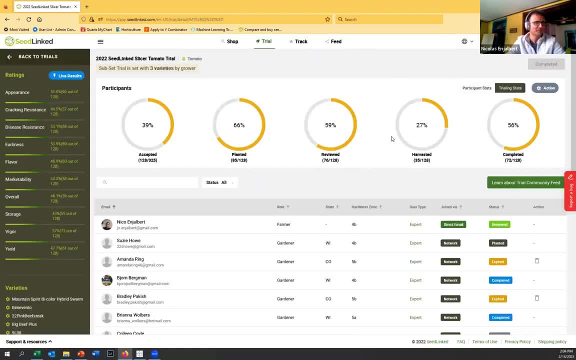 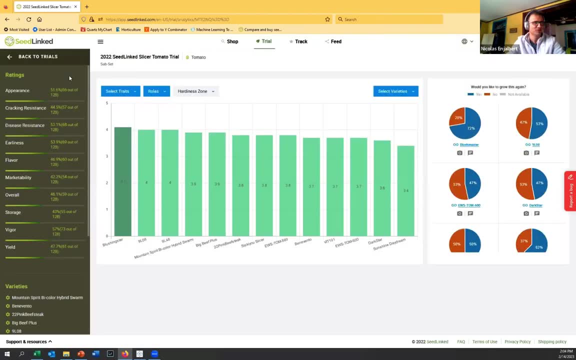 and so here's the again the data. you can see the percentage of participation At any given time, you can see live results coming from all your grower and you don't have to wait the end to make decision. It's all here. 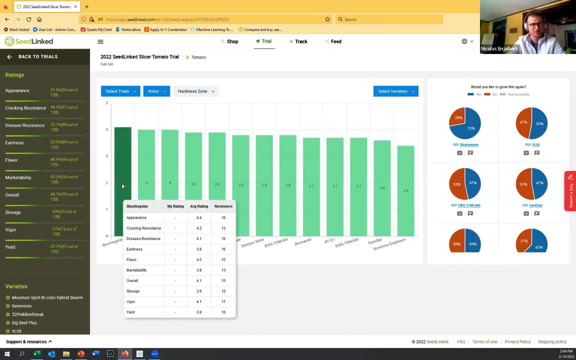 And so here I have all my tomato variety. I had 120 grower with a more than 50% participation rate And you can see for each grower you can see the traits or for each variety and how many grower have sent a review for each grower. 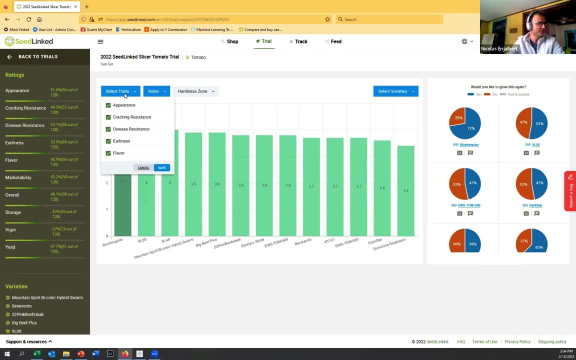 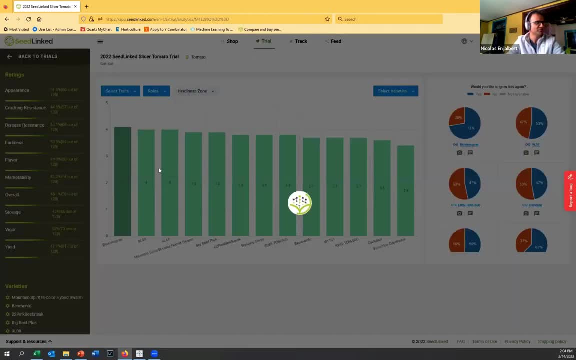 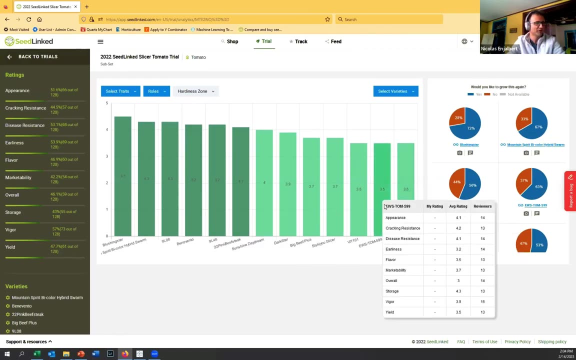 For each variety. you can quickly looking at different traits here. If I want to look at flavor, for example, you can see very different response. Look at, for example, those one bred really for a small storage And if, like here here, I can change again. 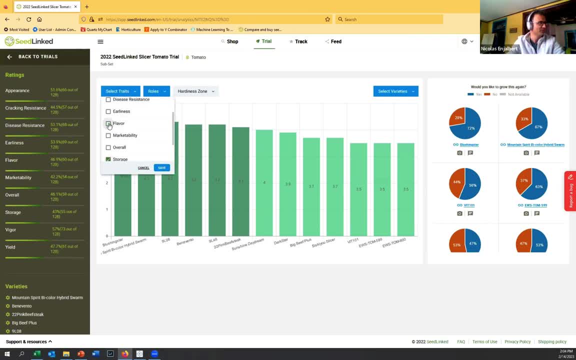 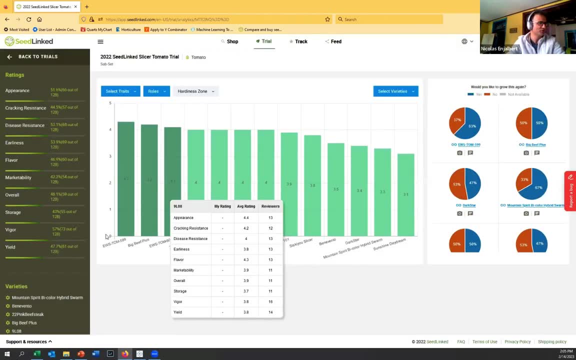 depending on your breeding goal, but you can see drastic change in order depending on which trait you pick. You can also, as we engage a lot of master gardener, you can. okay, I want only to look at farmer data, maybe. 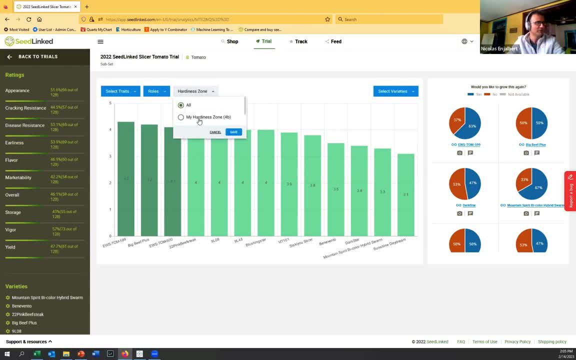 And also you can. okay, I want to look at only my Ardena zone or all Ardena zone. So that's more of the scoring part of seedlings. But I think, oh, and here big beef plus was a check. 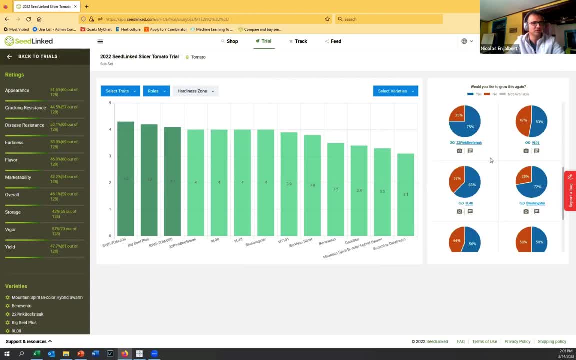 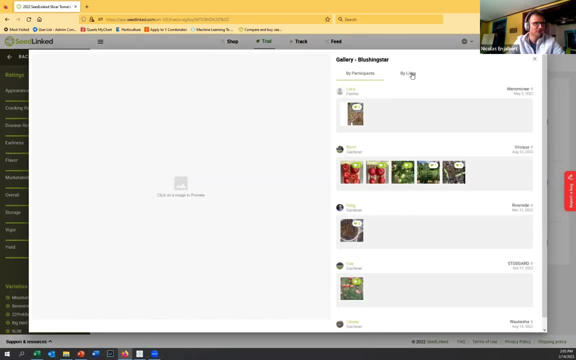 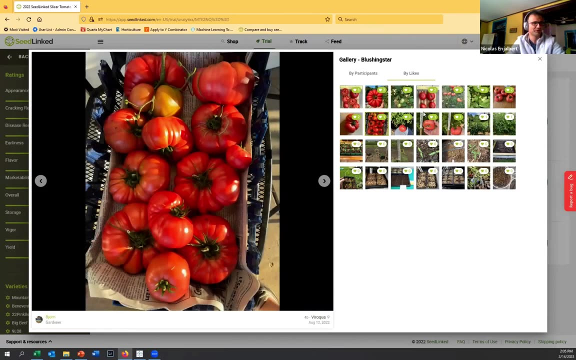 I think what is also fascinating to see here- let's say one of the best blushing star- is you also have picture from everyone and you can look at pictures sorted by, like you have a visual representation from many sites where you can see when the picture is taken, where by who, 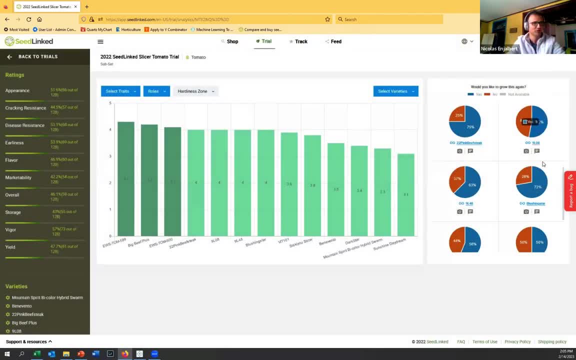 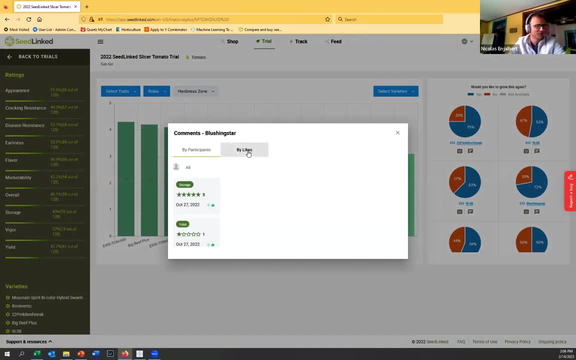 And so you have a visual story by all your grower. and also, as mentioned before, you have dozen and dozen of comments tagged by traits. So here you have the traits and you have comment and review from. you can see the long list. This is a power also of collaborative trialing. 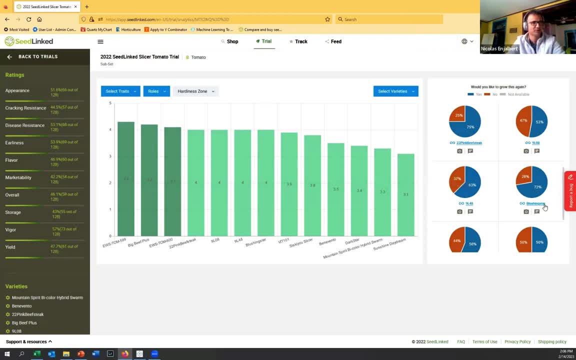 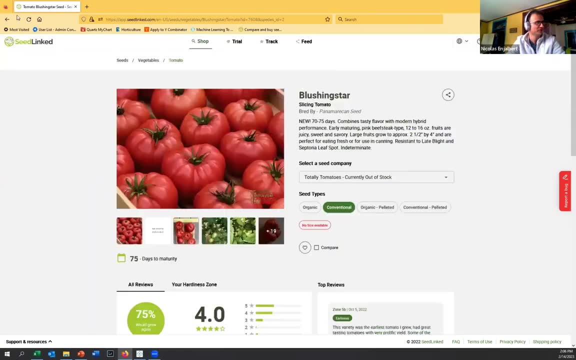 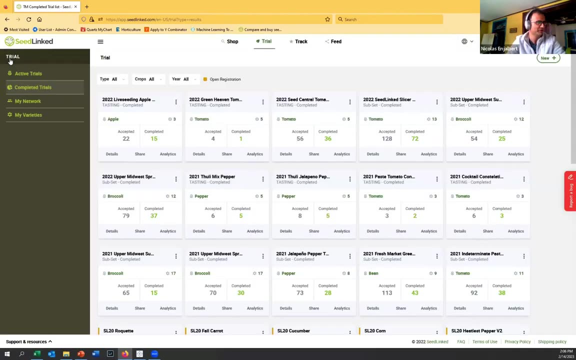 And then, if you decide, you can also make this data public and then all this information can be visible in seedling by other as well. And I think another piece I wanted to mention here: it's fully collaborative and you can also share here, Like maybe you work with other colleague. 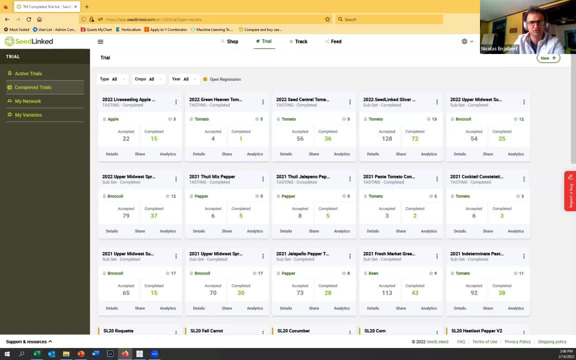 you work maybe with- I'm going to post here as a link here and just to give you an idea how we look- maybe other breeder or the people and they can have a view of the live visual trial. You don't, they don't need to. 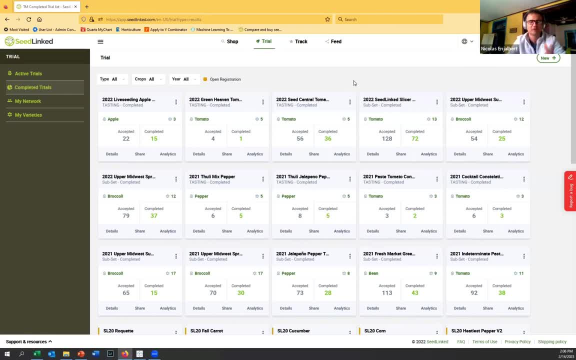 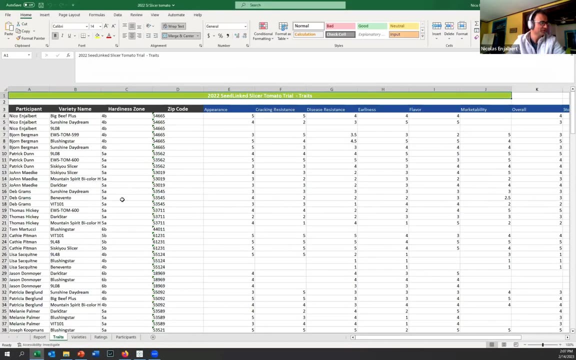 you don't need to wait 12 months to get it back or it's really live and you can make a quickly decision. So now I want to go over exporting data. You can export the data right away here And then you come in different format for you. 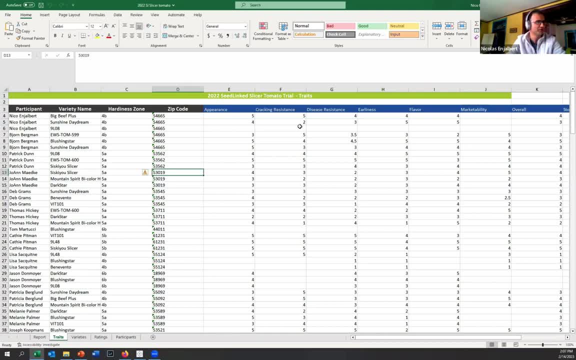 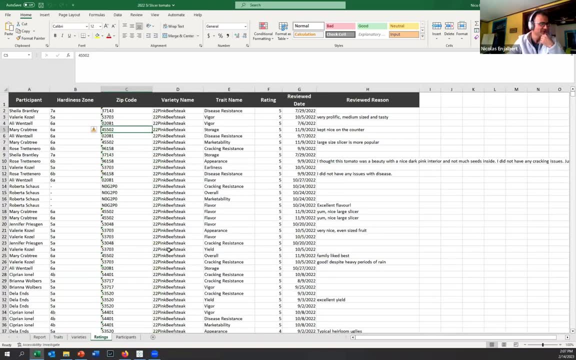 Like, see all the different sites, hardiness zones, zip code and also review. If you want to run further analysis, you can look also at date comments, and here's a tab with a row. data is From here. I'm going to try to quickly show a little bit. 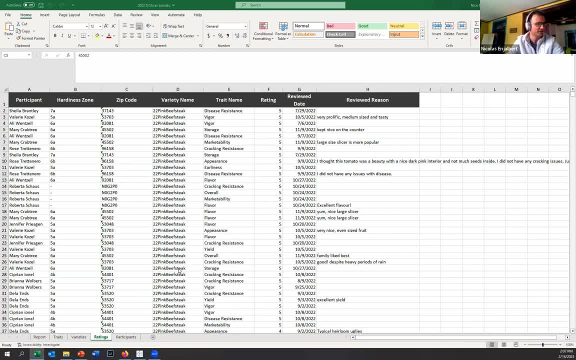 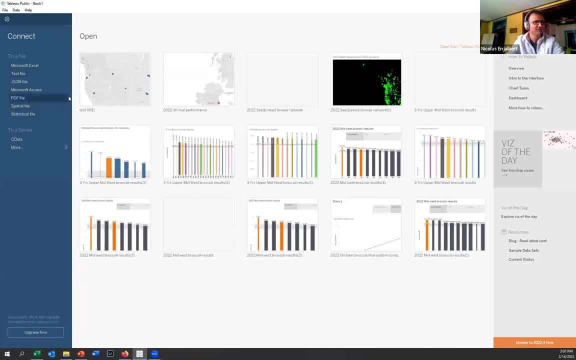 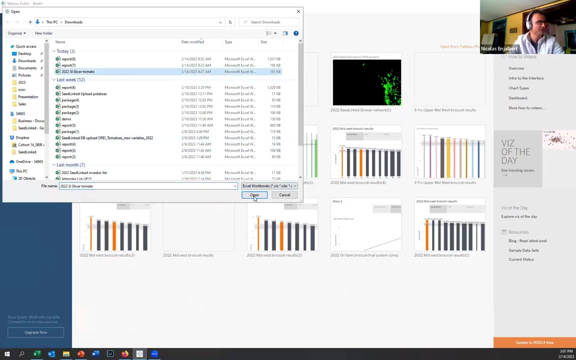 the use of Tableau, using just a raw data here out of seed link to do more further visual analysis. So this is Tableau public. it's free to download. It allows you to use multiple files here. I'm just going to take the file I just exported. 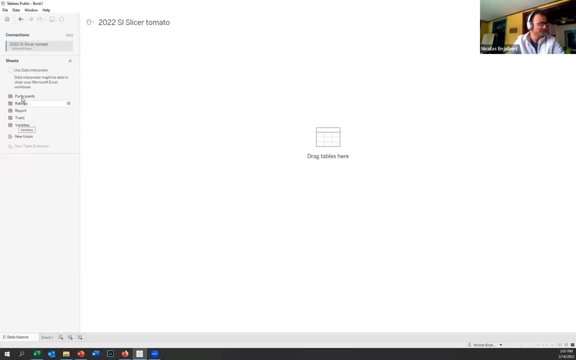 I open it and here is my different tab. It's Tableau is really intuitive and you just drag and drop, So I want to use the rating tab here, And here you have different format. You have the sheet where here is to build your visualization. 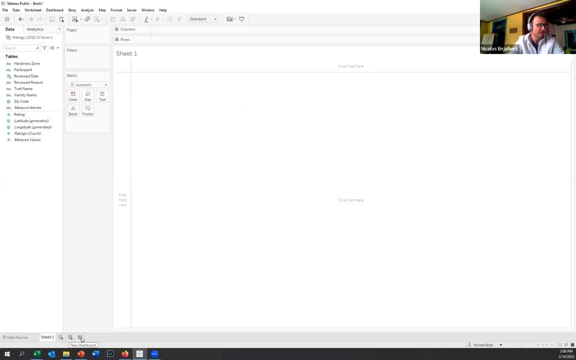 And then you have dashboard, which is to make it nice, And then story is to build a story of data that you can share, And so let's start with a quick visualization, So from seed link data, you can instantly you have all the localization. 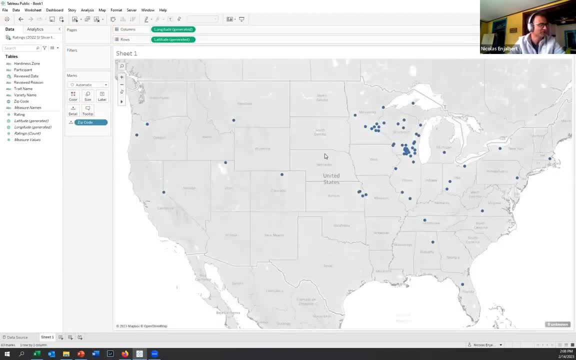 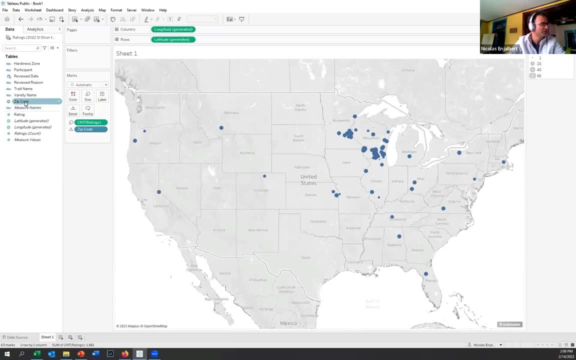 So those were all the site. I just drag the zip code. Tableau recognized automatically. You can put even the volume of data by site. If you want, you can even drag in the filter all the variety, and you can show filter here, where then you can color code. 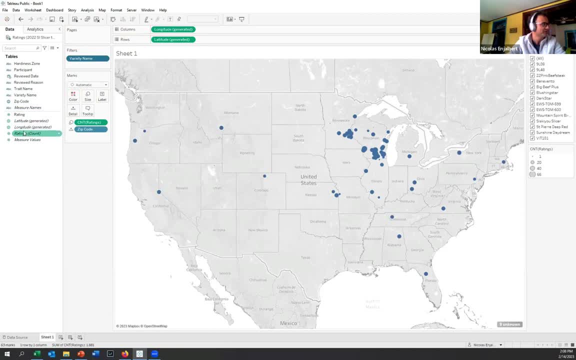 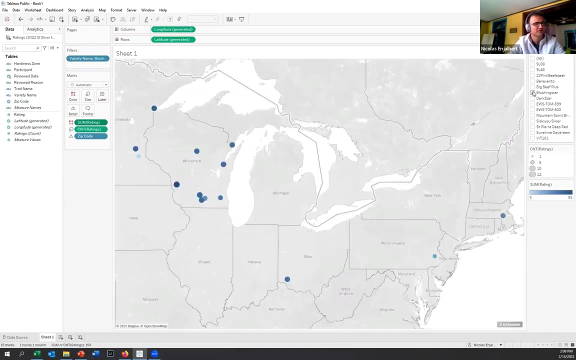 by traits or, I guess, by rating performance, And so you can put the rating into an average and you can see. and then you can look at different variety. Let's say blushing star, where it was tested and where it did perform well. 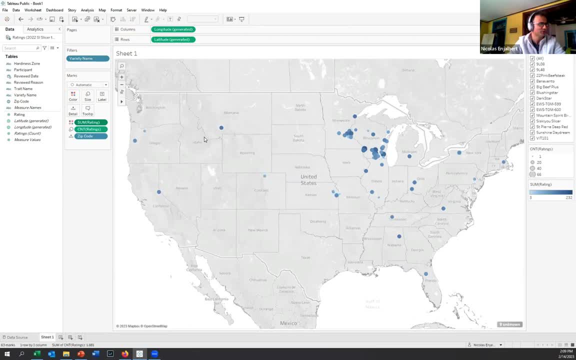 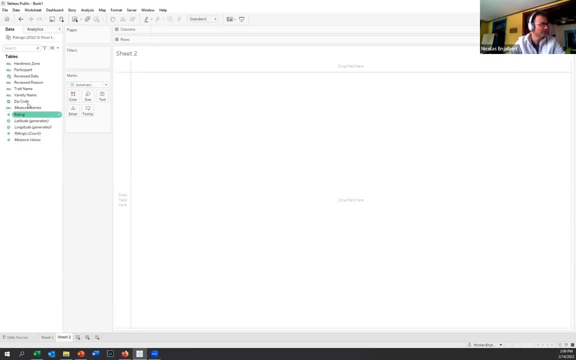 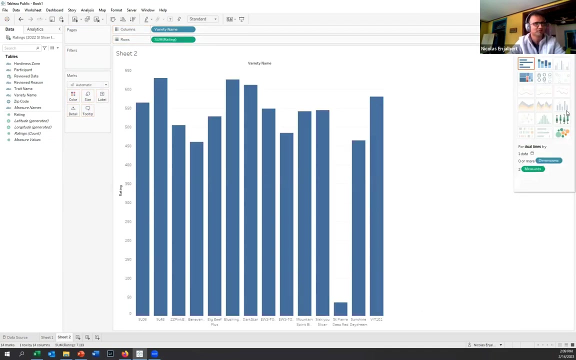 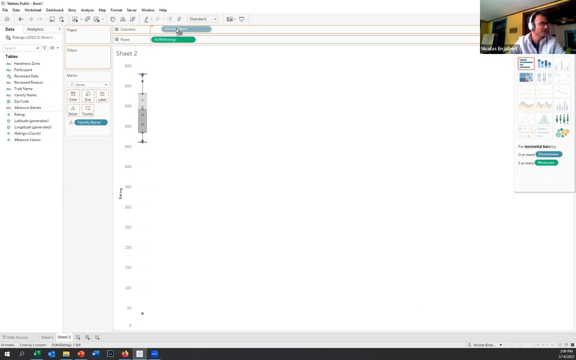 or where it did not perform well very quickly. So that's a really nice way to look at quickly data. You can also look at more viability of the data. that can be interesting. You can here you have different visualization And so you can looking at variability of data by site. 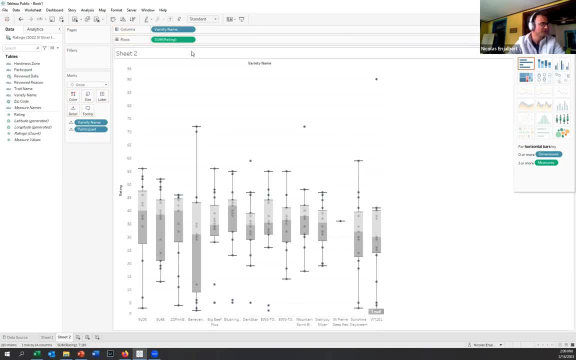 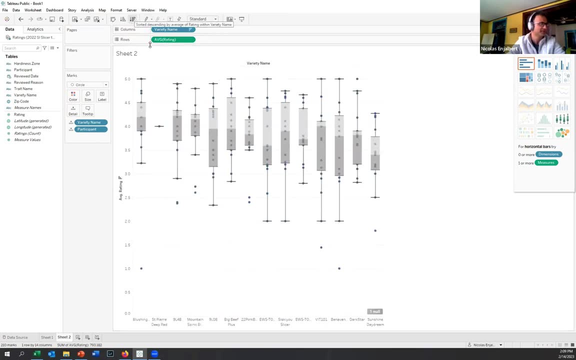 which is: let's drag and drop the participant number here And let's put on average data here So quickly. here you see also viability of data, certain variety of more spread than other, more stable than other. You can even only remove one data. you can. 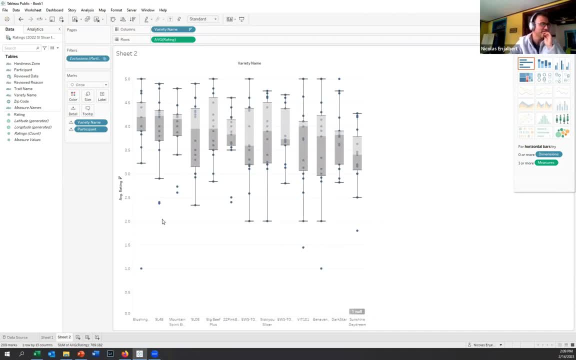 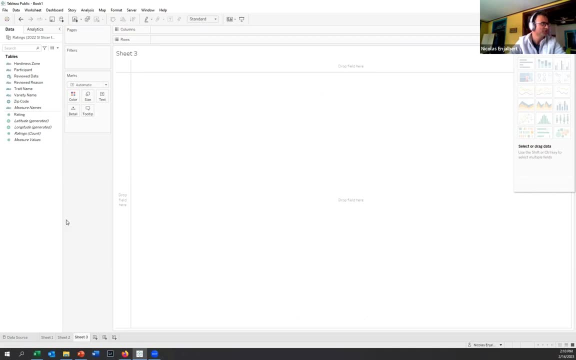 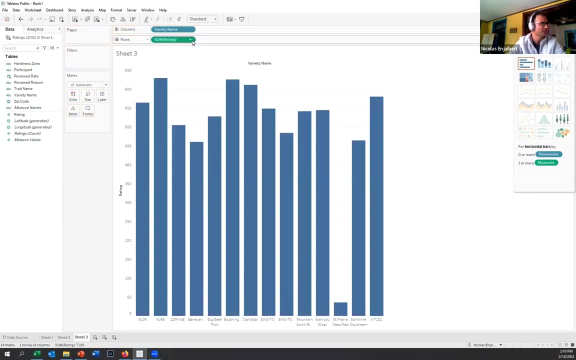 So that gives you a really quick, nice visualization of the spread of data. If you want to see outlier and so forth- And I think the last one I use quite a bit as a basic chart where I have my variety like this, this is going to be the average of the data I can sort. 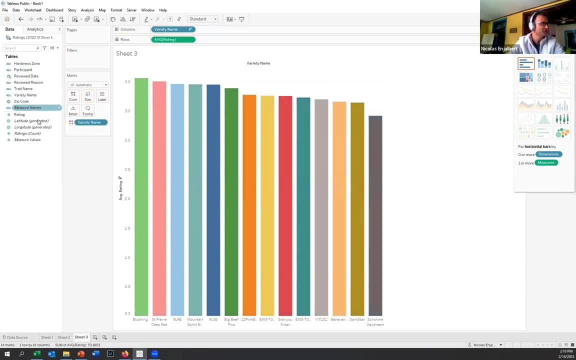 You can color code your variety, You can. okay, we're going to put the data on top here just to see. There's an average value And there's quick basic analytics here I can put an average with a 95% confidence interval. 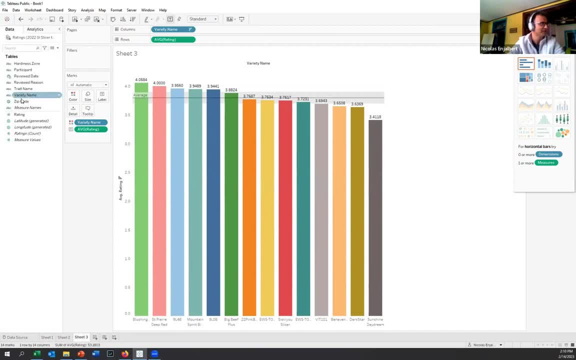 That's very easy to do. There's clusters, there's many different embedded things you can do. You can also put it as mentioned, Jerry. you can transform the data quickly with a quick calculation. For example, I want to look at data in percent of total. 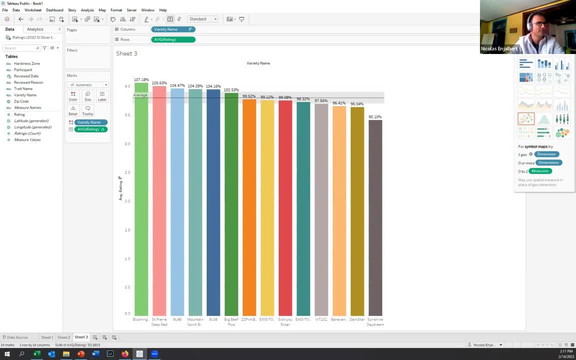 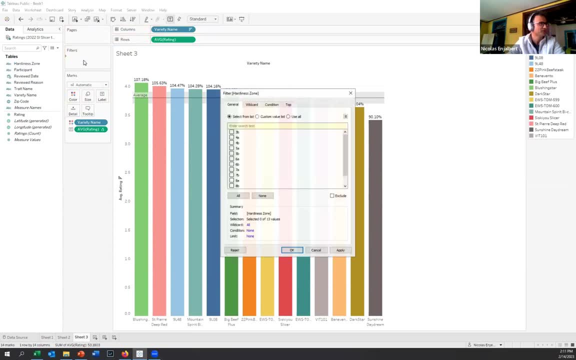 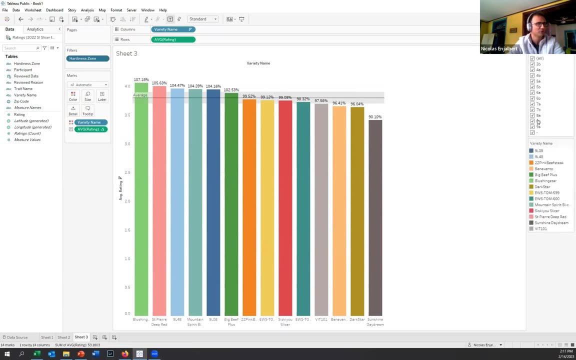 So deviation from the mean. I like to do that And then here you can looking, you can add: I have hardiness zone, And so I like to add hardiness zone as a filter. this way, You can look at different location, and how is this data performed? 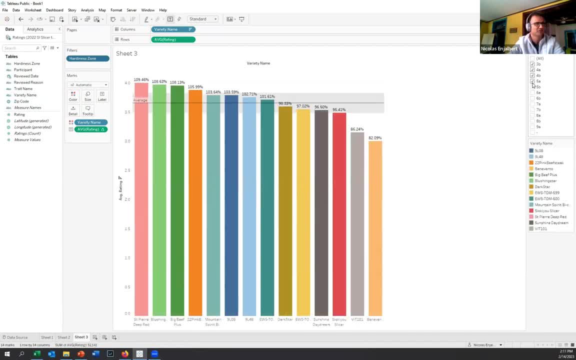 For example, just looking at the smaller hardiness zone, and you will automatically compute the result for you. And you can do the same with traits. So you can play with traits here. And so here you can. now I just for me. 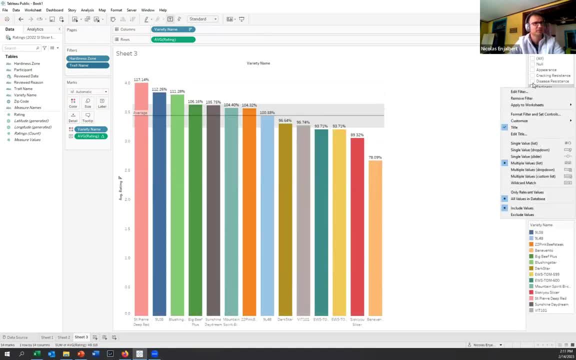 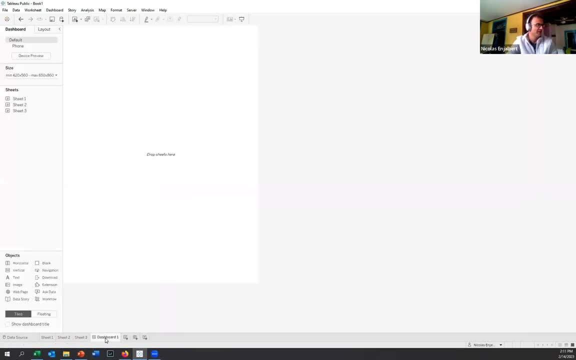 I want the best yields- early-ness, for example, and disease, And then you can quickly see as variety And then from here you can create quickly a nice story of the data that you can share with colleague and with other or, and so I create a dashboard where I'm going to create. 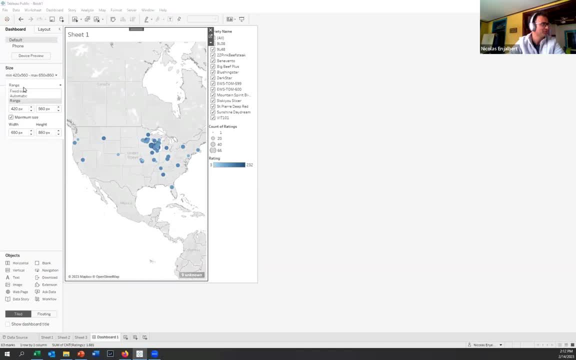 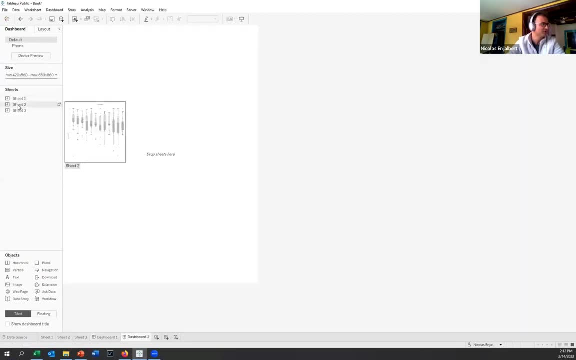 create a story. So let's say we want to show the map of the data and performance. That's going to be one nice slide. Another one's going to be- let's, the variability of the data. I made it auto fit here. 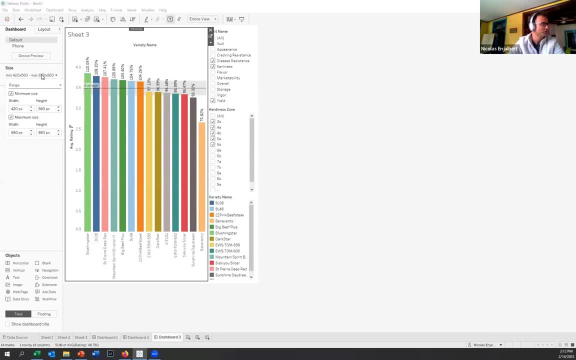 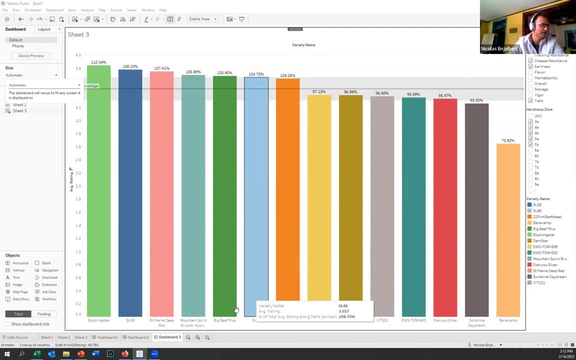 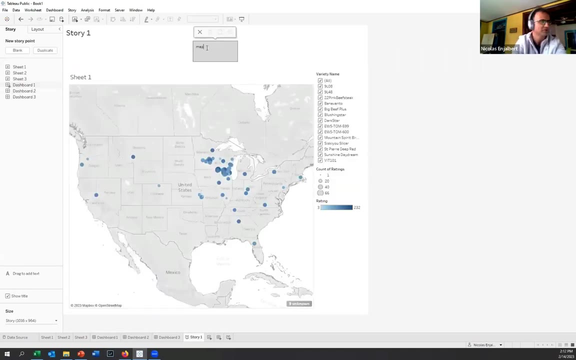 And the last one's going to be the overall performance to play here, And so those are kind of my nice three dashboard And then I can create a story where I can again draft is going to be my map and my variability and my overall performance. 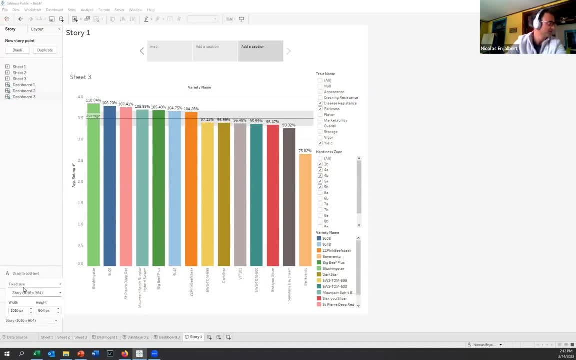 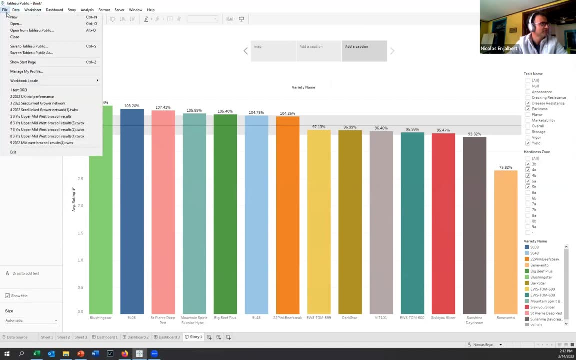 And I like to make everything looks nice. And then you have an account. I'm just you can really quickly save into the cloud. This is, let's say, test, just to give you a flavor of how we're going to look, And then I'm going to share this in the chat for you to see. 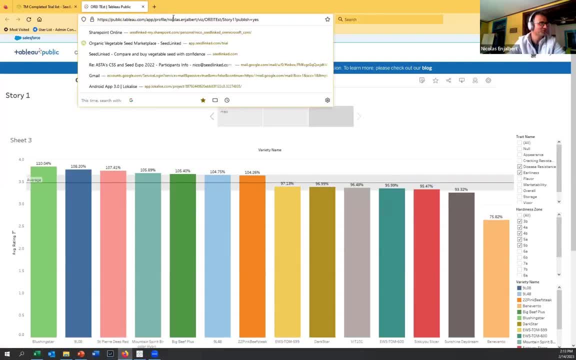 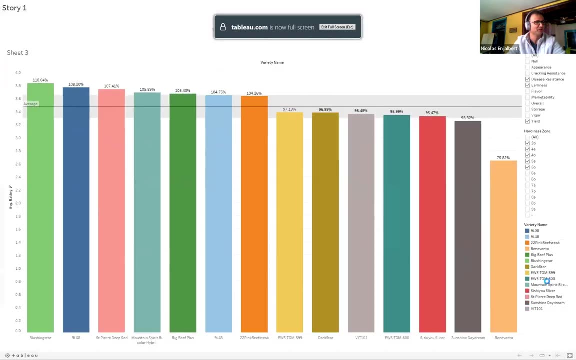 And yeah, that's kind of what I wanted to share. I know we are behind in time so I'm going to stop here, but I'm going to put this link in the chat here quickly for you to see as an example, And with Tableau, you can put in full screen. 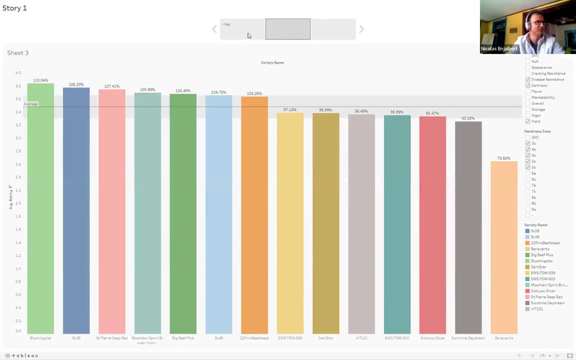 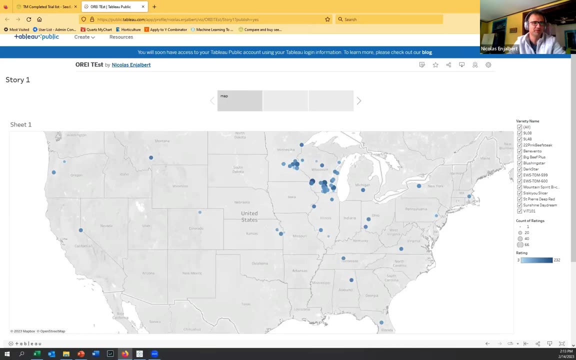 and really play with the data, And everyone can receive this, can play with the data, So it's very useful. So, yeah, that's it. She's wrapping up how to get them all set up. Ceiling can make better decision, So here we are. 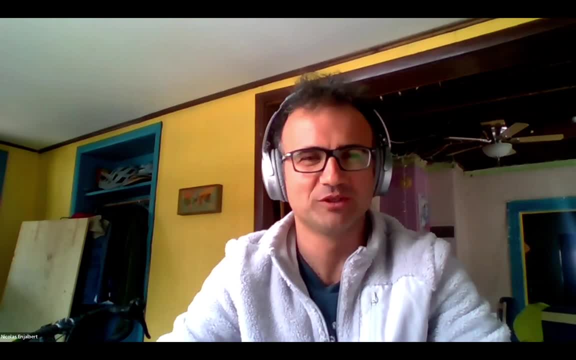 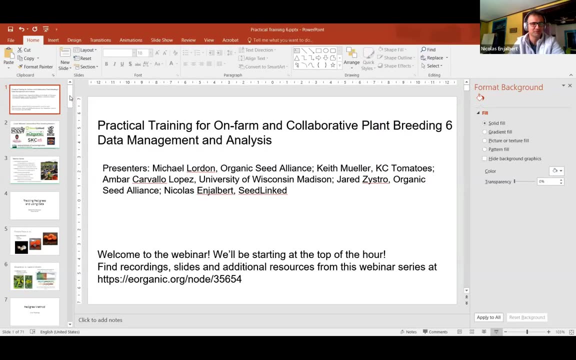 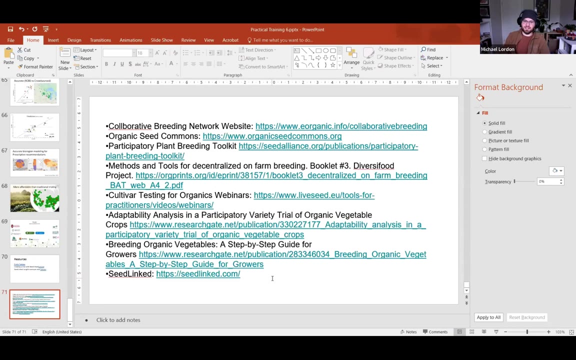 Always a time that just a couple of the tool in your toolbox to run collaborative trialing and make your breeding or trial program more efficient. Thank you so much, Miko. Thank you Ann, bar and Keith and jared- uh, everybody for your presentations. that was really cool. uh, nico, that software is. 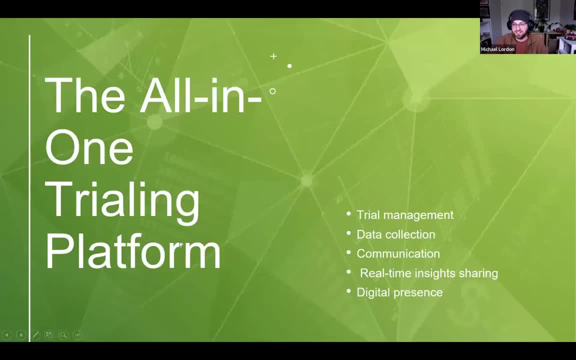 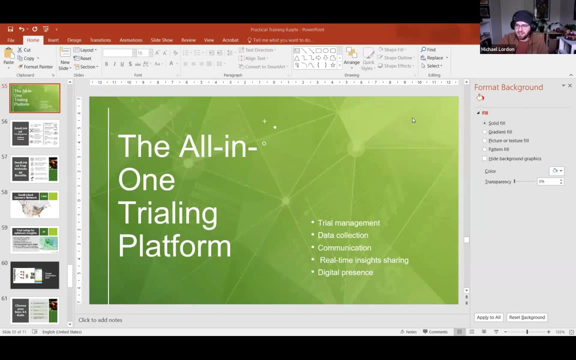 really powerful and it was really cool to see you playing with it real time and how fast everything is. um, we've got a. we've had a few questions that have come in that have been, you know, answered directly to there, but a couple of questions, uh, in the chat for nico: what are the qualifications? 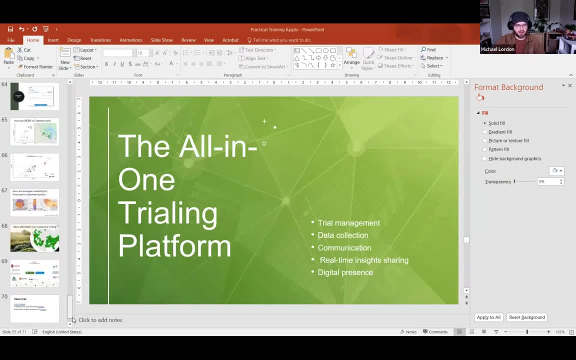 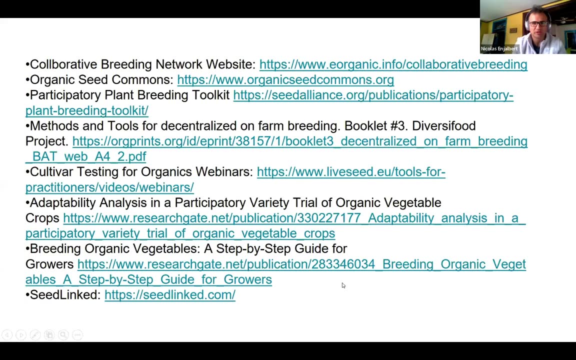 to be a seed link grower. what do you need to do to, uh, to participate in those trials as a grower? yeah, so, um, that's good question. as you run your trialing, you can. you can bring your own growers that you trust if you want to. um, you can also open it to everyone who want to be part of your. 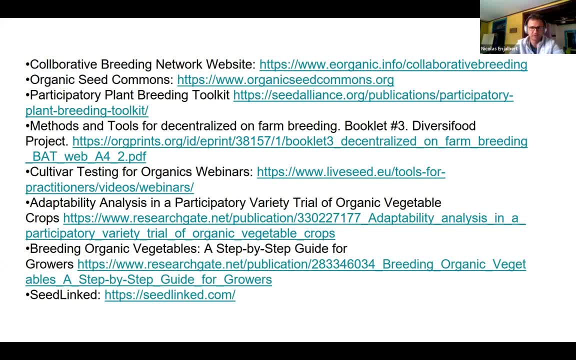 program and even if they have less experience- that's you decide- with within seed links, um, we kind of flag every grower who participates in trial, from beginner to expert and uh, so we know all the growers that typically are returning data and highly engaged and give you good information, uh, but, um, i really encourage. 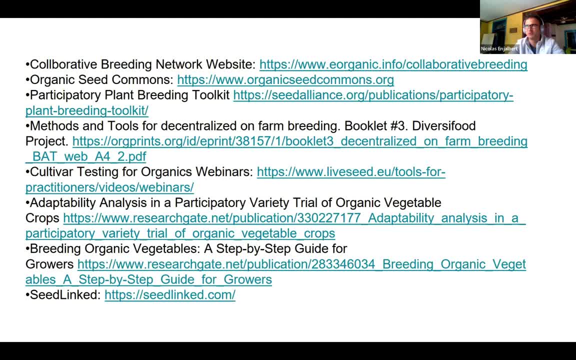 you all to give more trust to all the gardener and grower around you. oftentimes they have way more expertise than you think and the data that they send, especially when it's easy frame is, is just incredibly powerful. a clarifying question from the same person who asked that is like? is the weight of a response? 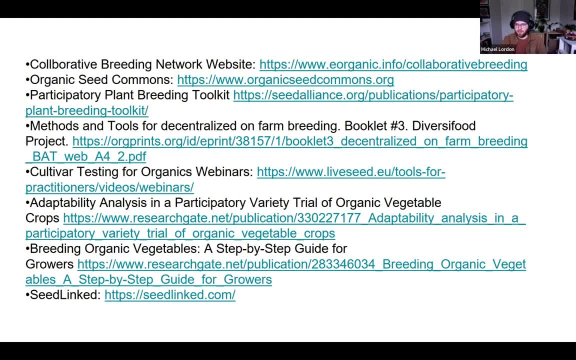 from a grower the same if they're just growing one plant on their balcony or if they're growing a full high tunnel. like, how do you, how do you differentiate the um amount of plants or the the level of participation between different growers? yeah, those are really good question. uh, the power, power of collaborative uh trialing, is that you're not. 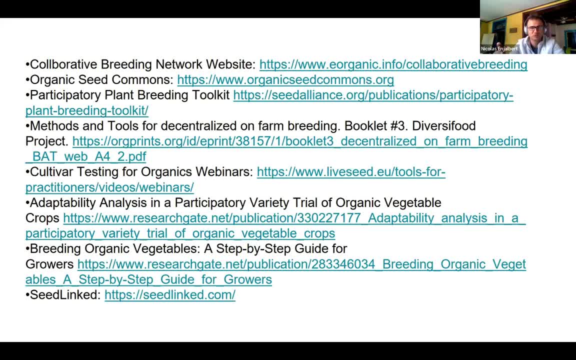 working with three grower, you're working with 10, 15, 20, 100 grower and, via platform, make it easier and what you do is that having more, you have definitely more variability, but then you have a lot of strength in in in the trends and so we, right now, we don't give any weight um in in the 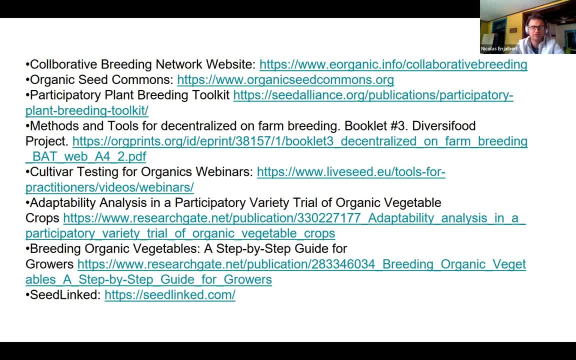 each one. however, we are working with a lot of grower and we're working with a lot of grower, so it's it's a it's a little bit too specific to give a specific weight. and one more question for you, nico: are you the breeder of dark star f1 tomato? 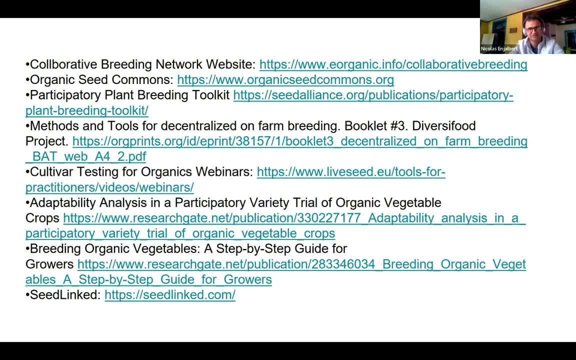 no, no, uh, pan-american asta dark star, and uh, a dark star, and i, i like dark star fool, but what's the difference between dark star or native dark star exactly? um, i think that that's a different question. um, so, the, the, the, the, the. the question is about the different Type I of the grower and the growing, uh, growing. 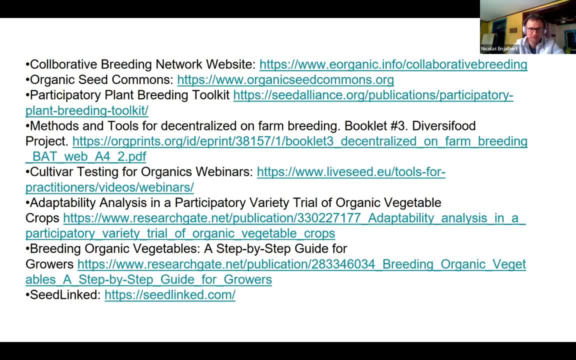 pernilineum, you know in the future. is this a different aspect of the seedling? is it a weird thing, or are you talking about seedling weight or seedling weight? I think Pan-American work with breeders, have their own breeder as well, but I think it's from Pan-American. 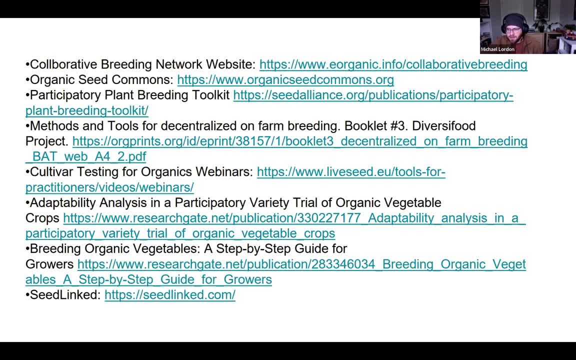 Question for anyone here that wants to respond. They're talking about with corn or with some outcrossing species. there may be a big improvement when using F1 or hybrid plants And they're wondering if tomatoes, for example, mostly self-pollinating crop, if they have the same hybrid potential as corn. 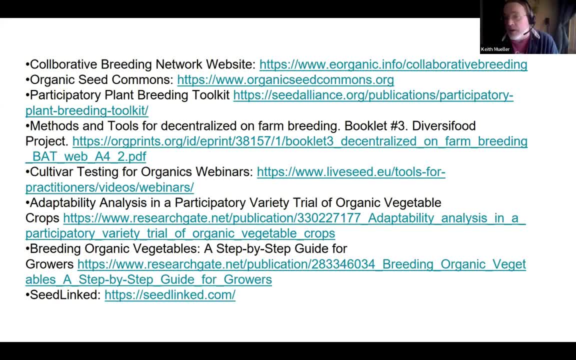 I'll pop in. Depends on the trait you're looking at. But yes, there is a hybrid vigor in various traits for tomatoes. It's very well documented. It just kind of depends on what you're looking at. I can also pop in a bit. 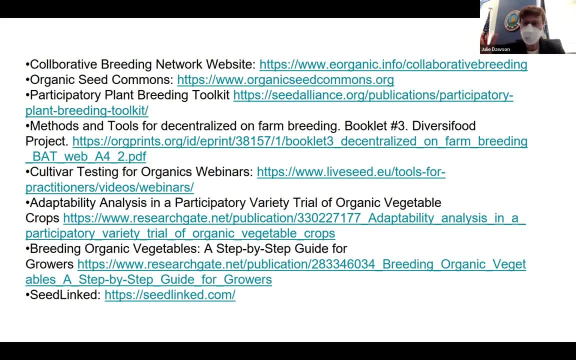 One thing that you can do sometimes more easily with hybrids is combine traits from different parents If you only need A heterozygosity to have an effective trait. So some disease resistances may be effective in the heterozygous state And that might allow you to combine disease resistance with flavor faster. 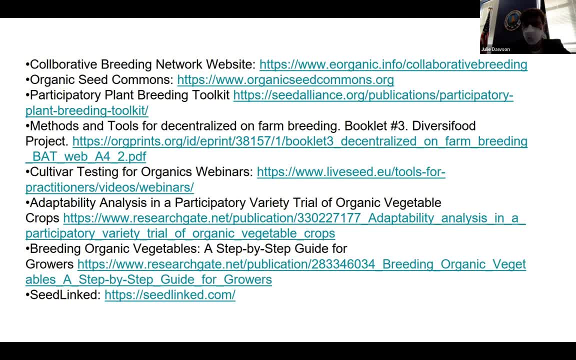 You can also then breed something that's homozygous for disease resistance and flavor, But that hybrid combination may be a faster way to get at some combinations. Thank you, Julie. All right, Okay, I was going to add my sound cut out for part of that. 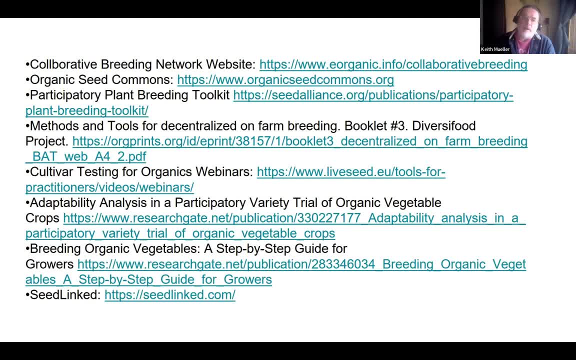 So I'm not sure, But sometimes when you're combining homozygous disease resistance in tomatoes, there's some bad linkage that come with it that affect fruit quality, And so sometimes it's better to have that disease resistance and a heterozygous state than it is in the homozygous state. 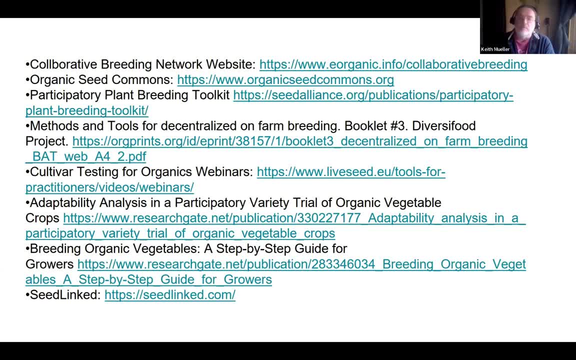 But that's not always the case. That's just an example And that happens with Fusarium wilt, resistance three And I think they broke the linkage. But tomato spotted wilt produced little bumps on the bottom of the fruit, which wasn't marketable. 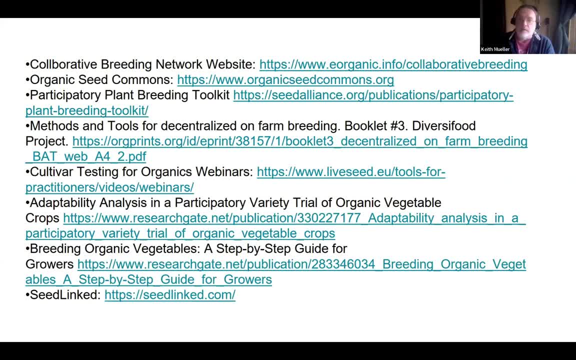 And so they had to break that linkage, which I understand they have now, But that was kind of why that was always put into hybrids. Do you know if pH genes for late blight have bad influence for fruit? That is one of them that, and I can't remember which one offhand that did. 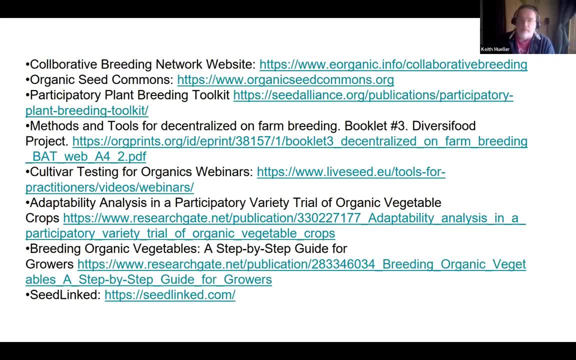 If it's in the homozygous state. it did affect fruit, But I can't specifically recall what it was. I think it was a blossom scar as part of it. But there's something else I don't remember. I we don't have late blight here, so I don't really look at it. 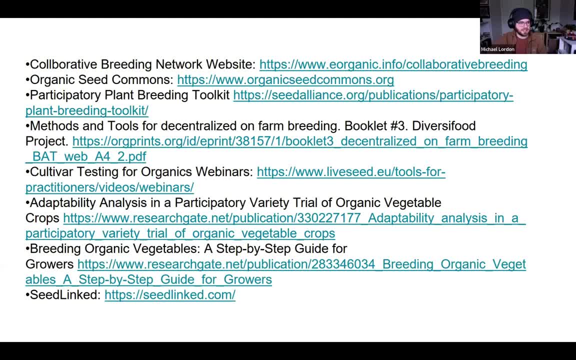 Great. Thank you, Keith. Also wanted To point out the resources that you see here on the screen: A lot of good materials from OSA, as well as from some other organizations that have put out some more advanced resources for data analysis. 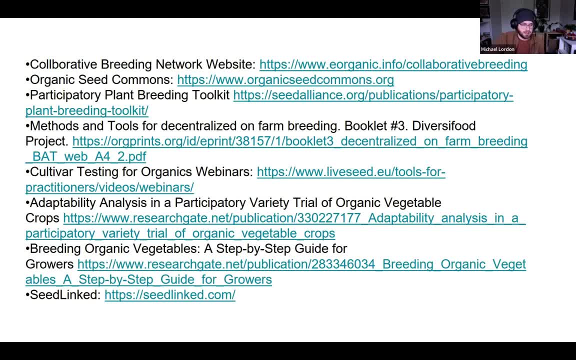 And so you're welcome to check those out. There's also a step by step guide for growers is a book that I have learned a lot from and I really like There's a lot of really clear examples. if you want to go into more of the breeding methods that were mentioned in today, like pedigree- 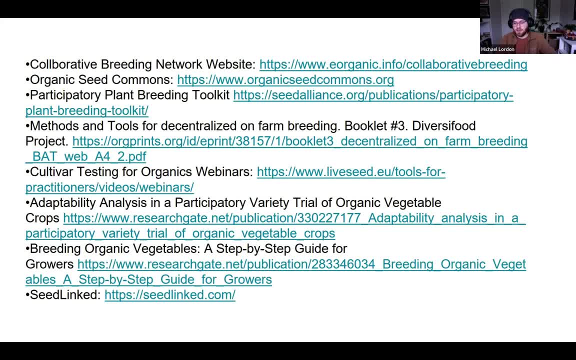 Bulking mass election It's. I found that to be a really digestable and easy to understand resource, So I definitely recommend that to farmers or practitioners. If you have any other questions, feel free to keep putting them in the Q&A or in the chat. 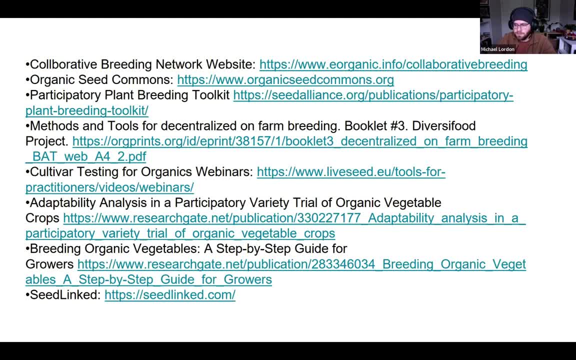 We just have a few minutes left here. Yeah, Go ahead. I have a comment about environment, tracking the environment- I learned this from a good friend over at HydroDRemain- and the laws of protection and preservationPalette. I didn't take it seriously. 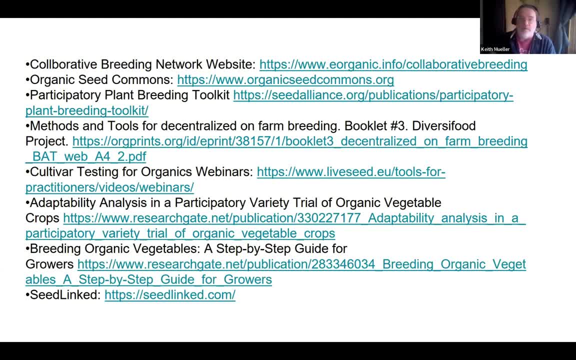 area So you can track fairly well what's going on if you're not there And I can't remember if they put that in a historical. Do you know, Jared, if you can look at that historical build that or not? But it was just. I was really surprised. I didn't know you could do that. 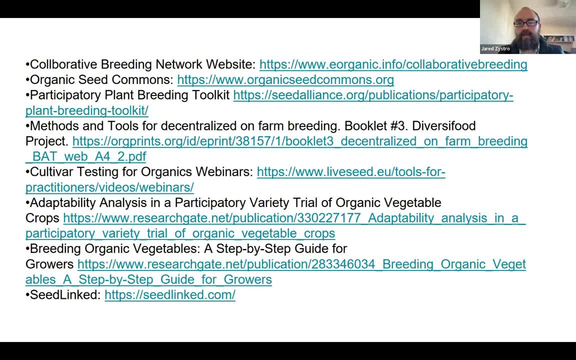 Yeah, I've had a hard time getting the historical data using that method, But the real-time data definitely. There may be a way to get it, get the historical data. Maybe it's a little bit more complicated, I don't know. 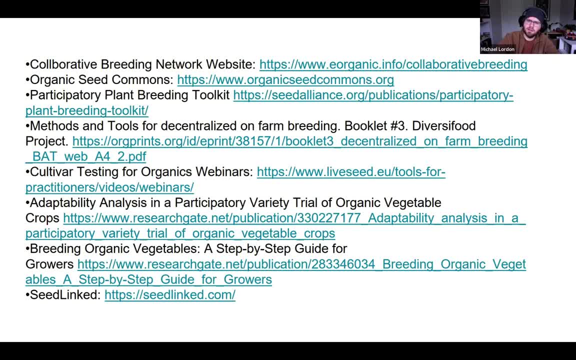 someone else knows, nico. i don't know if that's something that, uh, is one of the capabilities that could be built into seed linked, or if that, if environmental data is available. yeah, that's on the queue for a while and you know, we put it to heart in his own and then we 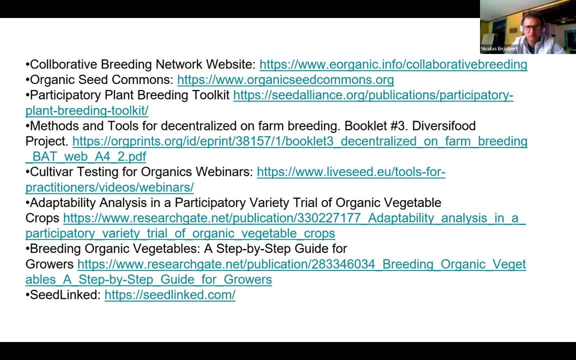 really is uh hoping to find funding to work with uh prism or oregon state uh, where all the climatic lab funnel to integrate um all those information. so it will come for sure uh, it's just a matter of time. but yeah, i'm really excited to yeah add more data, science and information behind seed links. 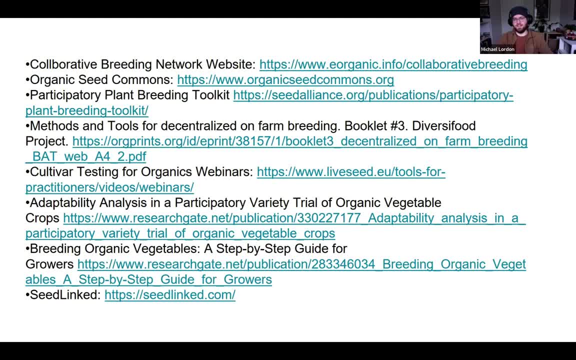 when we have the capacity. so i know you can do that. you can build that with, uh, the weather underground if you have your own station and create your own station, um relying on somebody else's hit or miss, because it goes in and out and if you're out in a field you're going to have to. 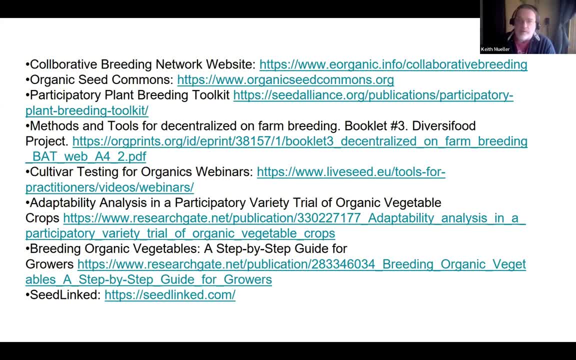 have internet connectivity and all that going on, you know. so it's better if you have a a good internet connection. you can build that easily with the weather underground. but um, you know, i wouldn't be valuable to me because everywhere i go i don't get great cell service. 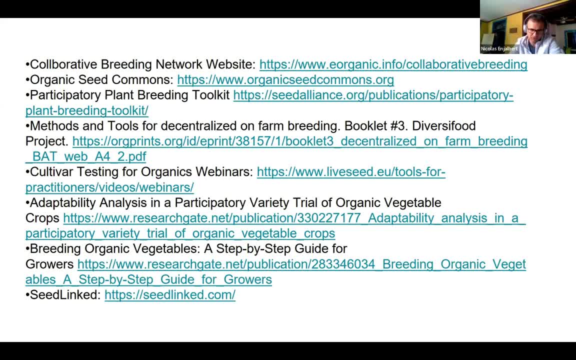 then for seedling, like you have package our package with connected to world claim, and so we are actually right now doing some analysis with um a group, dr vanitin, who is leading collaborative trialing and is analyzing all the data of seedling to see what can we do for gba. so yeah, i hope to be able to. 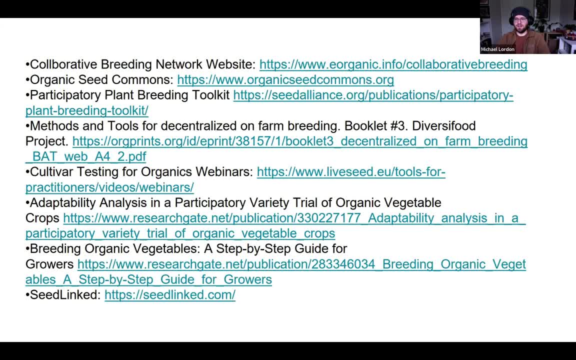 share more soon. great well, i'm not seeing any more any more questions that have not been answered so far, so i think we'll wrap it up. i want to thank everybody again for for watching and for all your great questions. uh, this is not the end of our project. i. 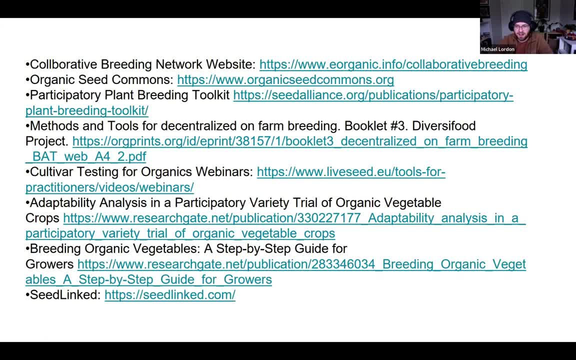 just want to say thank you so much to andrew and chris for sharing all this information and just uh for the worried about uh andrew in being sick. so much to know watching uh gba talk and um, we'll see all of that soon. next week we're going to be uh working on a new project. 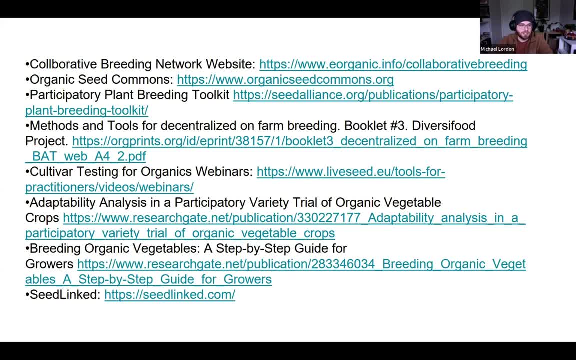 project that's going to be called the plant breeding project. so throughout this year, we're going to be, uh, compiling all of these webinars, along with all of the resources that we've been posting, and even more resources, short instructional videos and a few supplements. that'll all be posted. 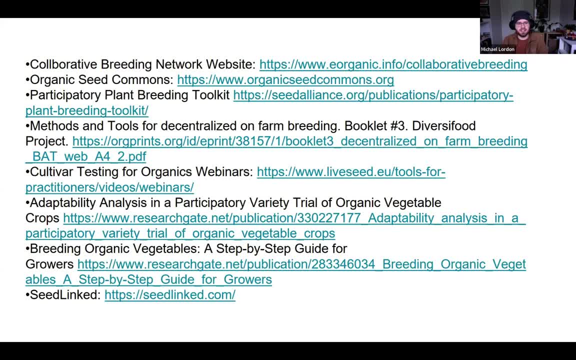 everybody who's interested in seed growing, seed policy, seed commercialization, plant breeding. It's a great network of people that you can interact with, ask questions, share updates. If any of the other team members here have any final thoughts, I'd welcome that. 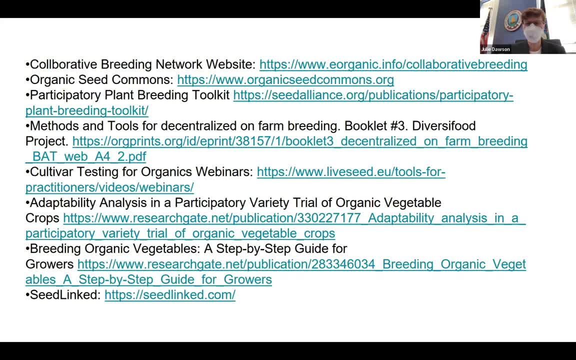 Thanks everyone for joining us and participating, and we welcome continued interaction afterwards, So don't hesitate to reach out. Yeah, thanks everyone for joining. Yeah, and get on there and join a variety trial on SeedLinked, if you haven't already, or the Seed to Kitchen Collaborative. 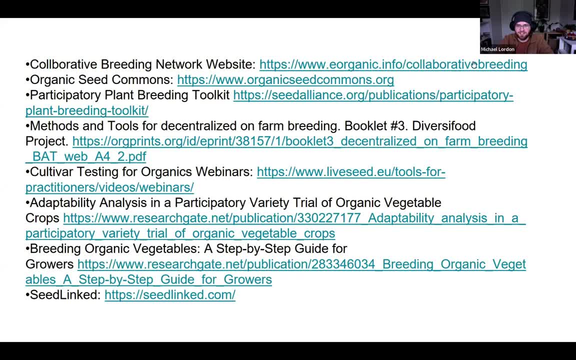 is hosting some more variety trials this year. So let's get involved, let's keep working together. 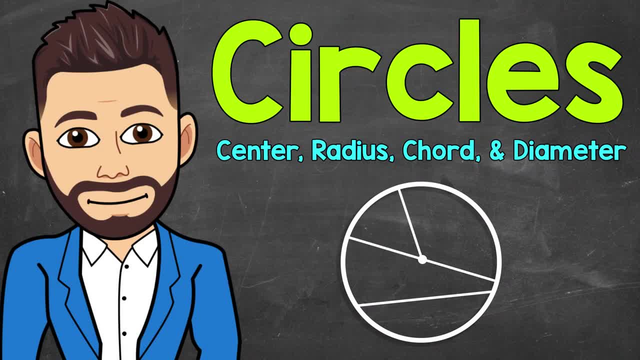 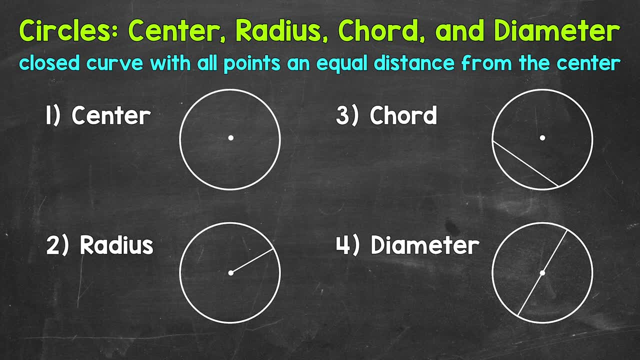 Welcome to Math with Mr J. In this video I'm going to cover four very important parts of a circle: The center, radius, chord and diameter. Now remember, a circle is a closed curve with all points an equal distance from the center, And circles are plain figures, meaning they're.